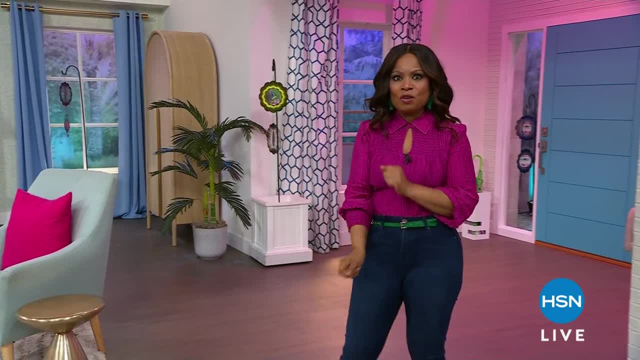 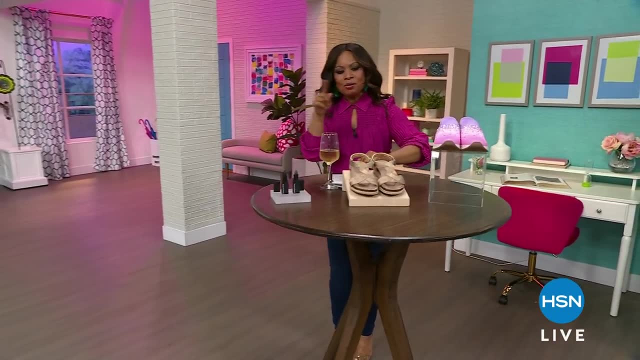 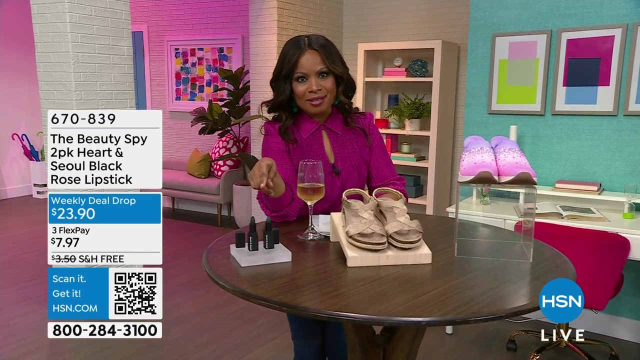 to be doing a little lawn and gardening. We've got beauty spy in the show tonight. We've got Kenneth Cole-Schulz. Come along with me. I'll give you a little bit of a sneak peek. Where do you want to start? Shoes, a little wine. Why don't we start with heart and soul? Have you guys seen? 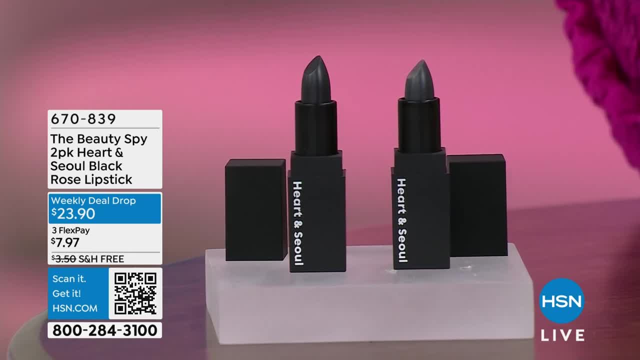 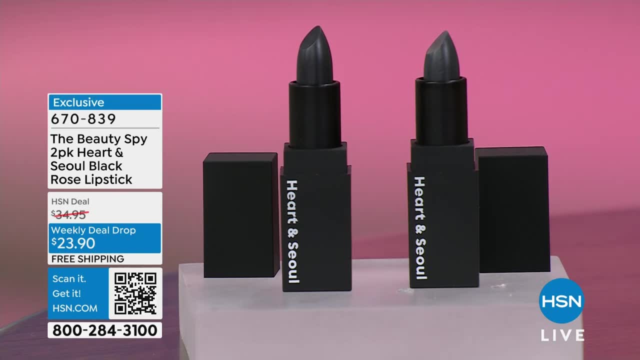 this. So this comes from a rare black rose oil that looks dark but works with the chemistry and pH balance in your skin that will give you the perfect, most beautiful berry color to your lips. It's super hydrating, super moisturizing, and we're going to give you a buy one, get one. It's. 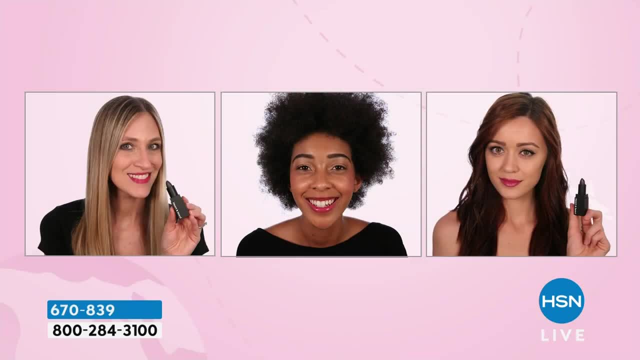 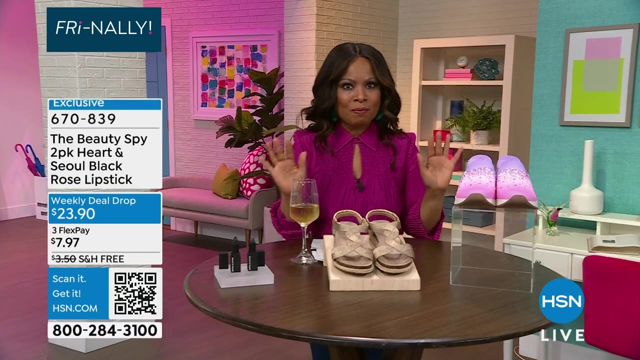 a two-pack of our heart and soul famous lip color. and it works on every skin tone because the lip color will customize to your own chemistry and your own pH balance. We have Chelsea Scott in the house, our beauty spy. She's going to be here live for the very first time. I'm super excited. 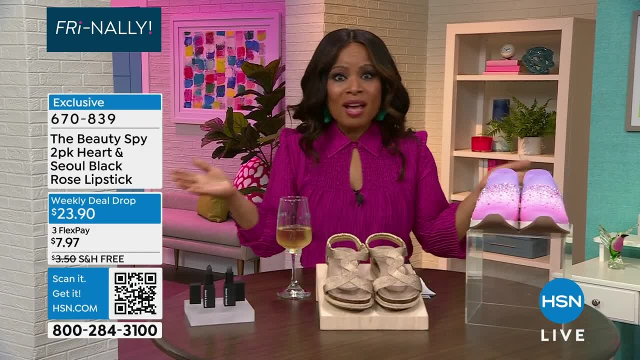 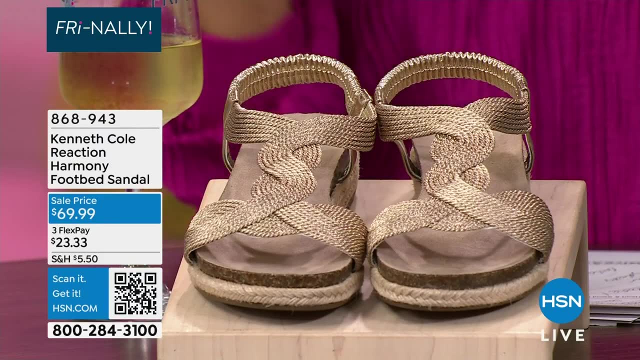 about this Sells out every single time. I would call ahead. And we love our shoes, don't we? So we couldn't make up our mind. Are we ready for sandal season or we want a little sneakers? So we're. 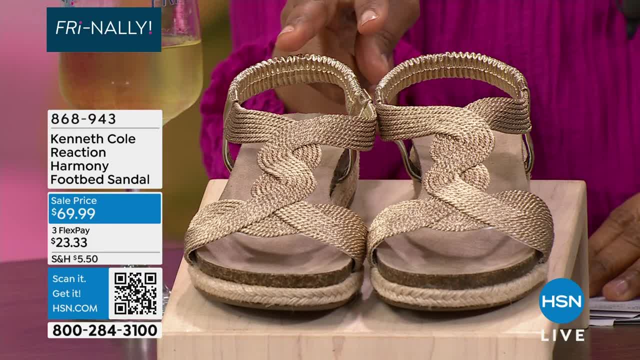 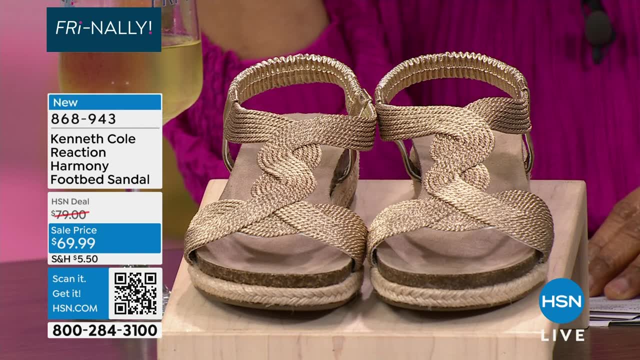 going to give you a look at both. Let's start with the sandals from Kenneth Cole Reaction. This is called the Harmony Footbed Sandal. You're looking at it in the soft gold. We have a pewter. We also have it in a black. It's brand new. It's on Flex Pay. It's gorgeous, Ready for a sandal season. 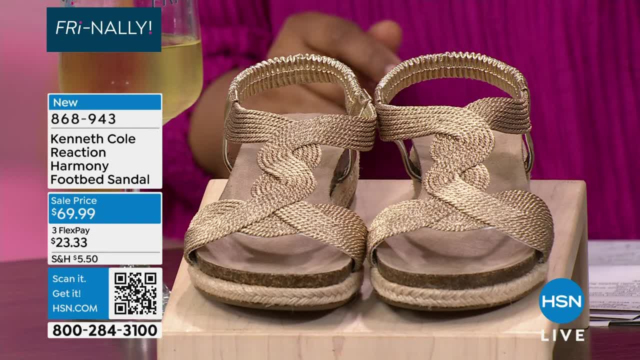 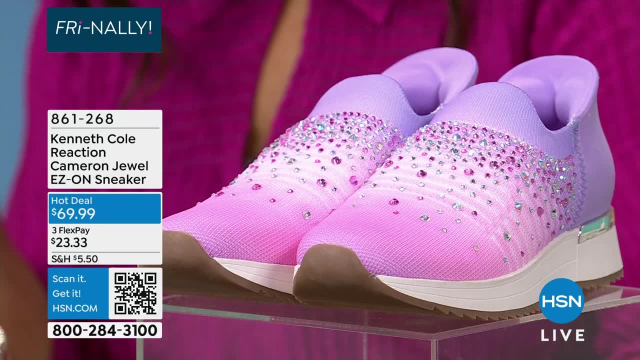 sizes 5 through 11.. Then, of course, we've got the sneakers. This is one of my favorite choices. It's called Unicorn, But we have other colors as well. Look at all of the jewels on this one. It's a slip-on, jogger style sneaker, which is very popular. 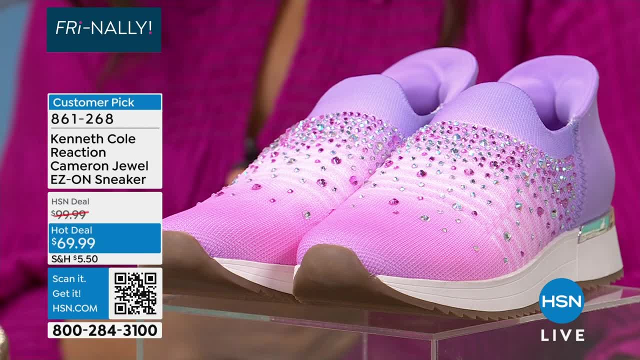 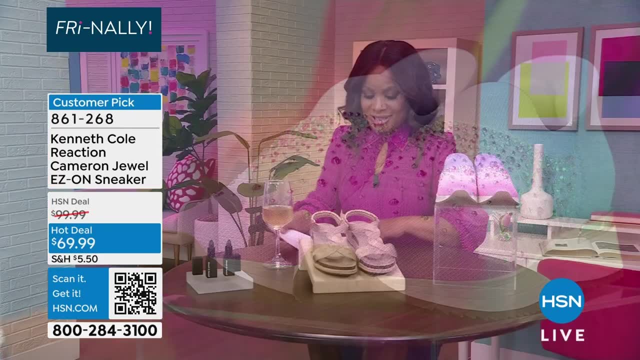 This choice is Unicorn. We've got a navy, We've got a black, We've got a cream And we also have a lime. So big show this hour, But we want you to get social with us And we certainly hope that. 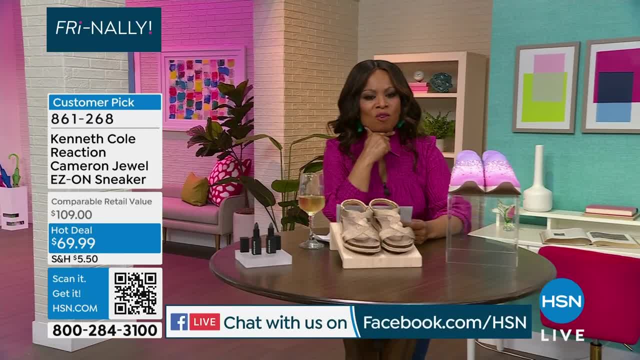 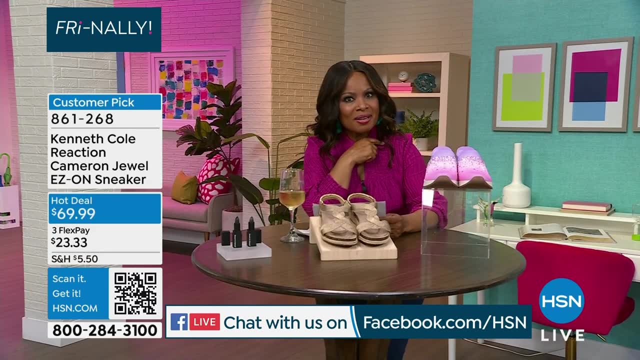 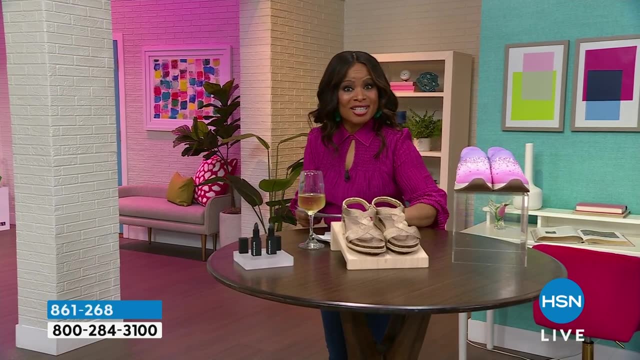 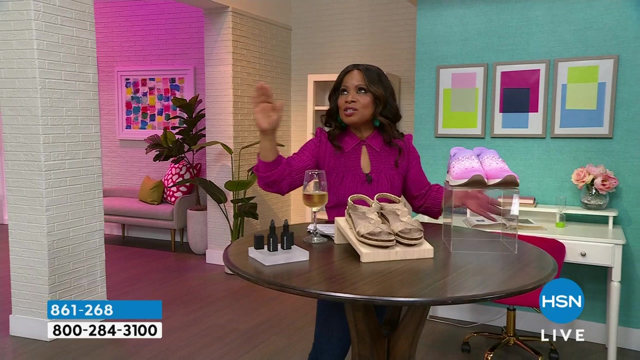 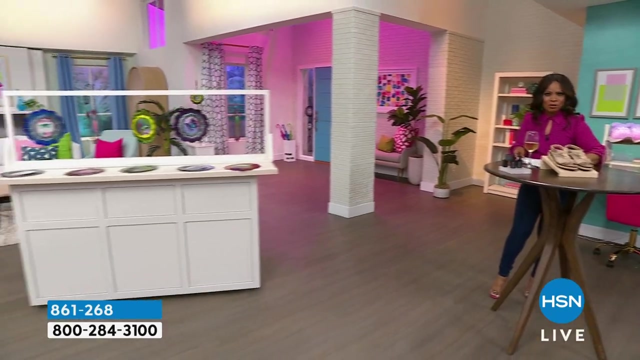 you will. So we kind of gathered around and thought about: hmm, for the springtime, what are we going to do with for spring? Well, get social with us. Let us know, Use hashtag giveaway and one of you will be selected to win a $25 gift card. Have you had a chance to see our today's special? Well, it's perfect for spring and it's perfect year-round. It's exclusive to us at HSN. We've taken it to a whole new level. As a matter of fact, you get a two-pack. We're going to give you our wind and weather today's special, something we've never done before. Let's go. 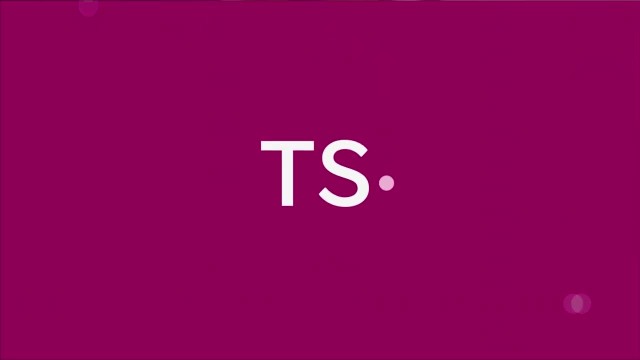 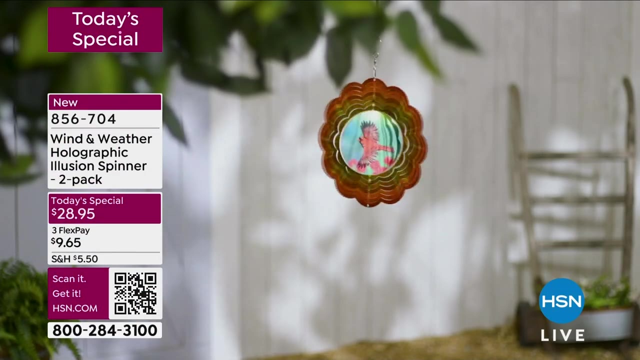 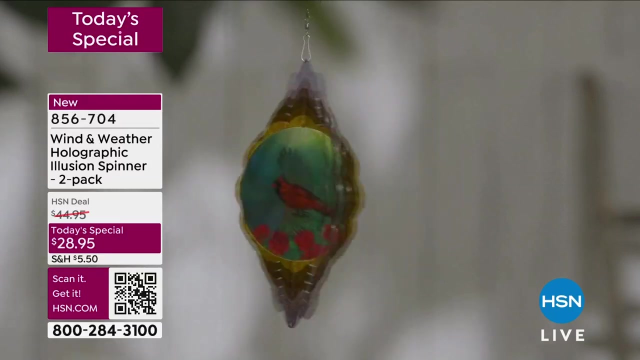 So as you look at this, look at how gorgeous these are- It looks like you're taking flight. whether you're choosing a butterfly or a hummingbird, or a rose or a cardinal, The hummingbird, by the way, is going to be the most limited. We only have about 700 remaining. 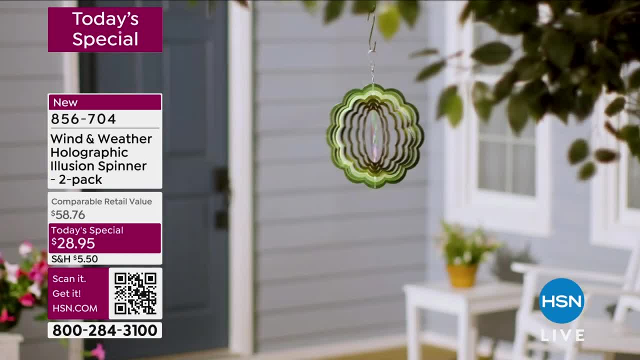 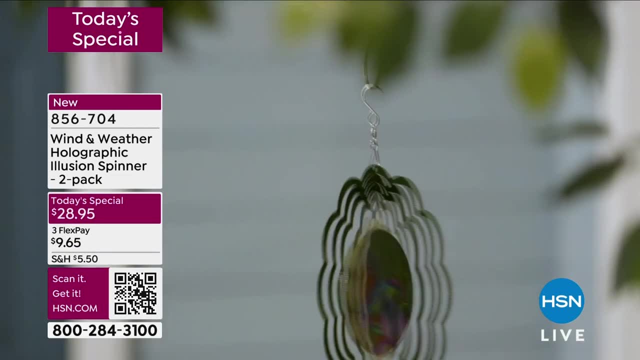 You're looking at the two-pack of our wind and weather holographic spinners. You've seen us bring them to you before. You're going to get a two-pack of our wind and weather holographic spinners, But never before quite like this. Here's what you need to know. You're going to hang these. 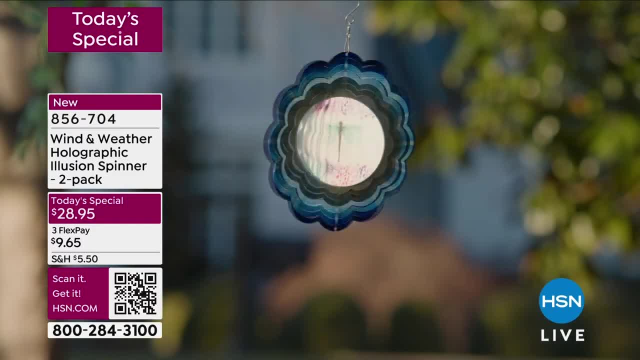 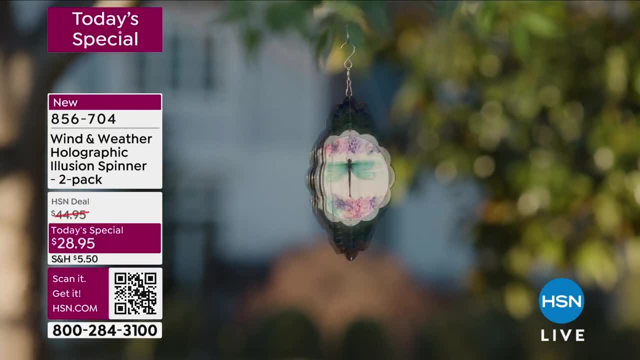 easily. They're about 10 inches, so the size of a dinner plate. virtually They're simple, but when the wind spins these around, you can see how the movement, the illusion of the movement, just comes alive. These are incredible. We're the only place that you can find them. We've got the. 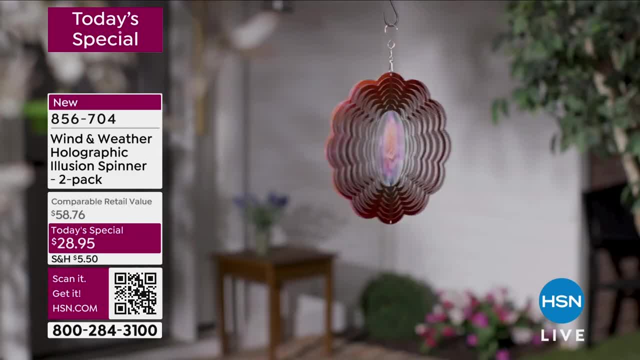 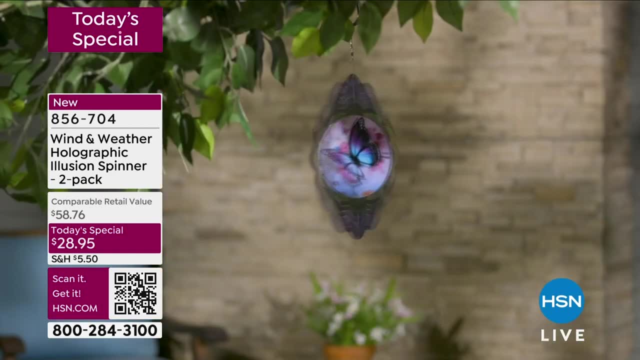 lowest price that you can find, and this is going to be the next to the final chance for the entire day for you to be able to pick them up. Let us know if you'd like to have the butterfly, the rose, the dragonfly, the cardinal or that very 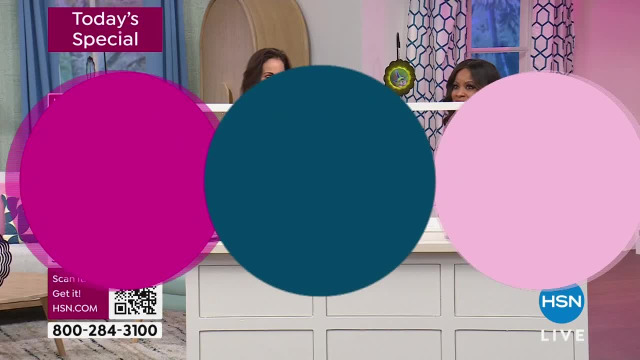 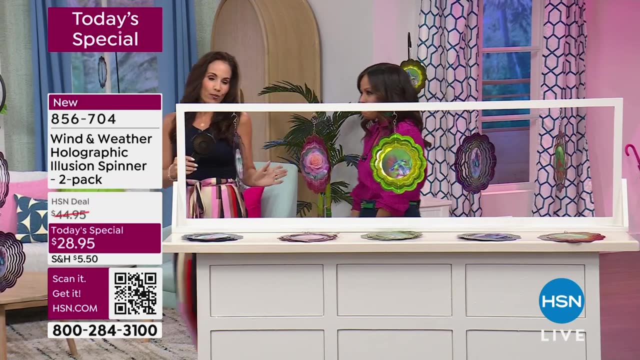 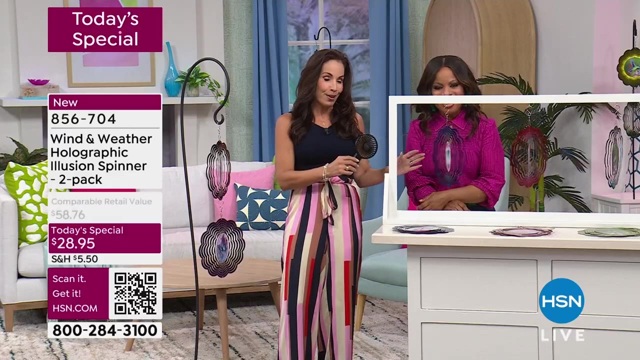 limited hummingbird. Joining me is my good friend, Yvette Lopez, who not only happens to be one of our home and garden experts, but we love these so much. I have had so much fun today and I brought a little hand fan out here because we're inside so obviously there's no breeze. but, as you can see, 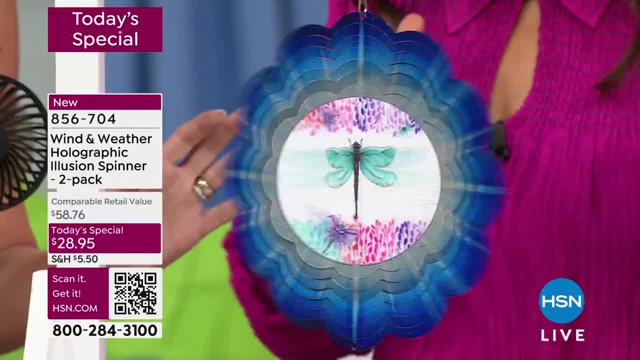 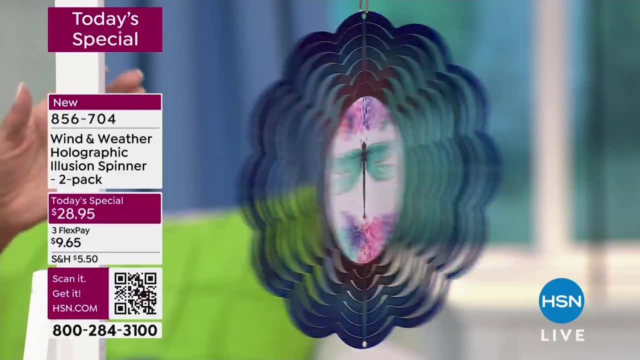 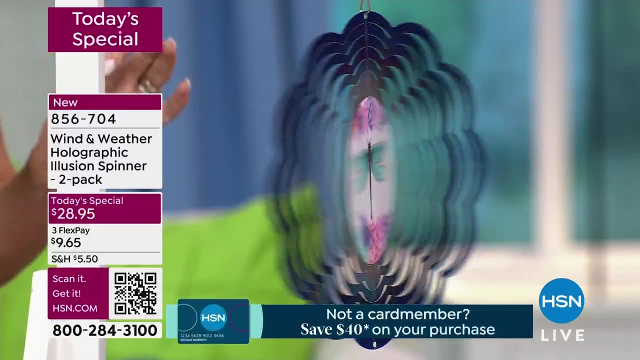 just this light hand fan. Wow, Look at the wings of that dragon. Look at that. In fact, I'll go back a little bit because that one's taken off there, but what I want you to take note on there, look at that holographic design. So this is brand new to wind and weather. 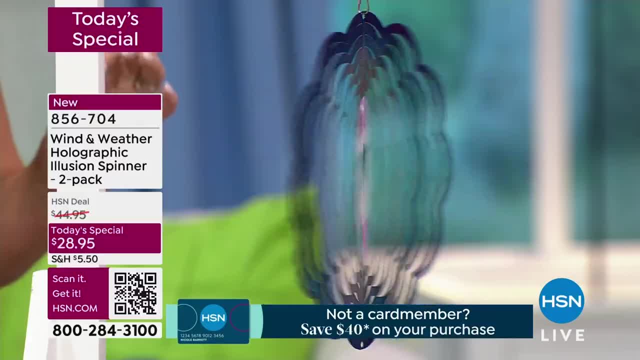 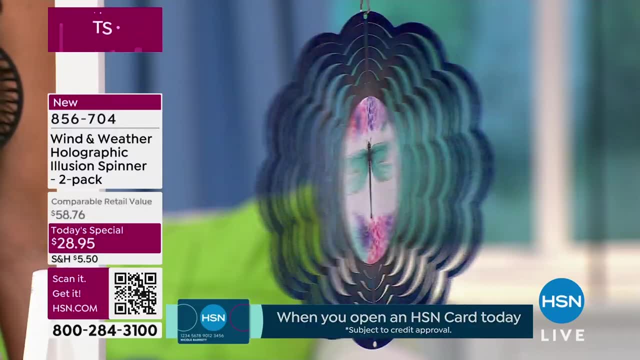 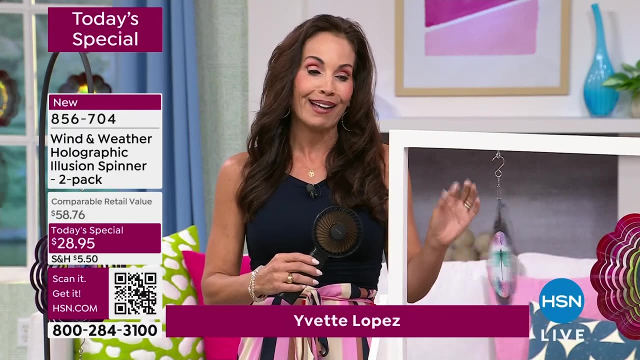 right, It's also brand new to HSN and it is exclusive. So for our five-year anniversary that we are celebrating today, we wanted to bring our HSN customers something exclusive, something new, and that's That's what we've done, and not just one, but two. You get two of them, As you'll see, the butterfly. 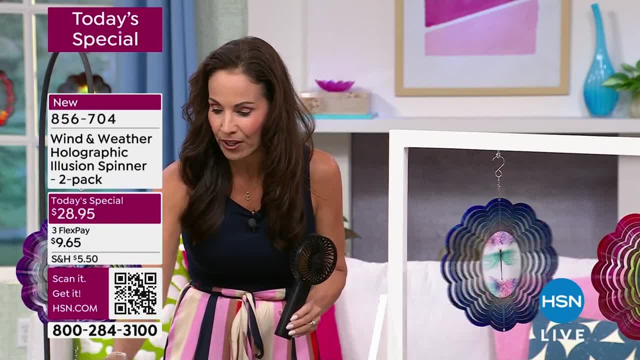 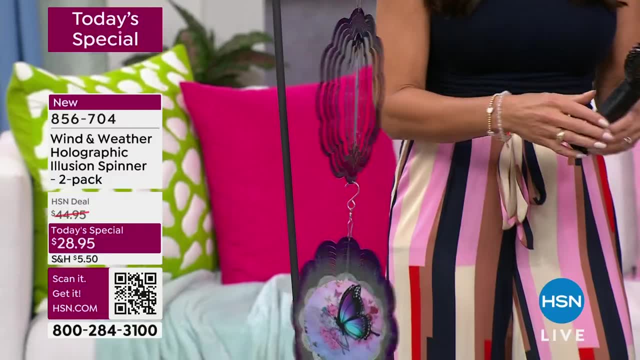 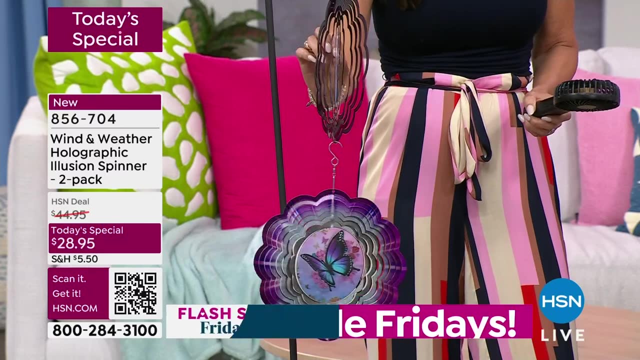 hanging here. they also can piggyback off of one another so you can hang them in a nice vertical space. And you know, Marlo, the reason why we did the two-pack is because we actually sold these last year, the same type, but not the holograph, not the hologram in the middle, And they sold each. 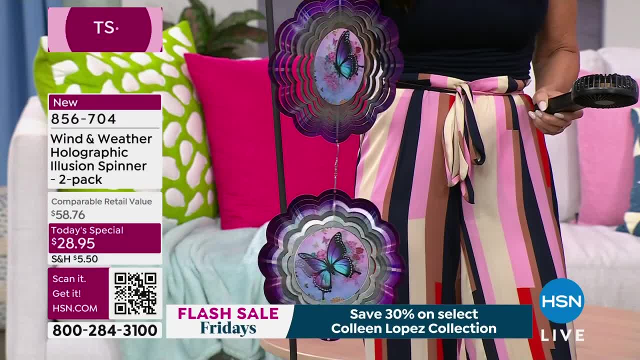 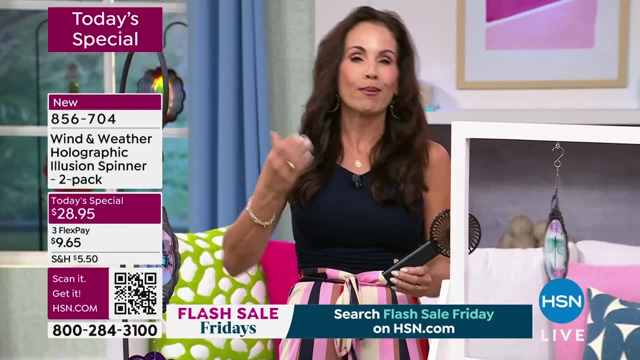 for like 18 and some change and they sold out. And when we read about it we were like, oh, that's so cool. And when we read the reviews the customers just said, oh, I got one home. I loved it so much. I got one for my mother or my sister or my best friend. So we figured: 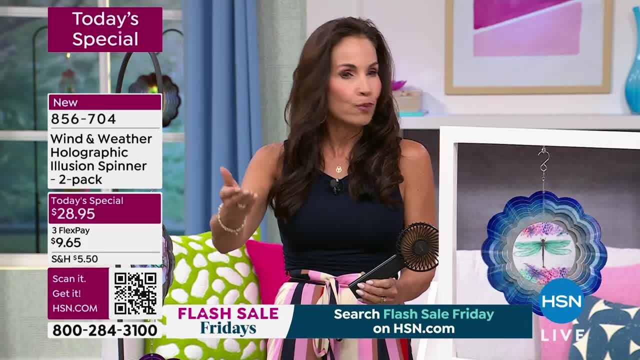 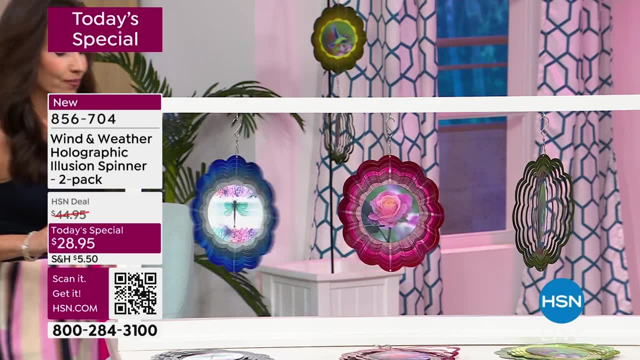 you know what, If you're buying multiples anyway, let's do a two-pack and give you a better value. I think what we're going to do is we're going to invite you to shop, We're going to show you, take you down to show you each and every one of them separately. I think you have a. 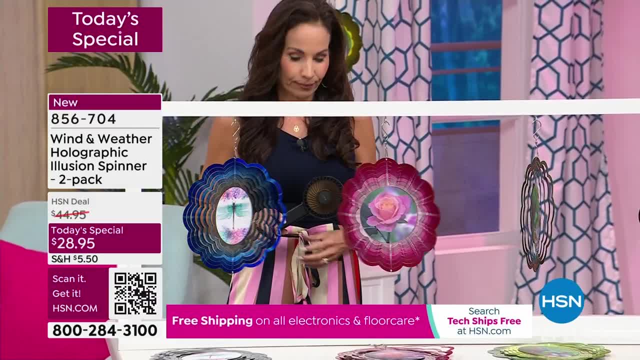 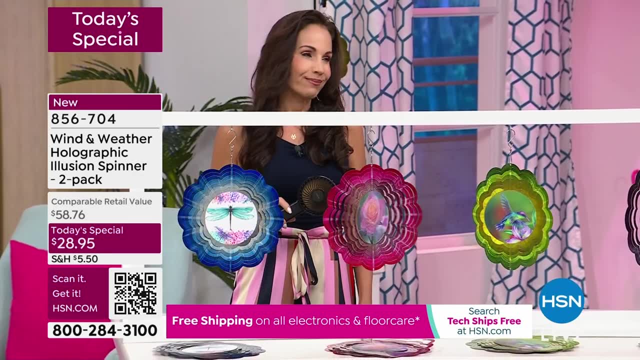 good idea of the dragonfly. Remember every one that you see. remember you're getting it times two, It is exclusive, It is the lowest price And this will be your final chance, this hour and next hour, your final presentation, to be able to grab it. Let's go to the rose. 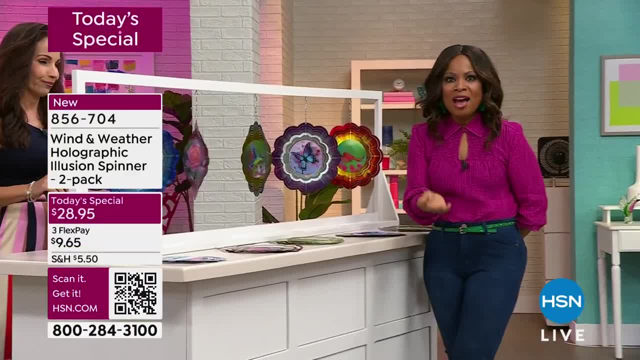 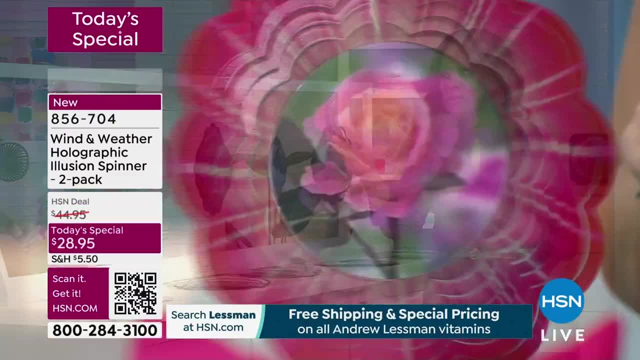 because Mother's Day is a month away, but maybe you're an avid gardener or rose means something very special to you and sentimental to you. I want you to get a closeup of the rose and it really just allows you to be able to see. Let me slow it down. Let me slow it down a little bit. 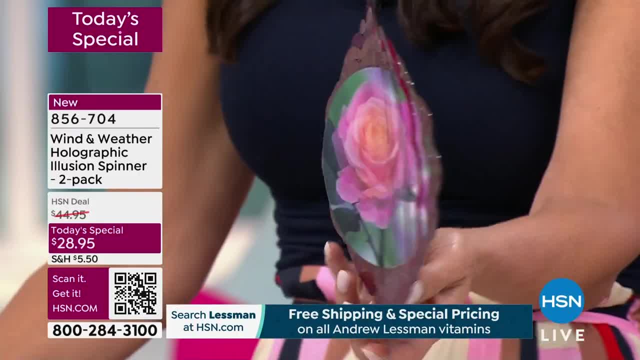 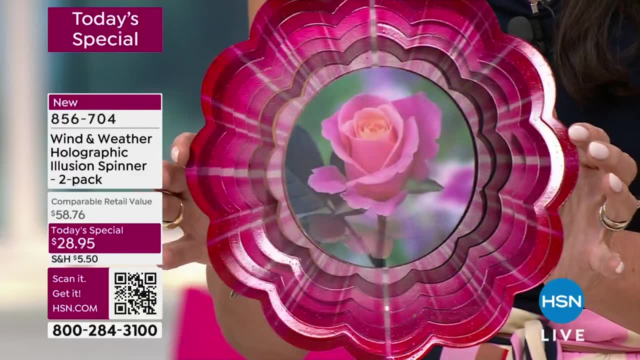 Slow it down so you can see. In fact, you know what. I'm going to stop it because I want you to see that all I do is shift it from side to side and the rose blooms. I was going to say that Look carefully, Look at your eyes So you look. 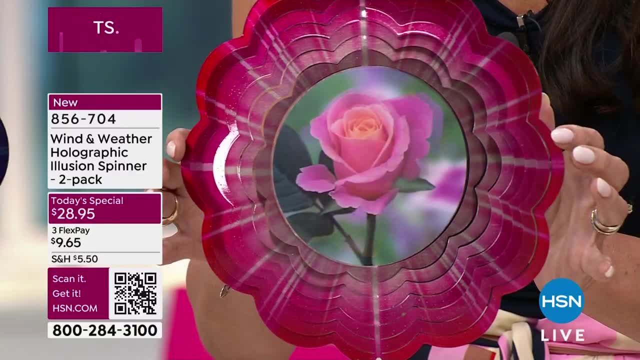 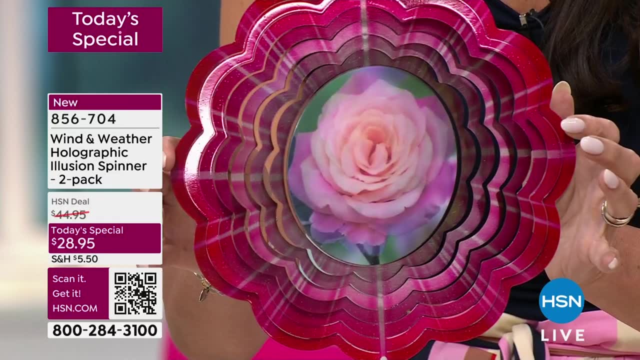 at. look at that Now. look at what happens. I know it's so magical and incredible- And look at the vivid colors. So you can't find anything quite like this out in the market. That's what makes these so exclusive. The size: they're about 10 inches in size. We're giving you two. 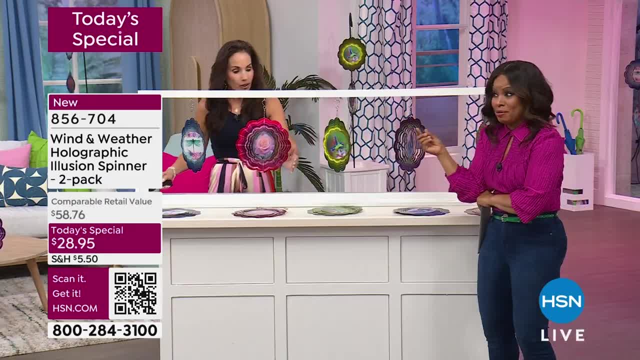 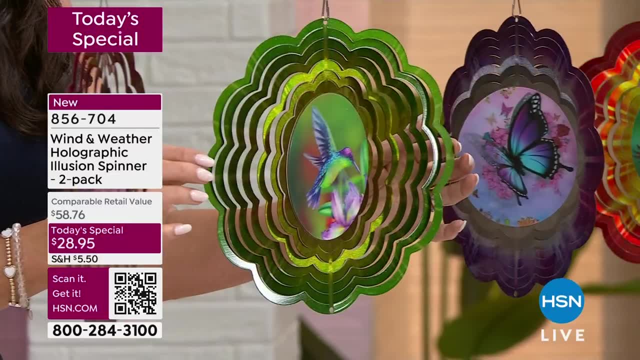 the roses. I mean, they're all beautiful, It's stunning. Okay, Let's show you the next one, because I'm telling you they get prettier as we go. You get the hook as well. Remember, you're getting two and you might want to pick it according to the color or your favorite little winged. 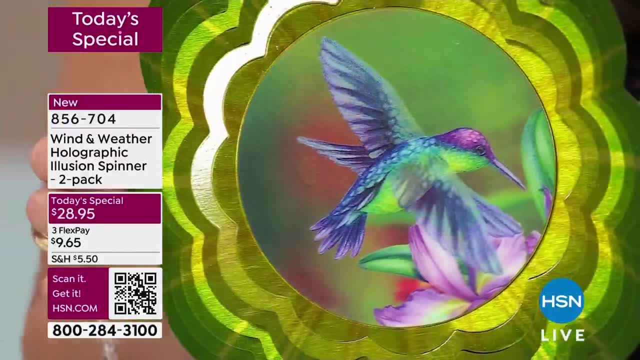 friend here. Here's a hummingbird, I know That's the one. only a few hundred, fewer than 700 remain. If you want the hummingbird, I apologize. Oh no, no, you're fine If you want the hummingbird. 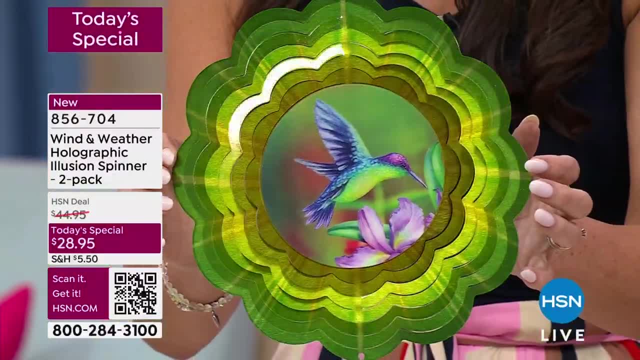 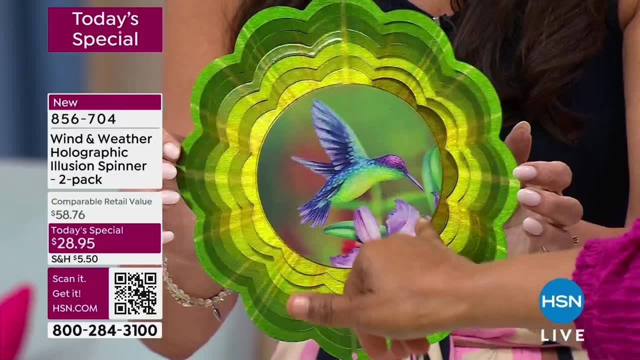 you do need to call. Take a really close look at the hummingbird and you can see- and it's the only one that's in this beautiful green. but look at the colors of the hummingbird and look at the hummingbird kind of coming down. It looks like it's flying but it looks like it has a little. 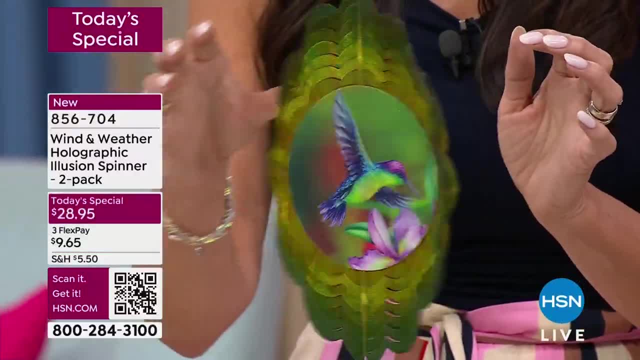 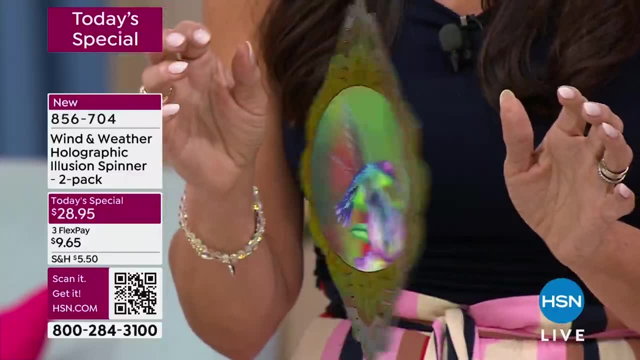 bit of a. I'll tell you what. when I spin it, you can see it in flight. Look at the movement of the wings there. There it goes. It just brings the design to life. It just really does. I don't. 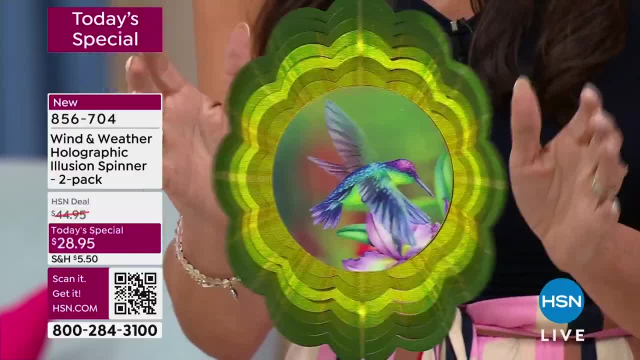 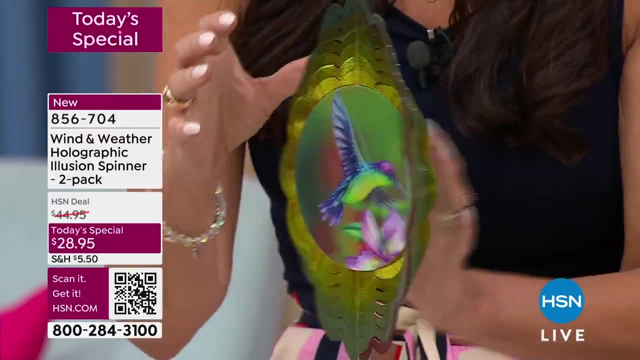 know how it does it, but I don't even care, I just love watching it. It's just that hologram. but I also want you to pay attention to the paint, the colors here, because when you notice it, doesn't it look like light is emitting from it? Yes, Yes, absolutely, It looks like light, and 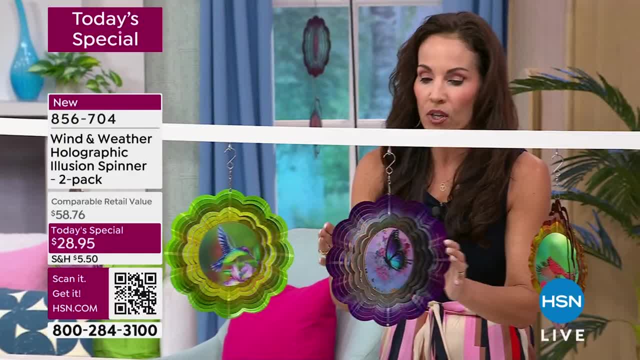 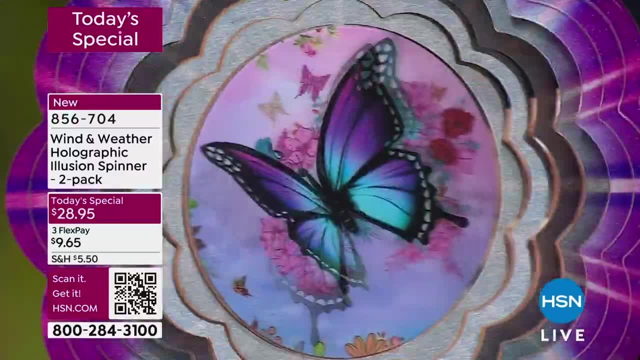 that's part of the illusion. Now, this is a metallic paint and I'm going to move on to the butterfly here, so you can get a chance to see all of them. Here we have the purples and we have the blues. Look at that. Look, the butterfly is just fluttering away. Here you have some silvers in. 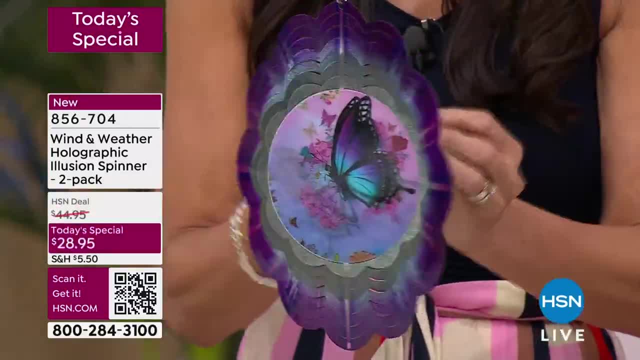 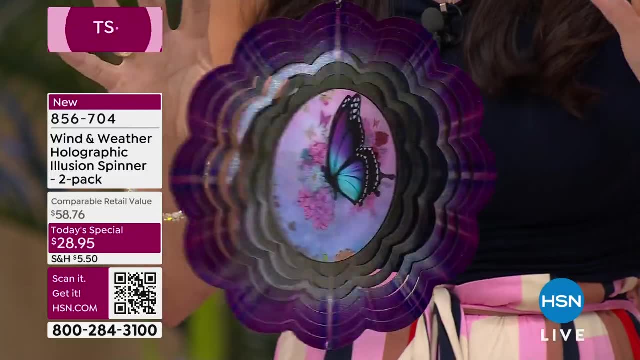 the middle and then the purples. but the way it's painted, in an ombre style, light to dark- this is very intentional and this is what causes that effect. It's like a starburst effect, like it's light, and that's why it's called an illusion. 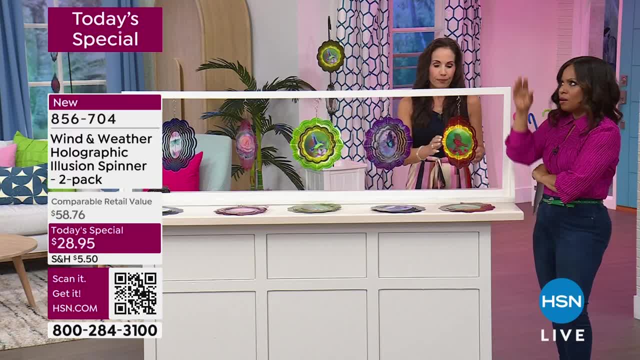 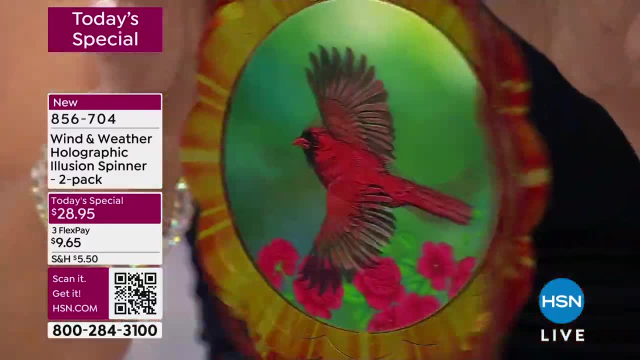 spinner. These would be great, even if you live in a condo or an apartment. you know, maybe you just have like that little bit of a covered area. You don't forget, this is a two pack that you're getting today. It's one day only. I know on the day we sold more than 19,000 last year. we actually 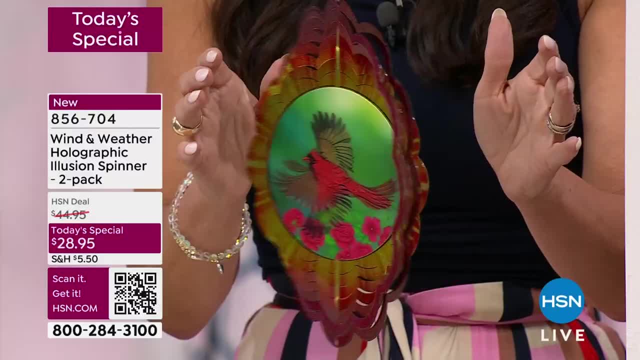 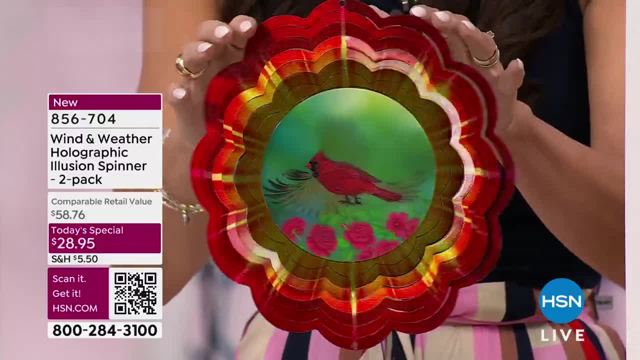 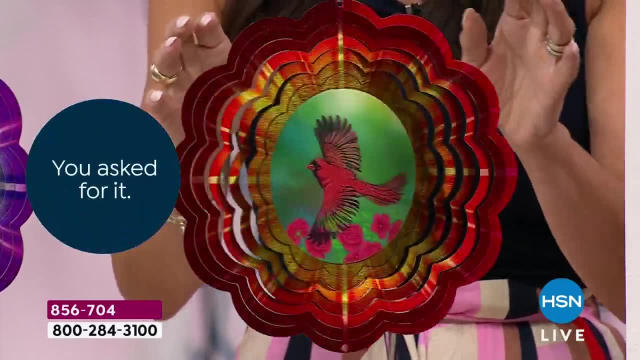 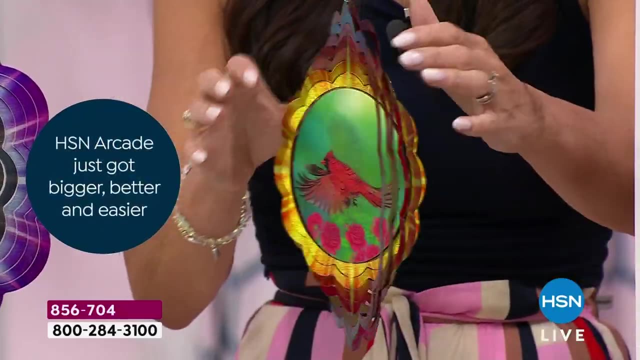 of course, all of this holographic movement, this movement that just is so incredible, as if the cardinal is in flight. Look at the wings, Look at how those wings just appeared to kind of go back and forth with this one And you have an opportunity, even when it's standing still. the 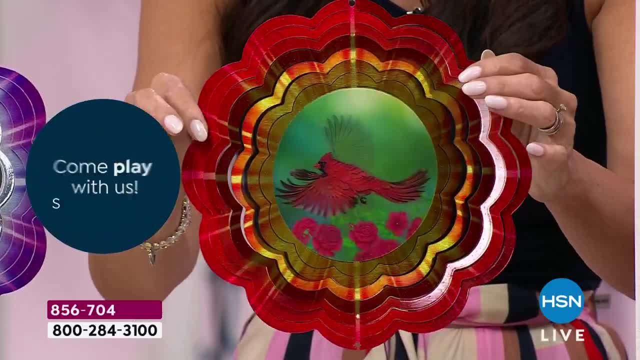 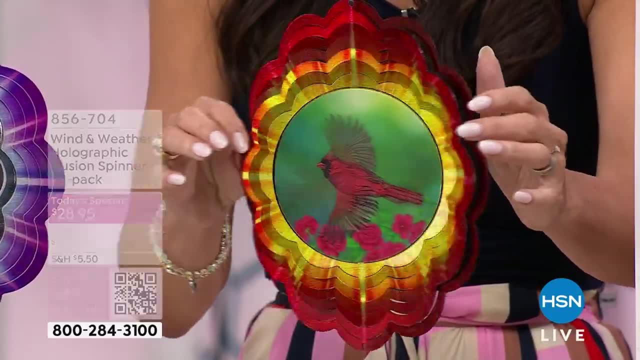 colors are so vivid and so beautiful as the sunlight hits this Gorgeous, The slightest little movement is going to be eye-catching. You're exactly right. And when these, when these are hung outside, I want to make sure that everybody understands, because they're. 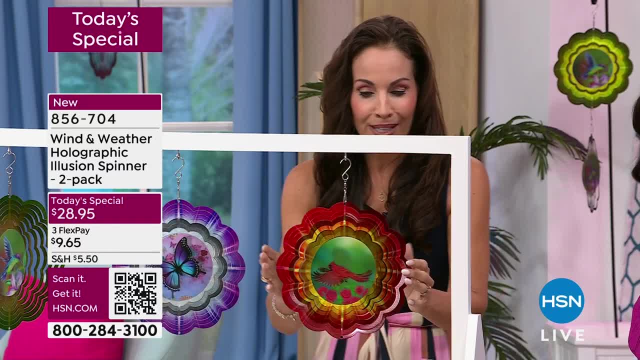 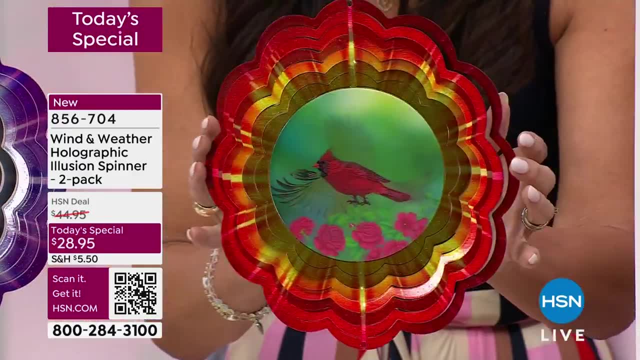 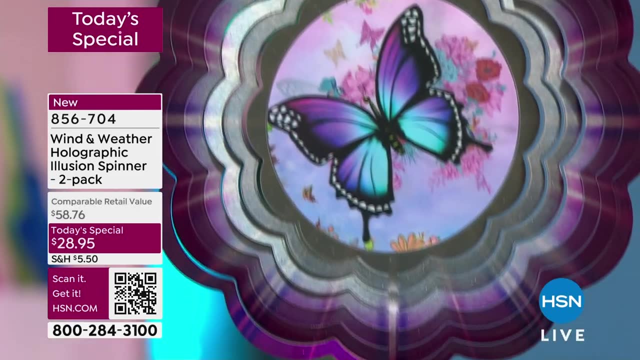 from wind and weather. these are made for the outdoor elements. So all these beautiful colors that you're seeing, this is powder coated. It's durably painted. What that means is, when it rains, when the sun shines down all day long, even when it snows, these are not going to rust, or? 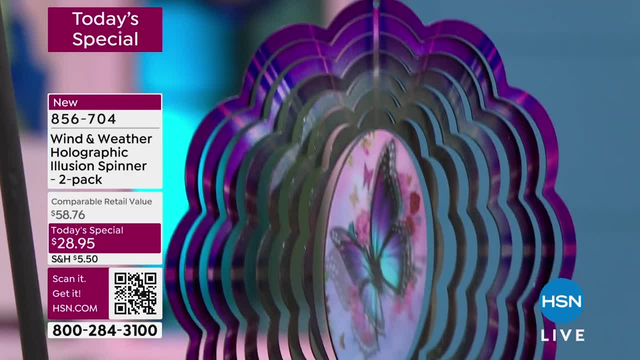 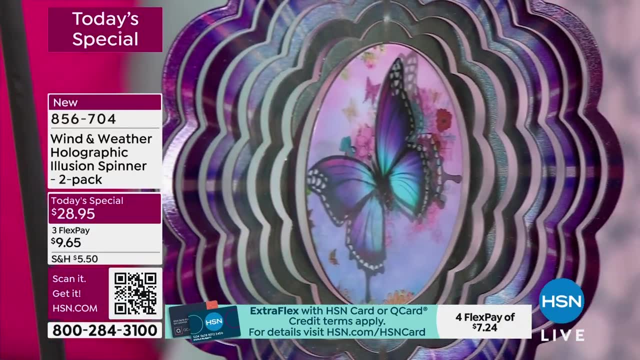 chip or fade Marto. they're going to stay this beautiful and this bright, season after season and year after year, And that's something that wind and weather really does pride itself in, along with wanting to bring you very distinct, unique pieces. It's the quality and the durability. 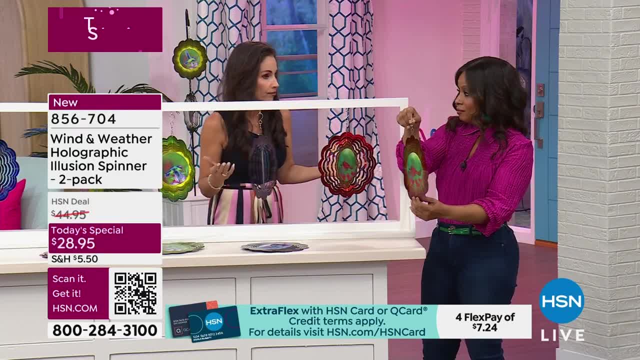 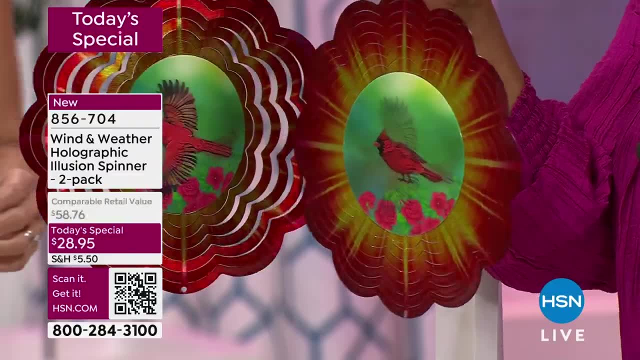 And when you talk about decor outside, that's important. No, no doubt about it, And I'm so happy that you talked about this being powdered coated steel. A lot of us know that from the origami products that we present, And we know that those 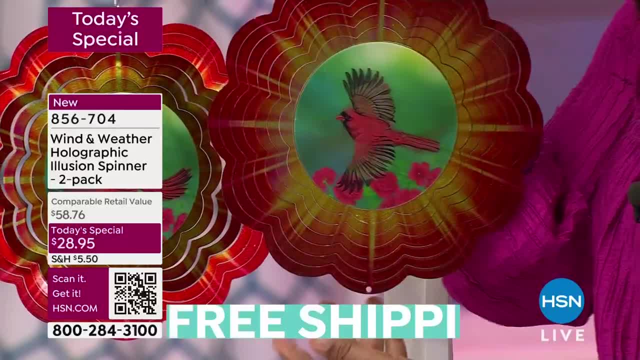 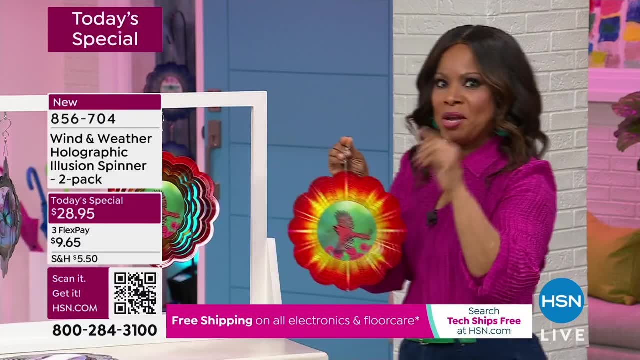 Those are going to be perfect because they don't rust right And you can see the size that. these are about the size of a dinner plate. So anybody that's driving by, believe me, they're probably going to slow down when they're in front of your home, because they are. 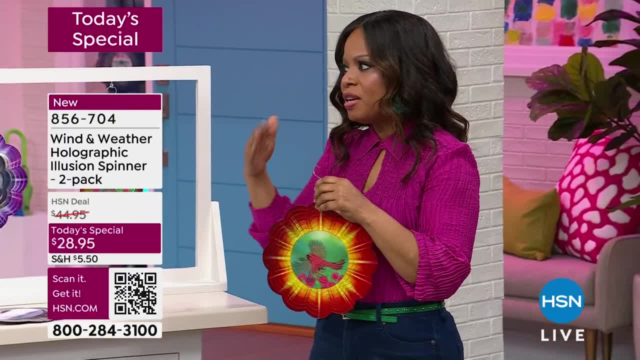 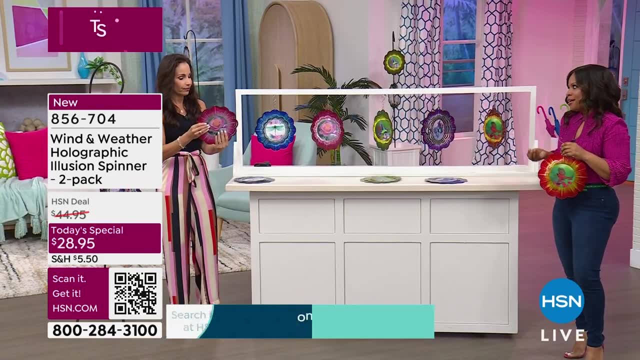 The colors, as you can see, are very bright. They're really vivid. You have a lot of different colors layered in to each one of them. They're individual works of art. The hardest part is deciding which one is going to be your favorite. We mentioned to you early on that we're going to 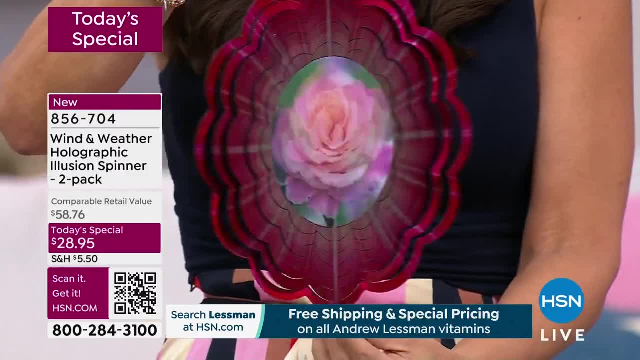 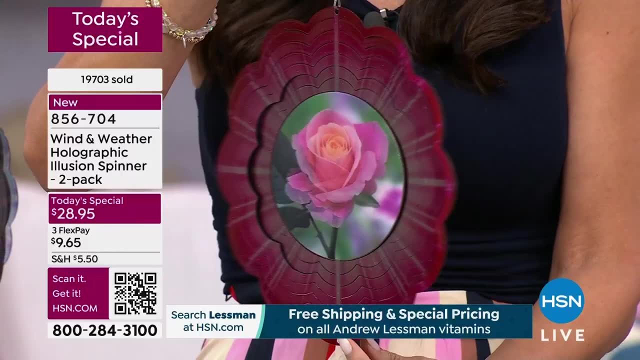 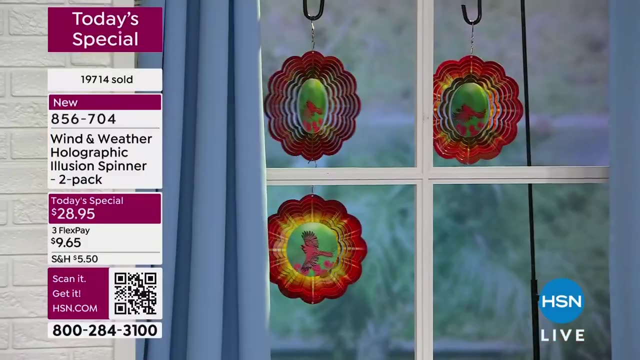 have a rose garden And we know that Mother's Day is exactly a month away from today. I look at that rose and how perfect. Or maybe your name is Rose right. Or maybe you just love roses and you have a rose garden. So you decide this is going to be the next to the final presentation. 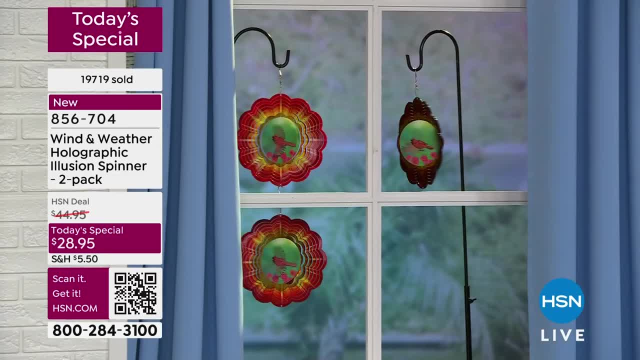 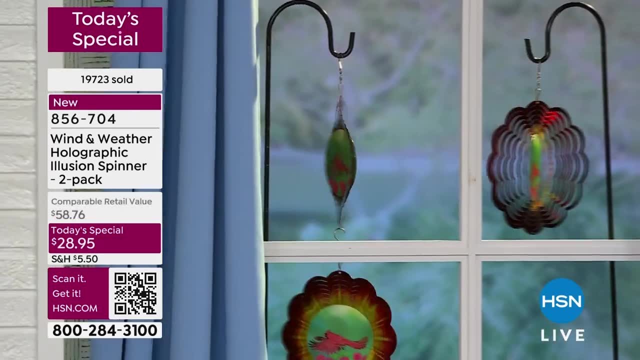 on the day And with only 19,000 gone, this will be the only day that we will ever offer this to you as a Today's Special this year, And it will be the lowest price That we have ever offered on a two-pack- And you mentioned that that one of these I mean. 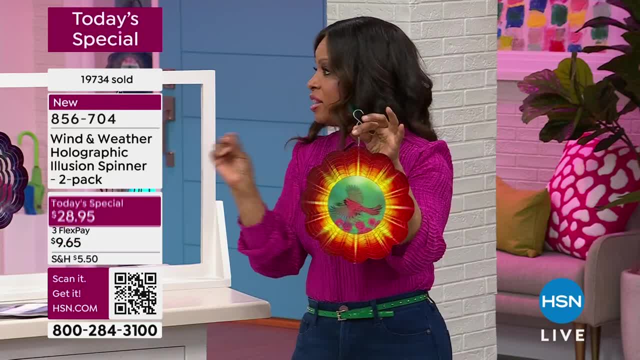 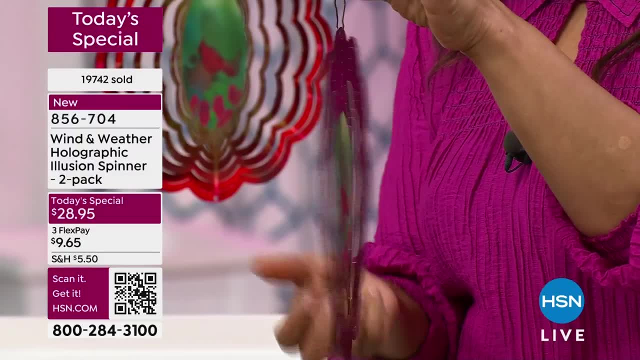 remember powdered coated steel. You get the hook, you get everything that you need to be able to hang these right out of the box. times two: What would you pay just for one of these in stores? Or if you were at an art fair, or- And that's where you would see something like this: 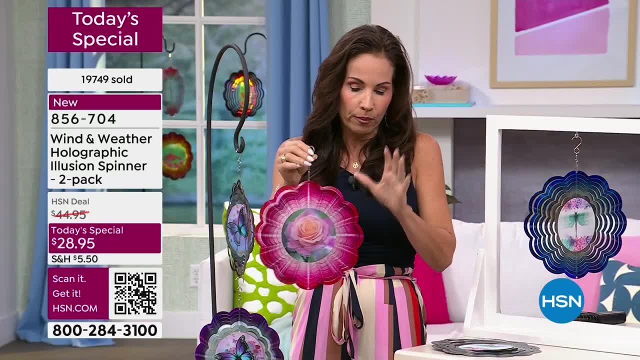 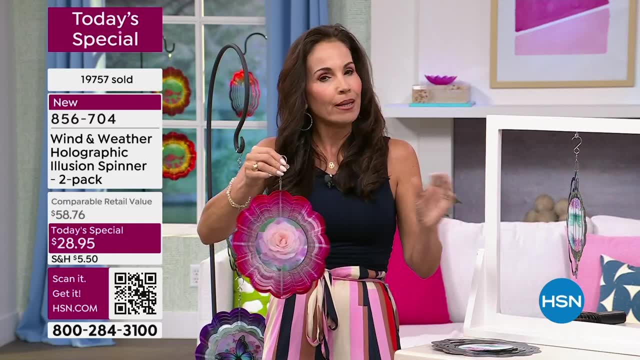 With wind and weather items, with their beautiful collections. that's where you would find them. you know, like art festival, It's the quality. And then maybe you look at the price and you're like, oh, I don't know if I wanted to spend that much. But here we are, celebrating our 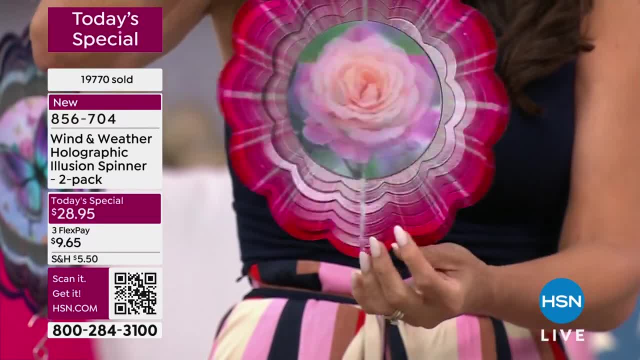 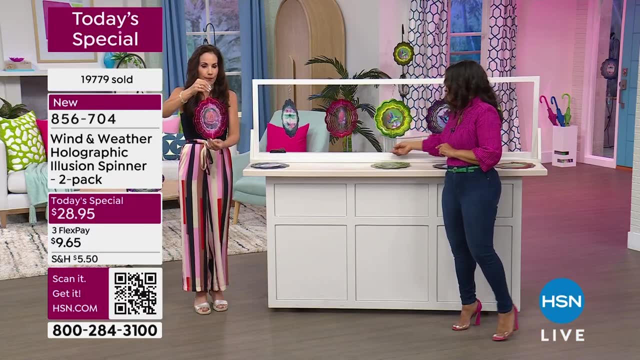 anniversary. We've made this just such a wonderful. I'm going to chime in there and interrupt you a little bit. Here's your update on the hummingbird. We only have about 500 remaining on the hummingbird, So I want you to take a look at that one. I don't know what happened to your fan. Let's find it. 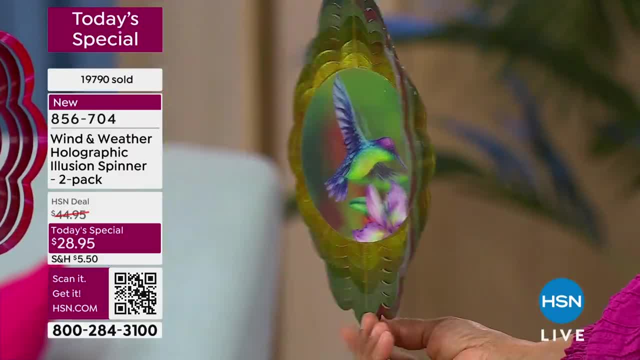 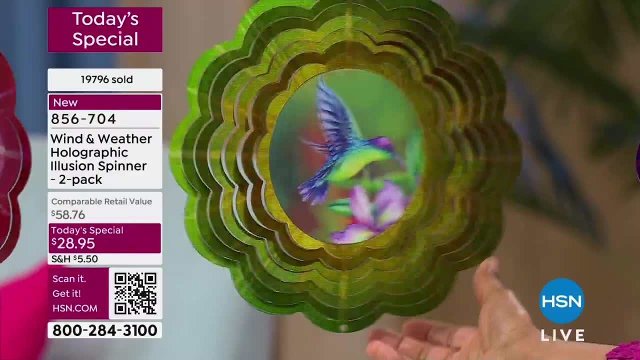 So here's your hummingbird. I'm just going to spend it just so that you can see 500 remaining on that hummingbird. That is amazing to me. Look at Front and back. So as this spins, you are going to be able to just absolutely love the design. 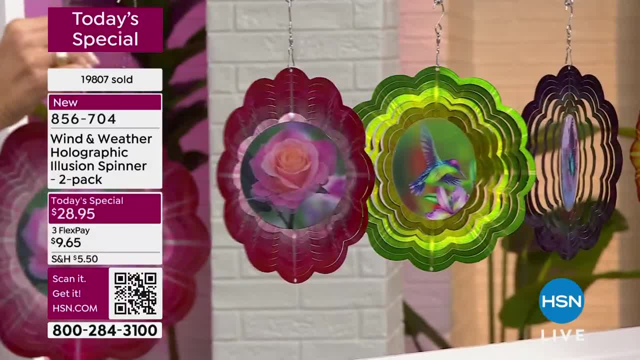 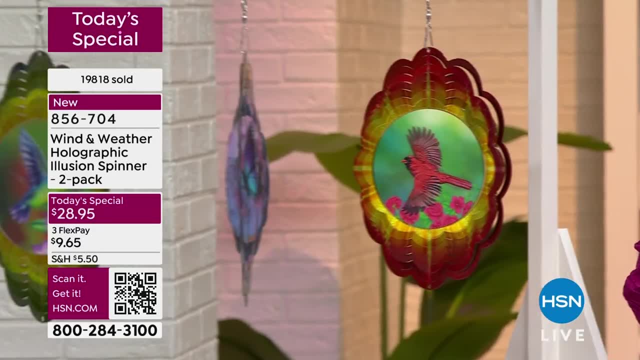 But there's your rose, Don't forget. we have the dragonfly. Your butterfly has been the number one bestseller on the day. And then, of course, I think so many of us are big fans of cardinals. But you'll need to order. We are offering flex pay. That means you can spread those. 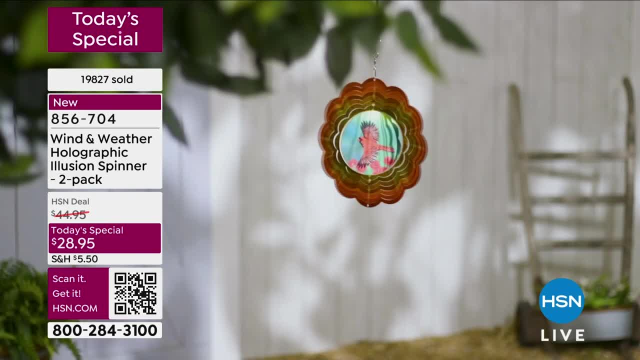 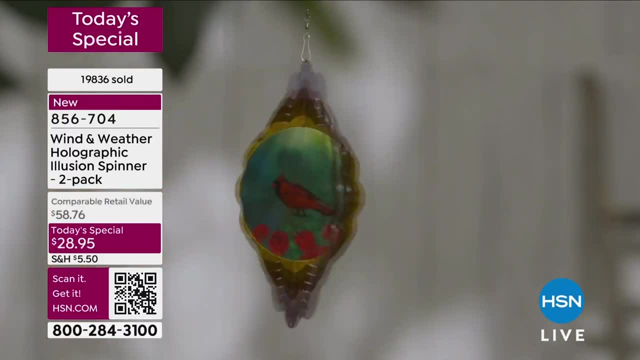 payments out over the next three months under $10.. But don't miss your chance to jump in on this exclusive. You can't find this anywhere else. It is the lowest price that we've ever offered on a two-pack. So one for me, one for a neighbor. 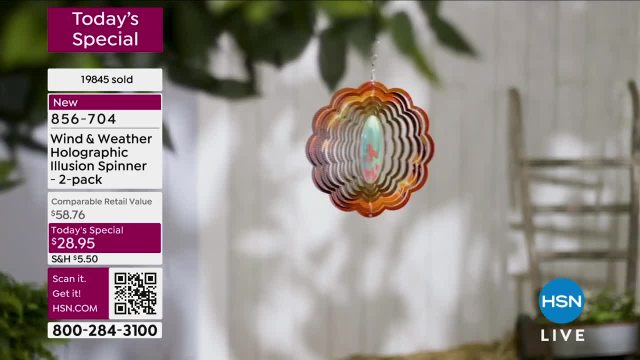 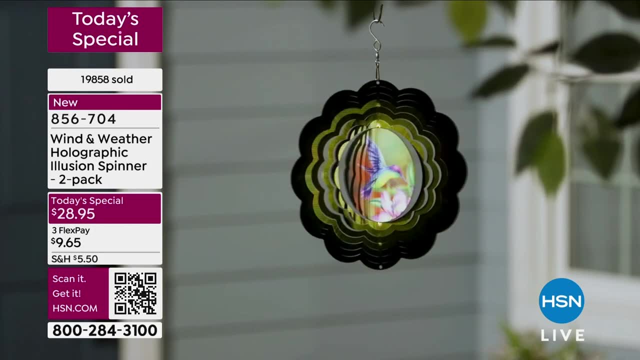 one for maybe the front of the yard, maybe for the side or the back, Because you know these are so versatile, As you see. you know you can hang it from a tree branch. Ty last night showed that he had three vertical in a space on a tree branch. It was absolutely. 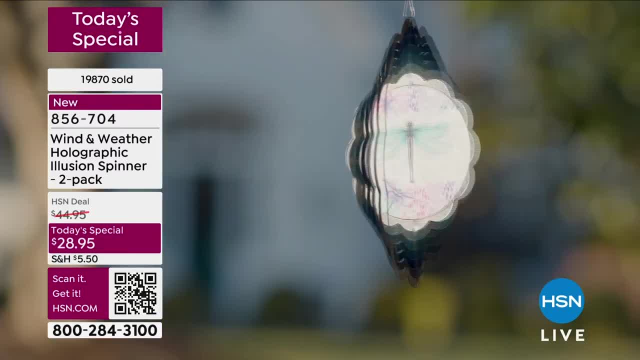 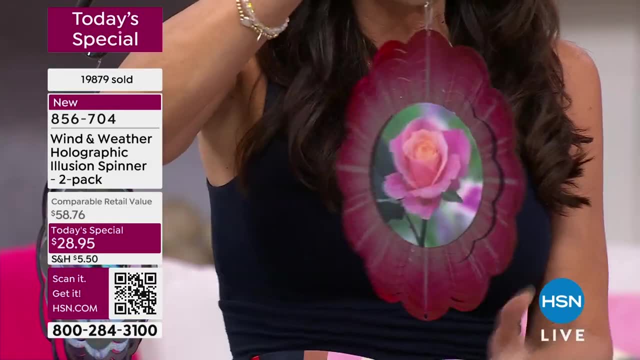 stunning. You can put them on a shepherd's hook, You can put them on a cup hook, anywhere, And they're light. So you know what I mean. You don't have to really use them. You don't have to use hardware. But I do want to mention something, Because when you get it home, this is how it's. 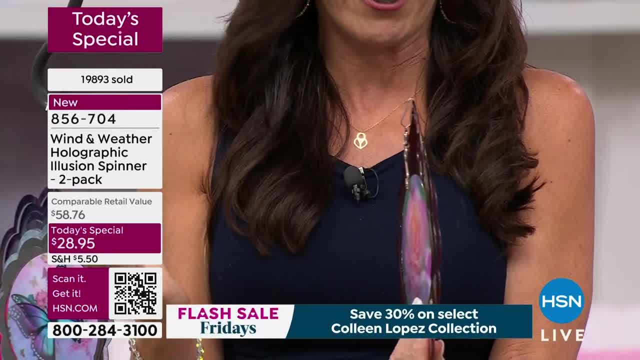 going to come. It's going to come in a flat box. So I don't want you to think, hey, I ordered a spinner, What's that? These are your two spinners, But it's going to come to you flat. And then what? 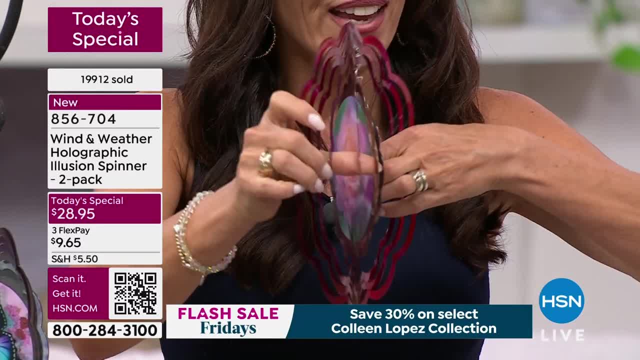 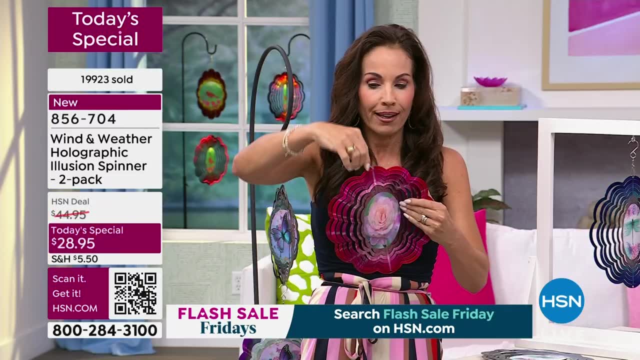 you do is you take it and you put your fingers and you literally fan it out. You see the way I just fanned it out, Because the metal is pliable, So it opens up. Here's your hook, And that's it. 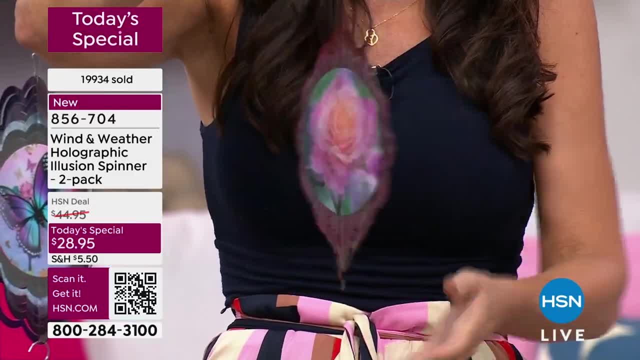 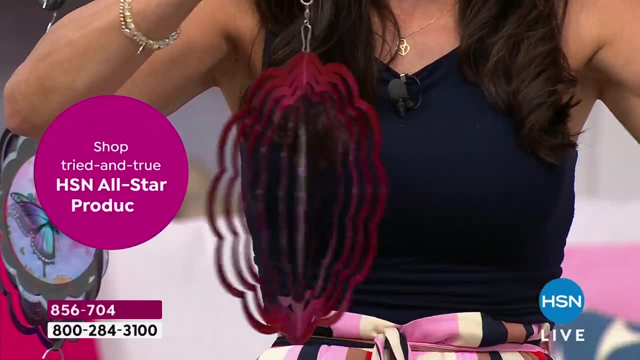 That's all you do. So this is simple. This is no tools. You don't have to do anything If you are sending this, maybe to your mom or your grandmother somewhere you know different in the country, if they don't live close to you. 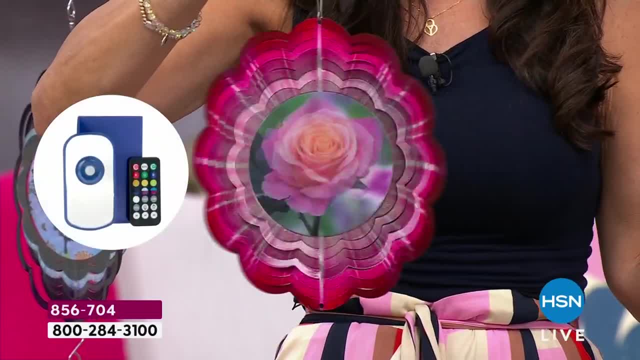 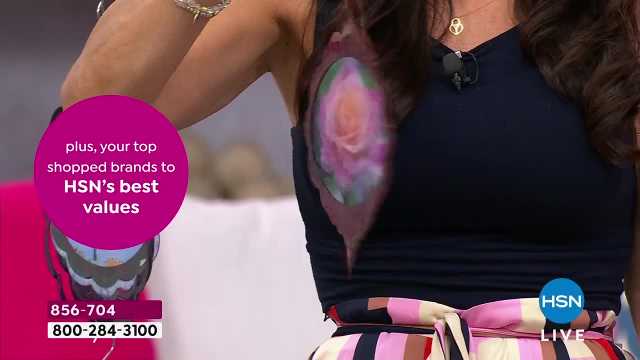 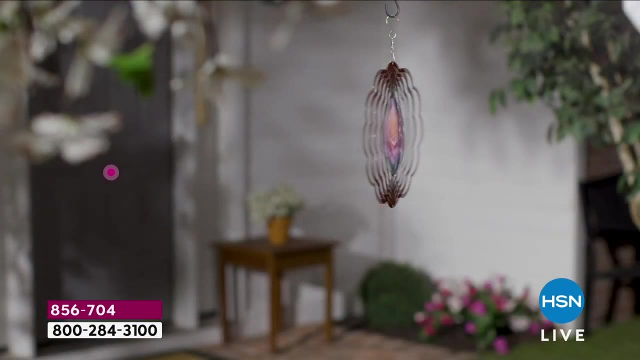 this will go right to them And there's no fuss here. You don't need a handyman to do anything, You just open this up, You pick your place And then, whoever you give it to, every time they see this spin, they are going to think about you. I'll tell you, I gave my mother actually about. 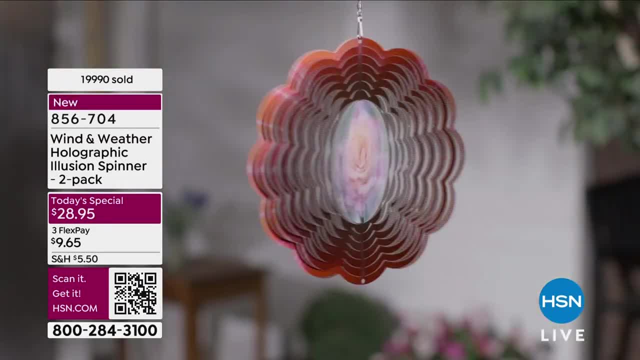 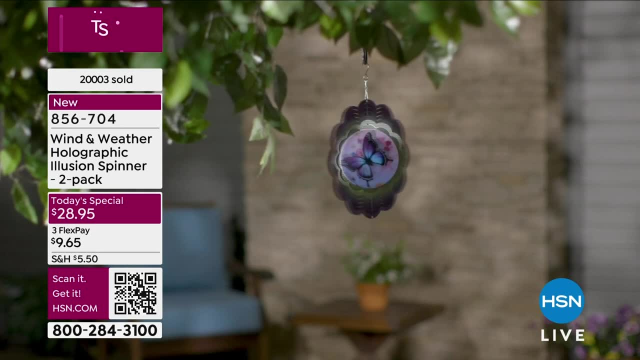 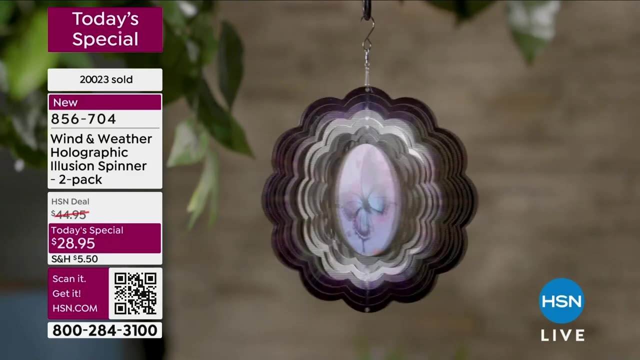 three years ago a spinner from Wind and Weather, And she loves telling people when they come by the house: where did you get that? My daughter gave that to me And you will get questioned because these are very unique pieces And whoever is at your house visiting or even your delivery person. 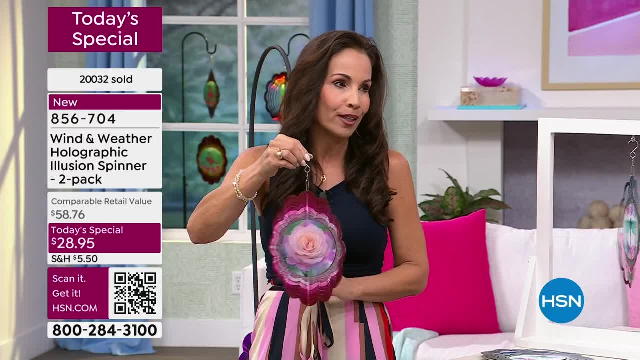 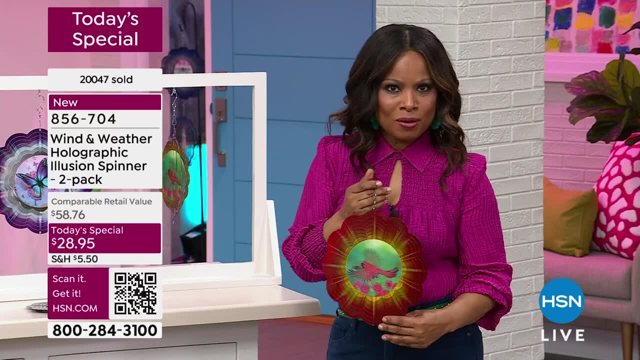 they're going to ask you about these. I agree, Because they're just different. You're not finding them in your local store. So here's what we're recommending: Place your order now. Well, here's what we've ordered. Only day of the year that we have this planned, Lowest price that we've. 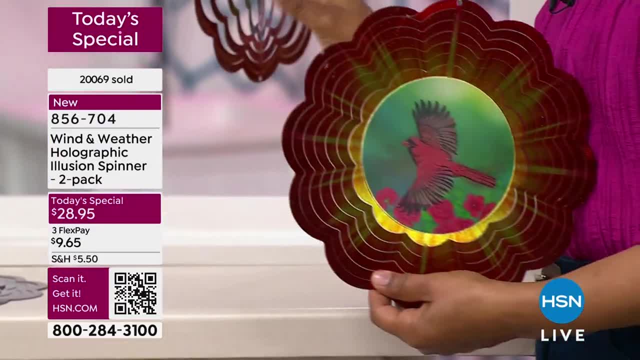 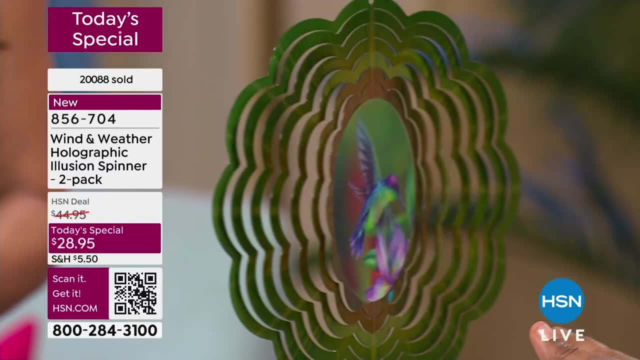 ever offered for a two-pack. Let us know which one is your favorite. Keep in mind that that hummingbird. fewer than 500 now remaining, So this choice will be the first one to sell out. We only have one more airing of our Today's Special, Only one more chance to grab this. 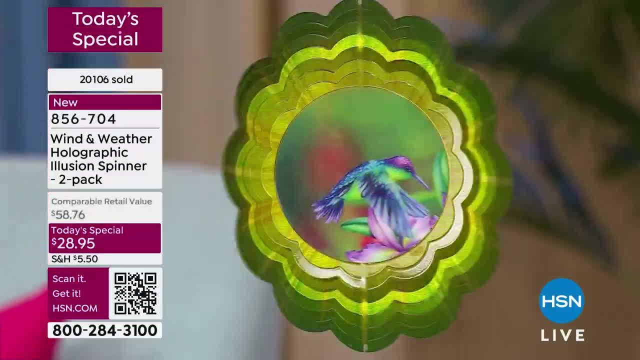 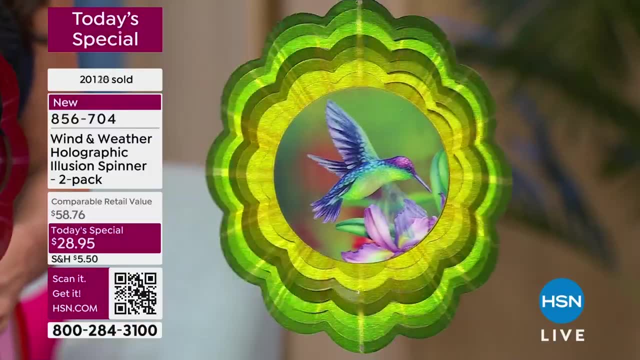 So make the decision. Let us know which one is your favorite. Many of you are buying multiples. I don't blame you. You know that you'll pay far more for something like this in stores. We actually have a retail compare of closer to $60.. That's about right. So these are, you know. 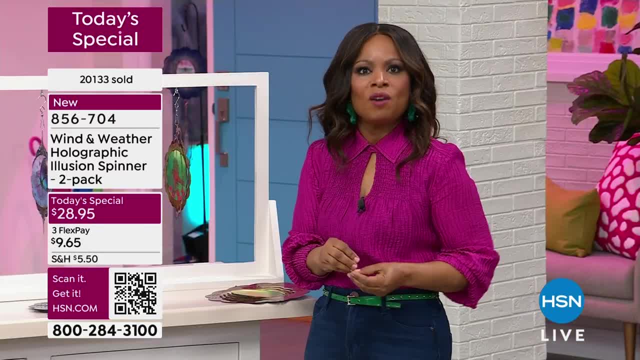 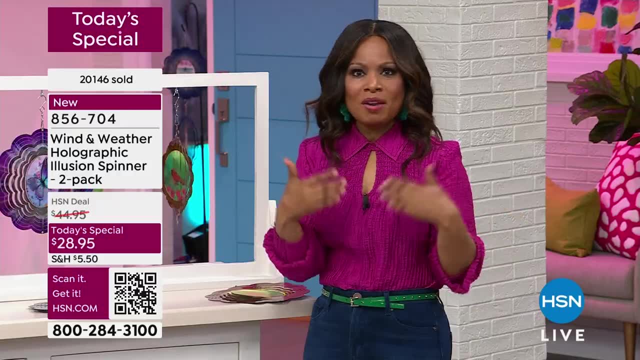 virtually- you know, comparing these to the stores- virtually half off. And when you're talking about the quality and longevity of powdered coated steel, you never have to worry about them. You never have to worry about them rusting or tarnishing in any way. They will remain. 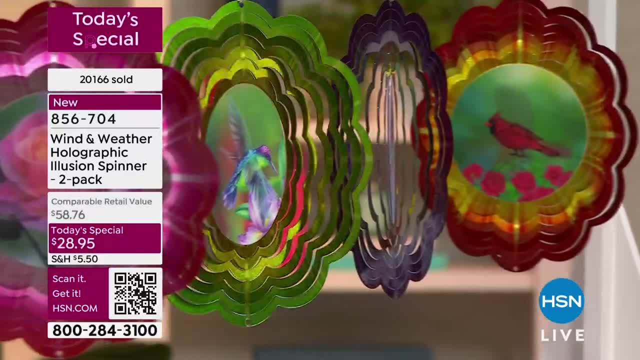 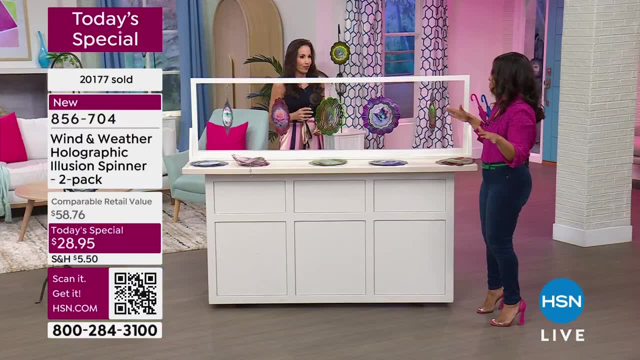 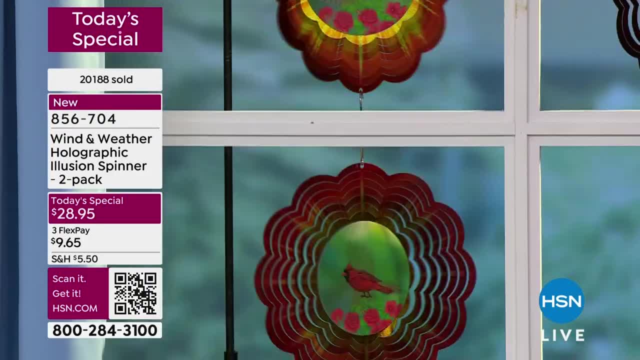 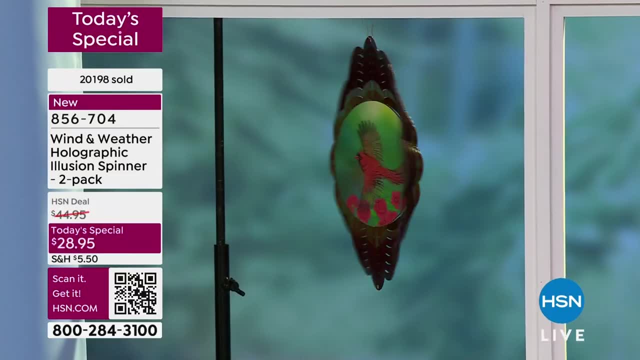 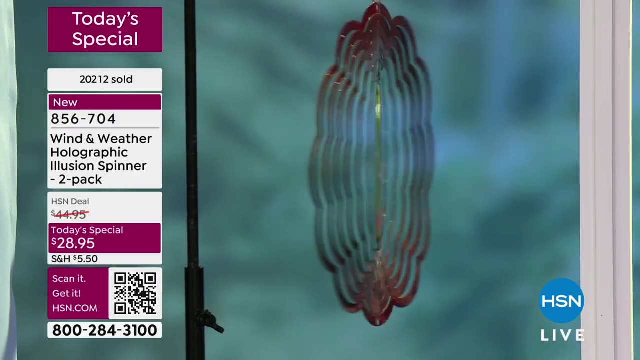 Look at the look at that Cardinal. Look at how that Cardinal- I mean look at the movement that you're seeing there and how that Cardinal is like in flight and that wingspan it is just moving. Look at how it's moving its wings. It's magical. That is incredible. You can't take your eyes off. 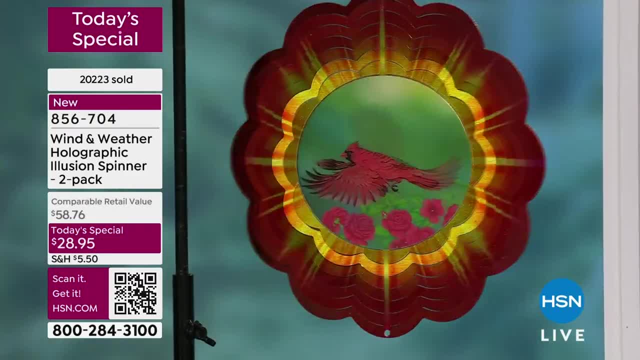 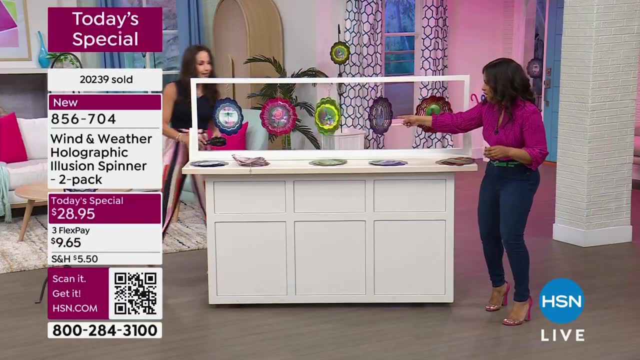 of it And remember: when this comes to your house, all you have to do fan it open and hang it, But people are going to say: what is that Right? Well, I want you to see the butterfly too. The butterfly has been the one of the best sellers on the day, And it is. look, just look at that. 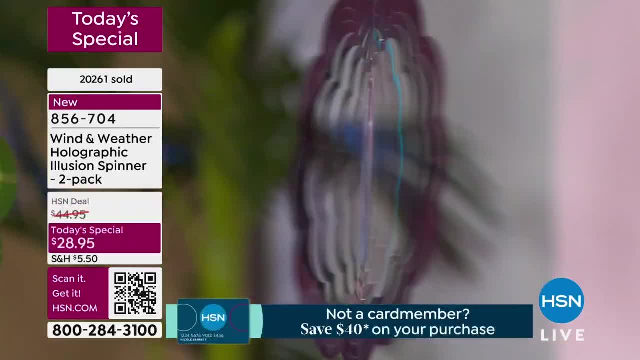 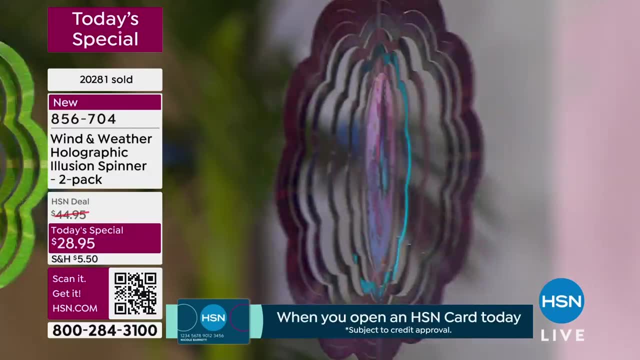 the colors of the purples and the blues and the blacks. And if you look carefully there's smaller little butterflies behind the larger butterfly- Can you guys see that? And there's also a little bit of a floral bouquet. So if you look in the back, you see how you see. 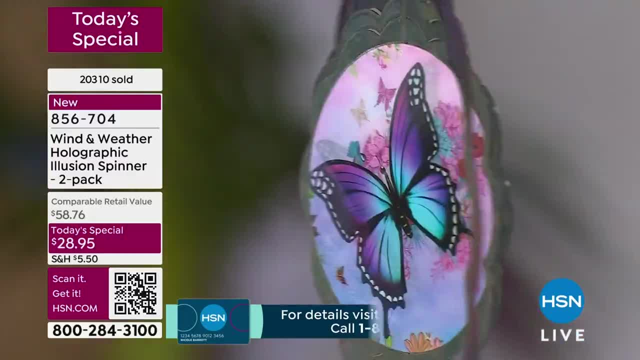 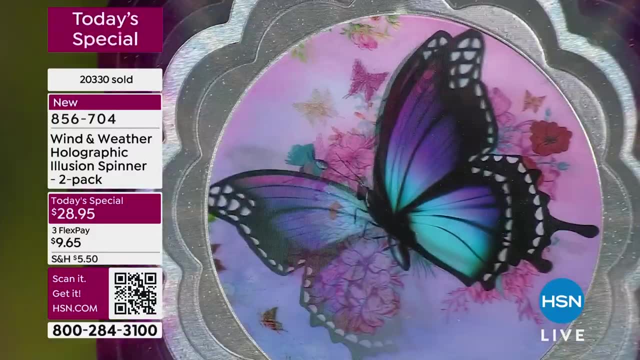 the smaller little butterflies in back. But once we put that fan on this and you can see how it will move by the way, 350 remaining in the hummingbird. So last call on that hummingbird If you'd like to have that hummingbird. 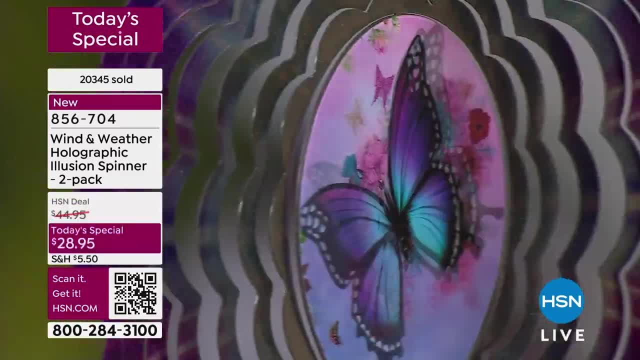 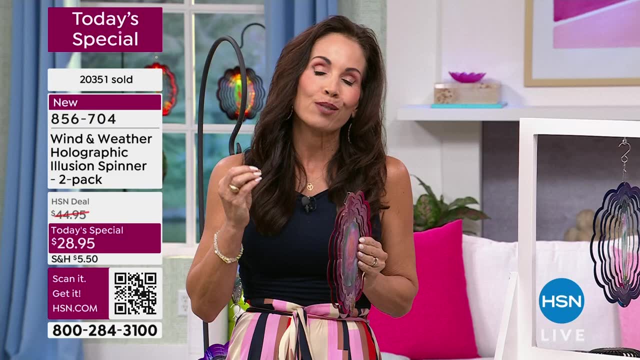 you'll want to call in there. It's hard to choose because they they really are all really, And I promise you, if you get these home as gifts, which you probably will just make sure you get some for yourself, because when you take them out of the box, right When you, when you see that, 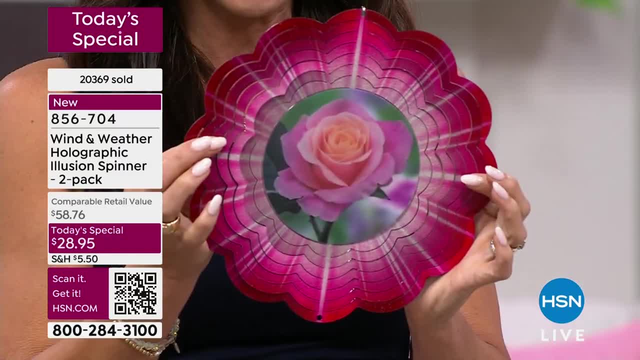 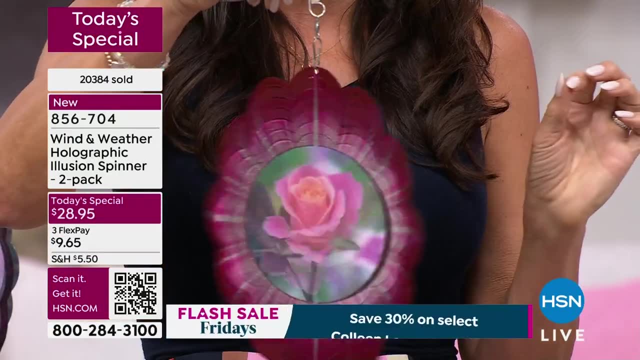 Oh, this is your spinner, and you take it out And you look at it and then you fan it open, Cause that's all you do And we're giving you the hook. You're going to give it one spin And you're going to say: I'm not giving that as a 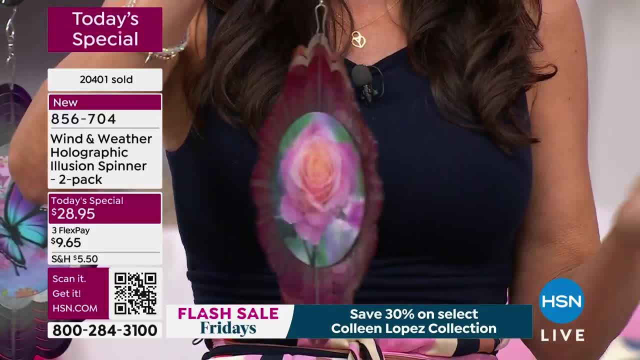 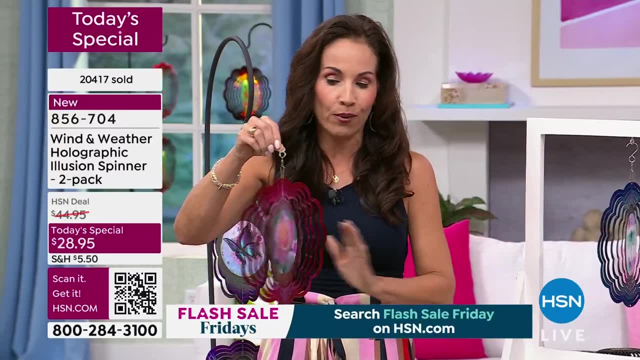 gift. I'm going to keep that for myself, So keep that in mind. And also I also want to mention: right after mother's day- we're coming around the end of the year- You always want to give teacher appreciation gifts at this price point. I think this is a phenomenal gift for a teacher. 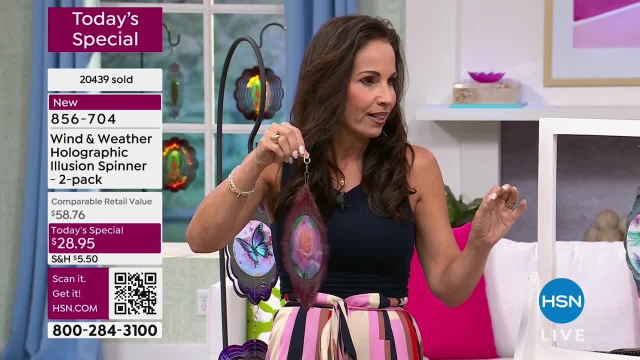 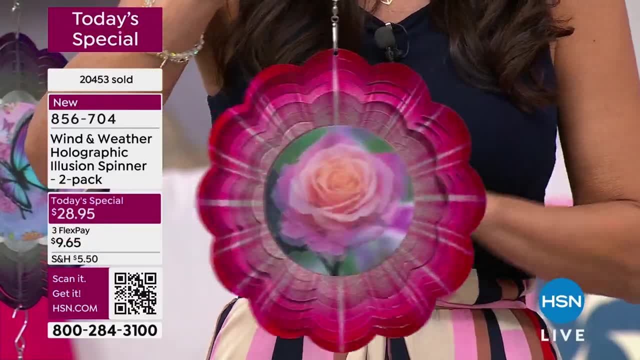 I remember struggling to always try and give a gift that was different. you know this. just, the value is so much more than what you're paying. And let me tell you, I'm all about giving gifts that have such a wonderful value but are different, like 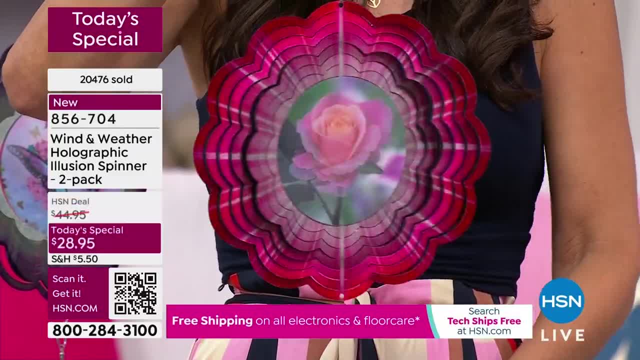 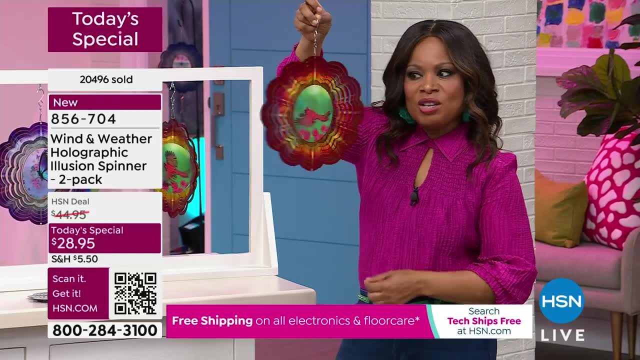 this. Well, if you'd like to shop, don't forget that we give you 30 days to make a final decision, with well over 20,000 that have been spoken for. Don't forget that you'll receive two of these, So you just let us know which one is your favorite. Remember, they're about 10 inches in. 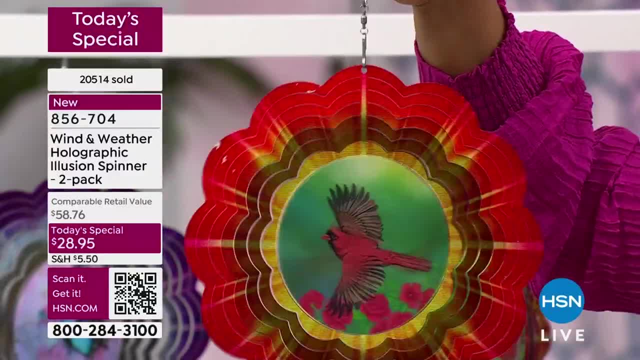 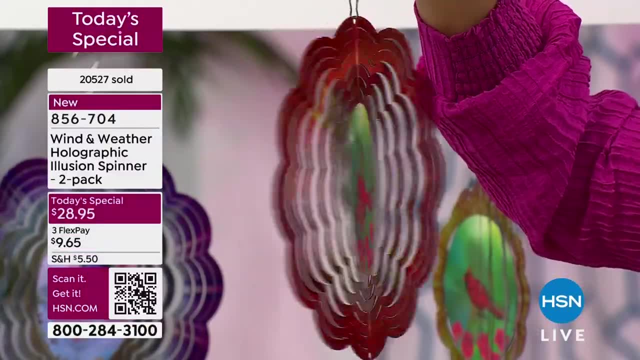 diameter. You're looking at powder coat of steel. The hook comes with it, So you don't need to do anything right out of the box. but look at that. Look at them again. I am, I am just absolutely just mesmerized. Imagine when. 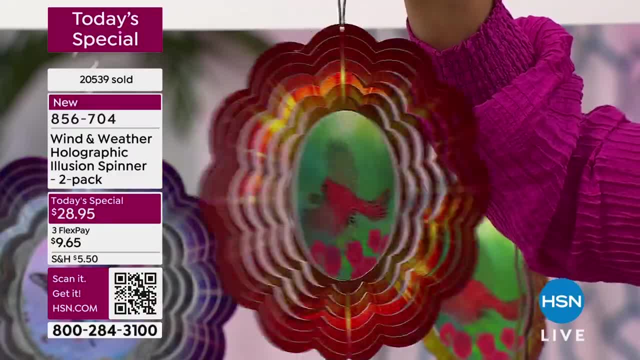 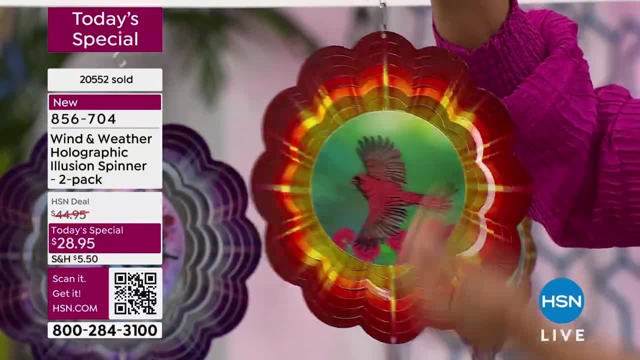 people come to your home and there's just a subtle little bit of wind, that happens and they will see this and they'll go. oh my goodness, where did you get it? I can't wait for you to unpackage them so that you can feel the quality. Many of you know that powder coat it still. 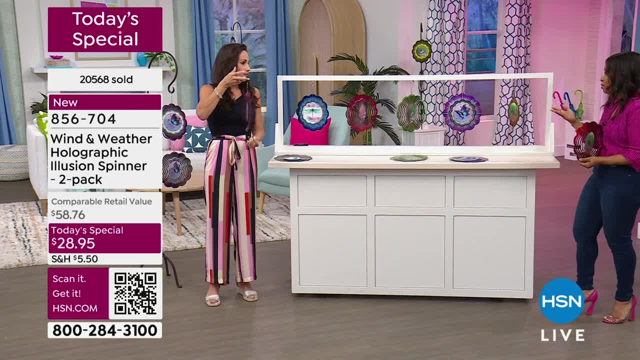 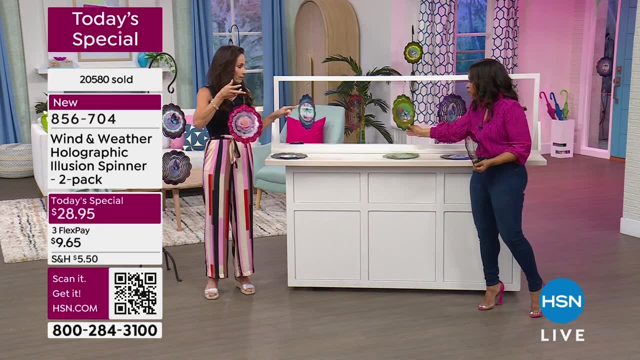 feels rich, It feels luxe. I personally don't have a favorite. I do think that they're all equally beautiful. I do know, though, in the hummingbird, that one is almost completely sold out, So I want to give you a close look at that hummingbird. give you an. 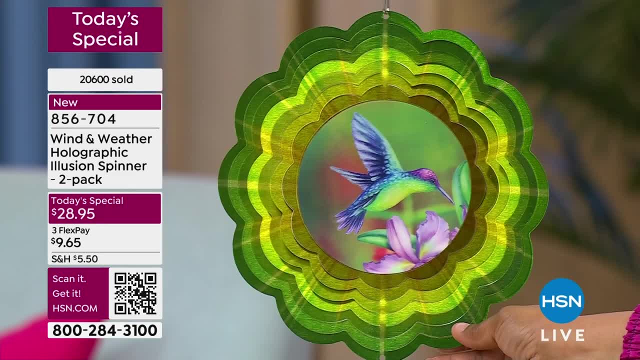 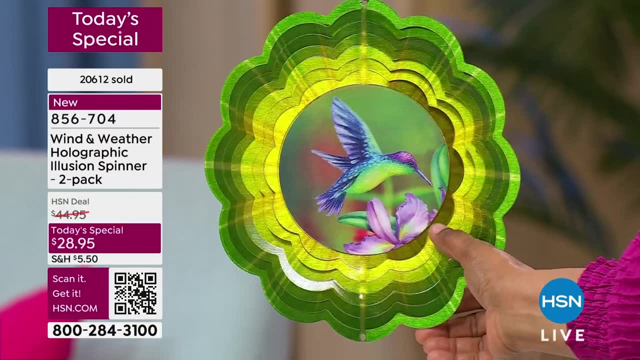 opportunity. If you love greens, green is certainly one of my favorite colors. The hummingbird has a little purple in it, a little blue in it. It does have a pretty little flower at the base, as you can see. So it's looks like it's going to go in and right. Yes, it does. And then when it starts, 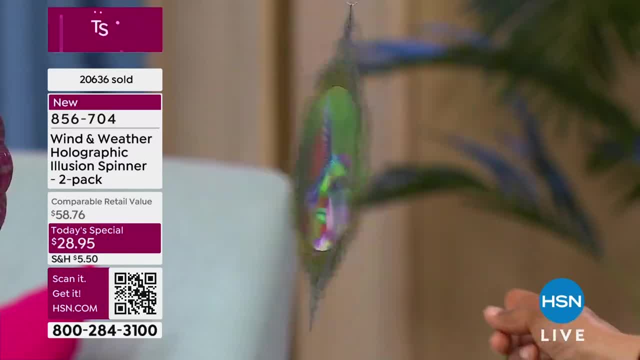 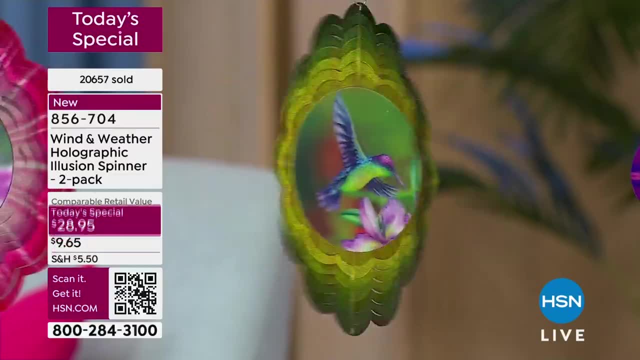 going. it just flaps. So let's show it to you. The hummingbird will sell out. So if you'd like to have that hummingbird, look at it, go now. It looks like we kind of came upon it and it's like, okay, I'm leaving, I'm going to take flight and I'm going to leave The butterfly. 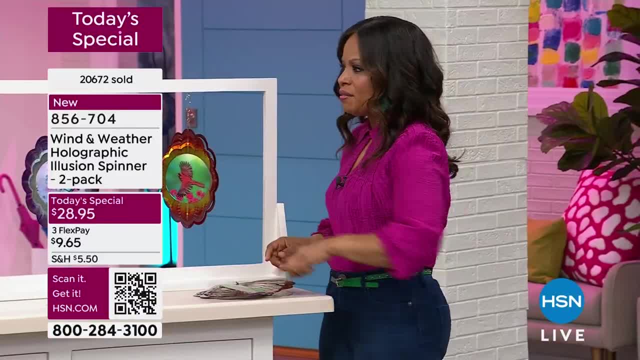 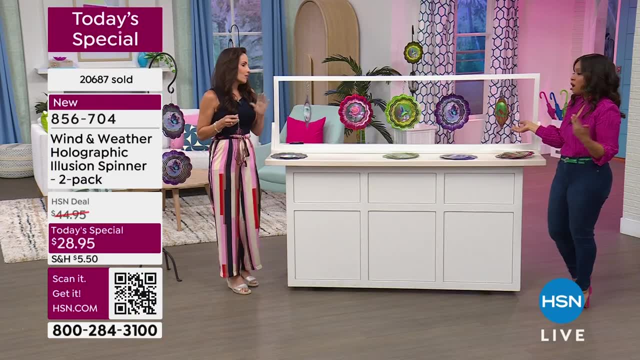 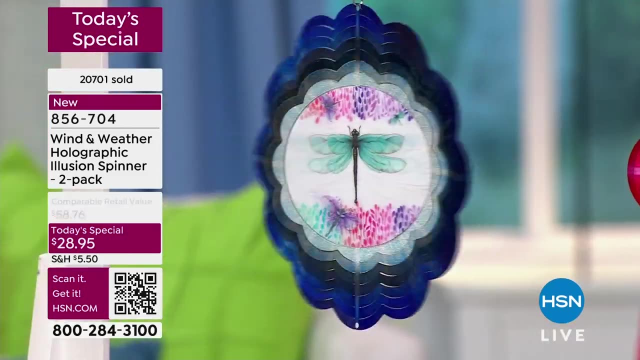 has been the number one favorite on the day or the best seller on the day, But the dragonfly, I think it's really great. The rose and cardinals are a fan favorite. It's always a favorite, And what I like about the choices that Wind & Weather made here is all of these, all of these motifs. 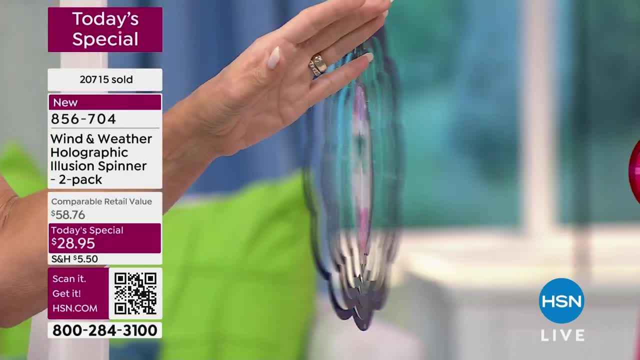 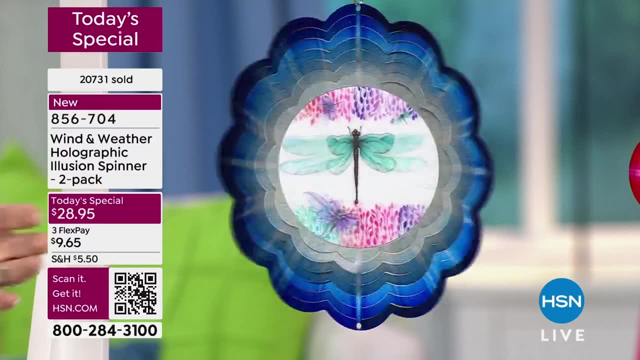 mean something different. to somebody Like my daughter's- a butterfly girl, you know- and like the dragonfly, that means positive change and transformation. I know I have a, my best friend. when she sees a cardinal, we walk the dogs together and she'll see a cardinal. She'll be. 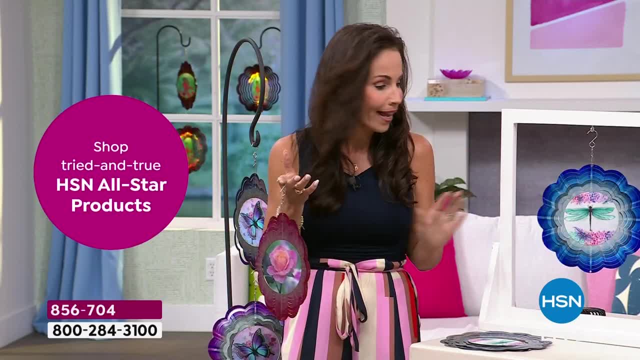 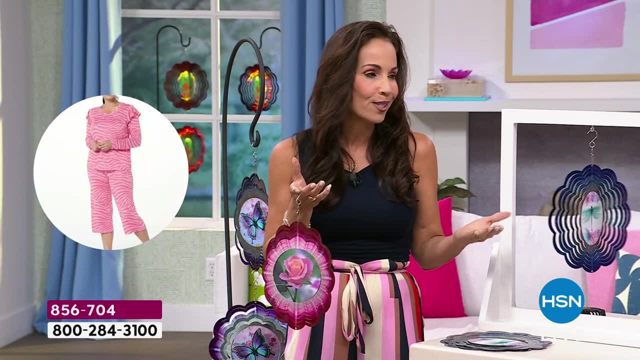 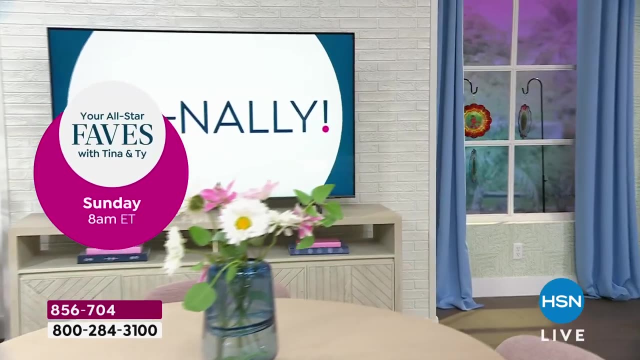 like: oh, dad, you know it makes her always think of her dad. So I'm actually going to get my best friend, the cardinal, for Mother's Day, And it's just the fact that they're so personal and they're they have such meaning for us, The hummingbird. I always think of my father because we spent some 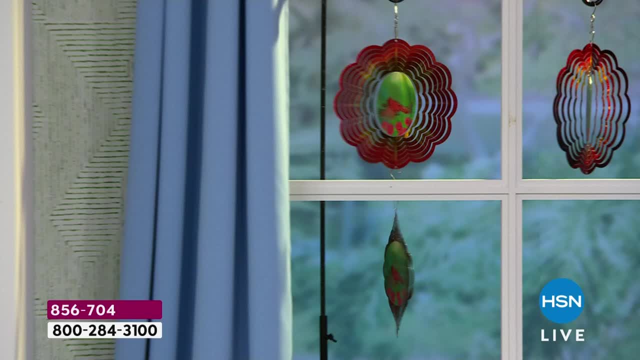 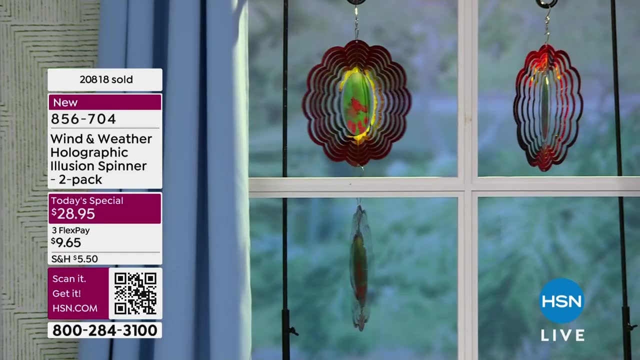 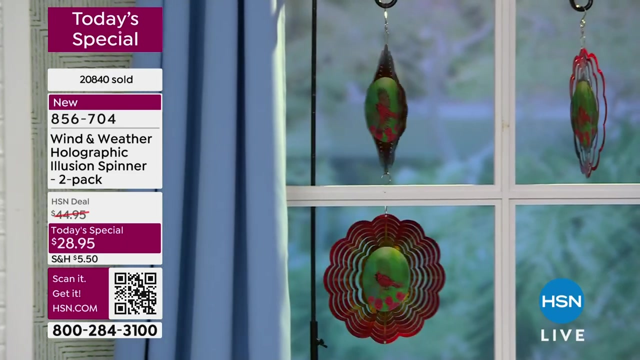 time, you know, in a cabin and we watched hummingbirds for hours. So you know, everybody has that type of story. We all know someone that loves one of these And if they don't, I guarantee you they love roses. But what this enables you to do is it lets you give a personal 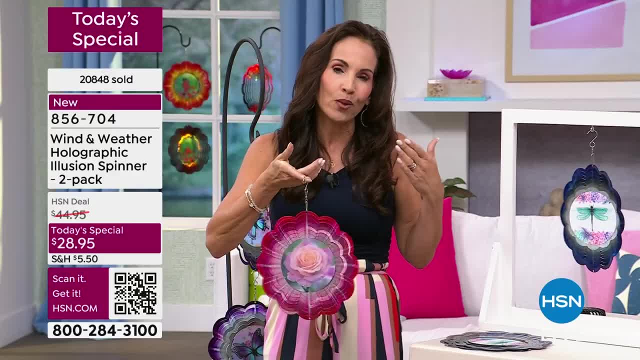 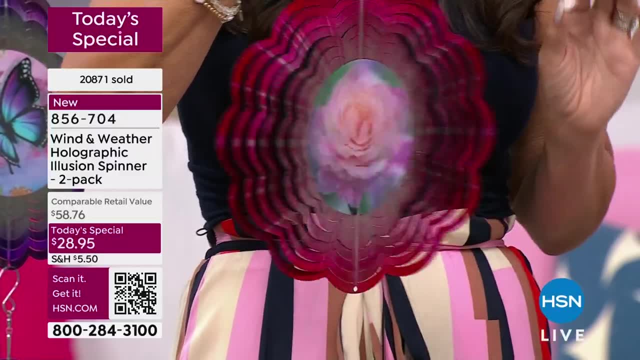 gift, which I always think is so nice to give something where someone knows: hey, this, this person really knows me. They're giving me a cardinal or a butterfly because they know that's what I love And, again, they're always going to think of you when they see it spinning. 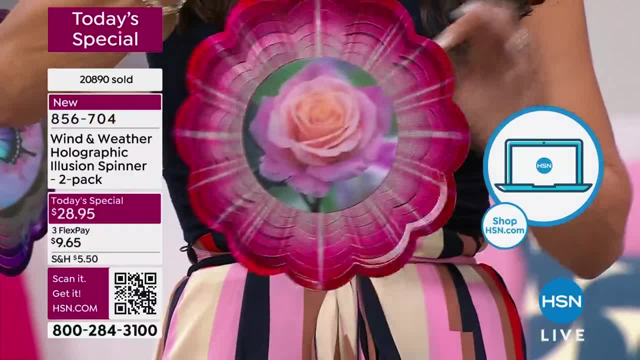 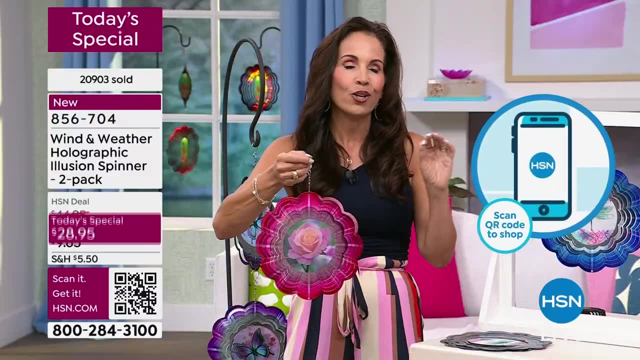 When you get this home, I recommend putting it somewhere, maybe where you can see it from indoors- Maybe if you have a kitchen window and you know you cook a lot or you're washing dishes- because you'll glance outside and you'll look at it, It'll catch your eye, It will put a smile on. 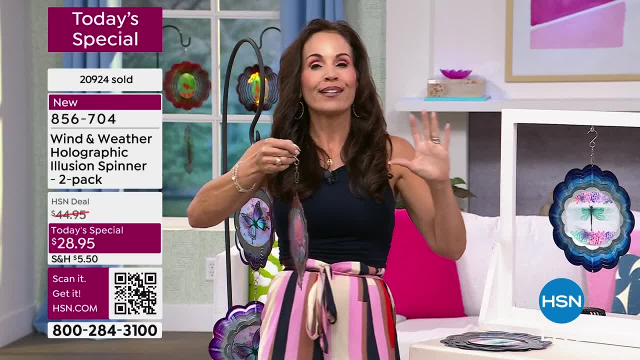 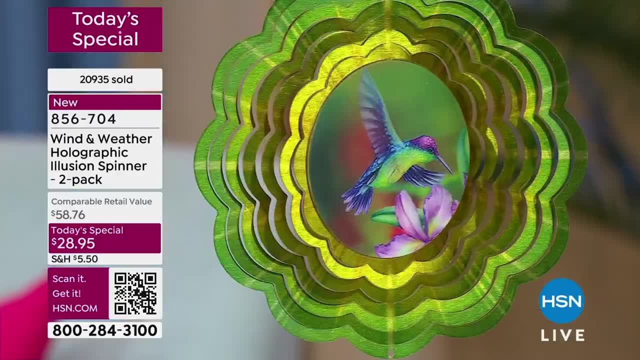 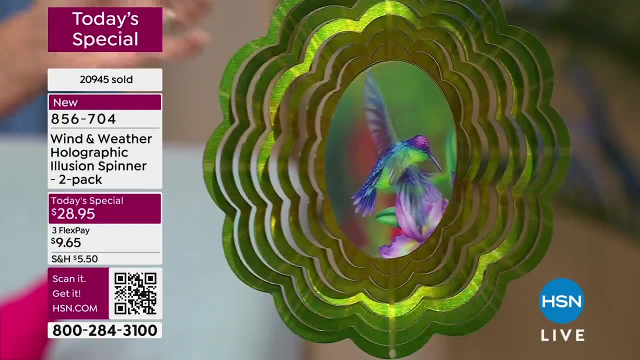 your face without you even realizing it, And it's a great way to give a personal gift. I have mine outside my um, I have um a work office and I have it right outside with some other nature birds, you know, go around it, And just yesterday it was storming and it was windy. 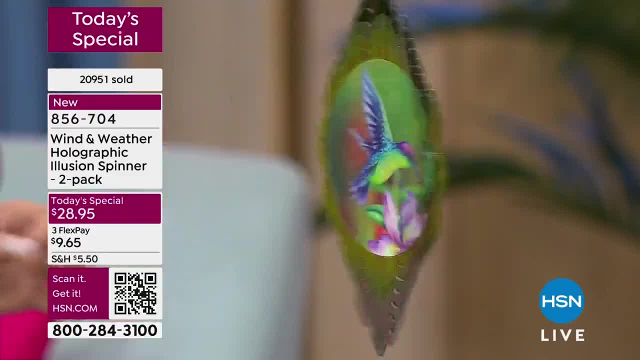 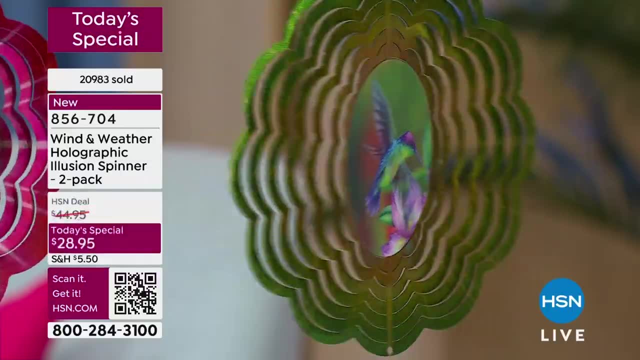 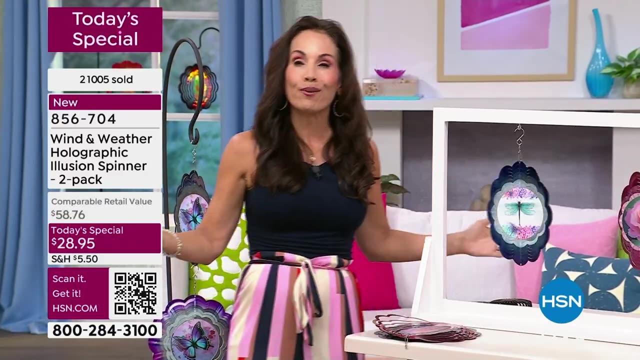 My spinner was going and this looked gorgeous, with rain coming down because of that metallic paint. So I want to remind you: this is the quality of wind and weather, So let it rain on it, Let the sun shine on it, If you are somewhere in the country that still has. 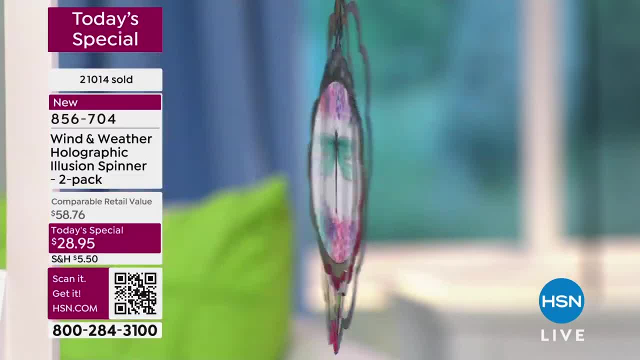 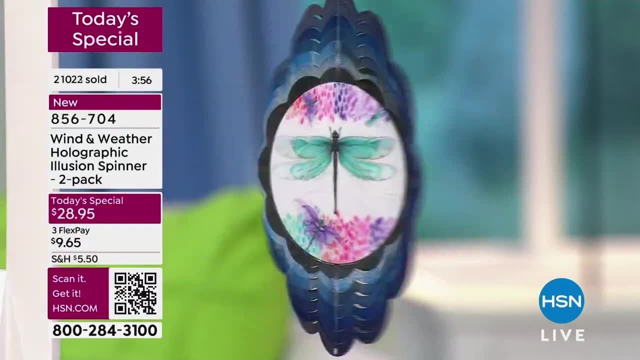 snow, put this out for a pop of color immediately, And then, once your lawn in your garden starts evolving, move it around. You're right, Move it around to different places. different shepherd's hooks, different, you know- cup hooks in different places, different tree branches. It's easy to move. 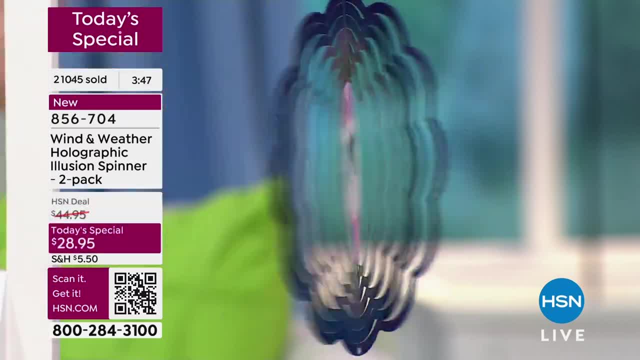 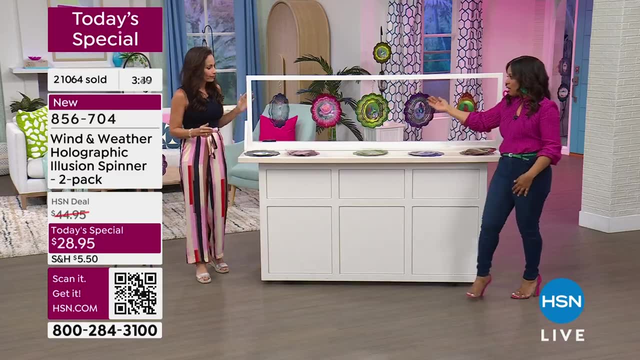 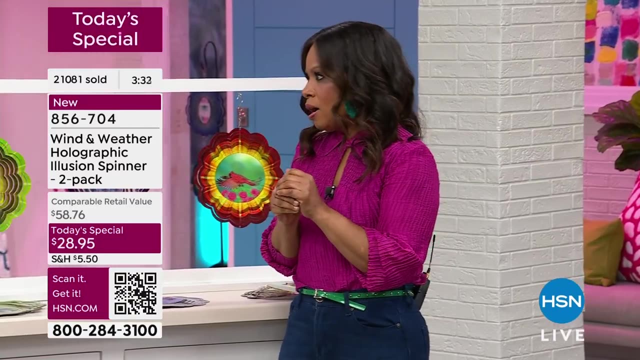 around And, uh, okay, You get in here, Cause I know you have an update for us, So our hummingbird is now completely sold out. Okay, We, in fact, are going to leave it here. Oh, what a beautiful choice. I mean, they all are gorgeous. I will say this: If you're an artist, um, if you love color, 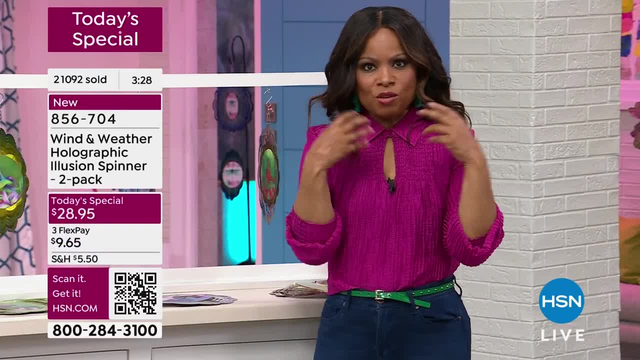 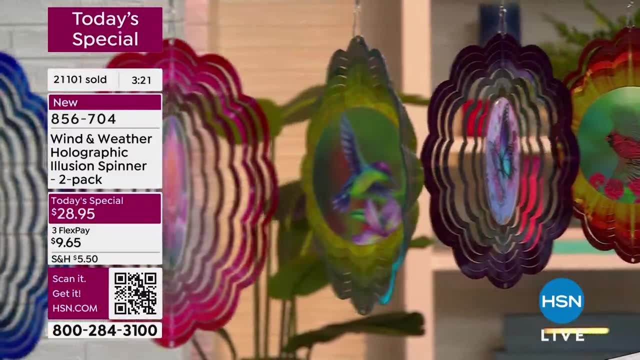 and I know sometimes on televisions not everything translates beautifully. These are stunning in person. They are absolutely stunning. The colors are so vivid and bright and three-dimensional. So the hummingbird is sold out. We know that the butterfly continues to be very popular. 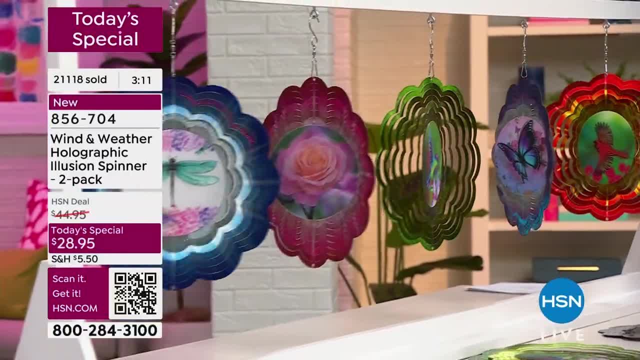 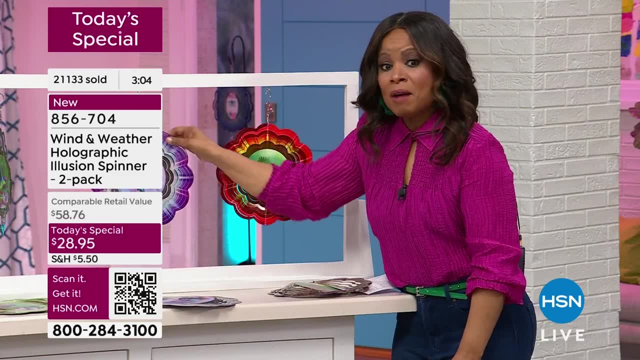 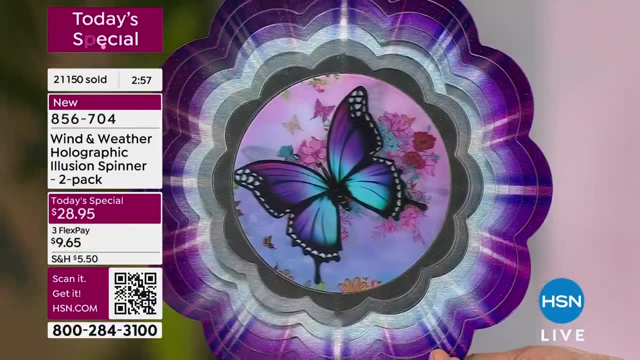 but make your decision. 21,000 sold on the day And I have just been given the update that the next one that could potentially sell out will possibly be the butterfly. So if you'd like to have that butterfly- and, by the way, next airing is going to be the final presentation, Just look at that, as I just 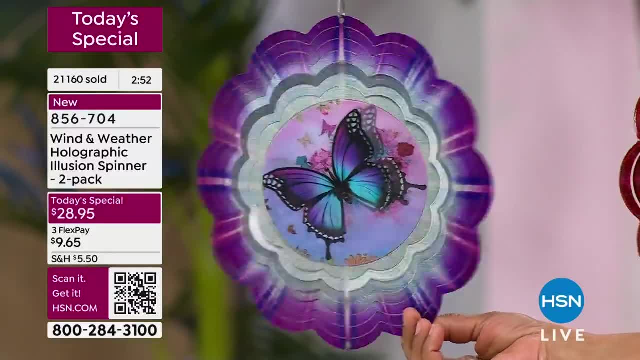 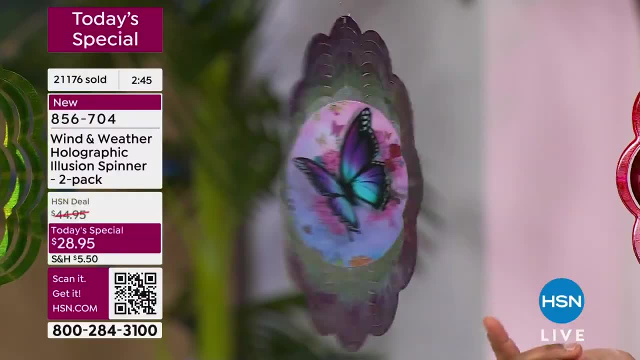 kind of rocket side to side, but look at how that wing just moves right here. I'm going to spin it just a little bit and you can see how it goes. If you'd like to have it, don't forget times two as our best value of the day. 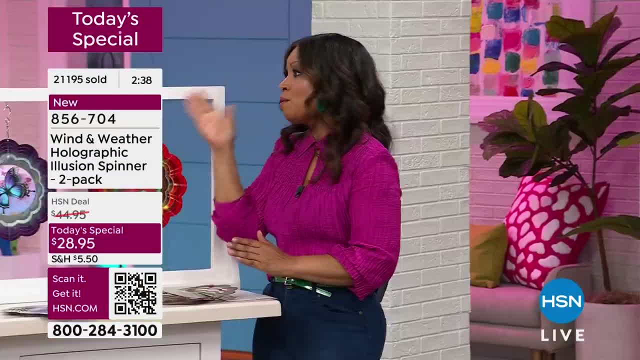 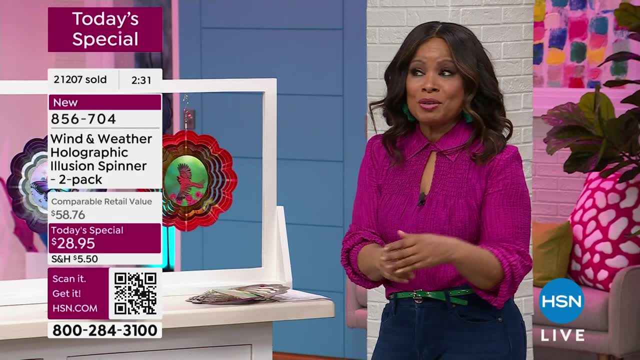 Lowest price that we have ever offered. Don't miss it. I agree with you: These make for amazing gifts to be able to give, And I would buy more than one set. You'll be thrilled. Your neighbors will ask you about them. They'll go: what did you get that? And you can't find these anywhere else. 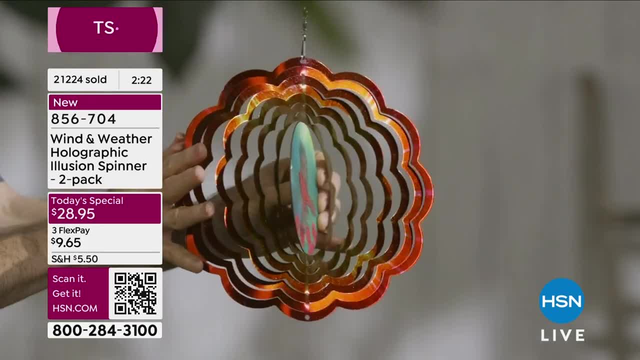 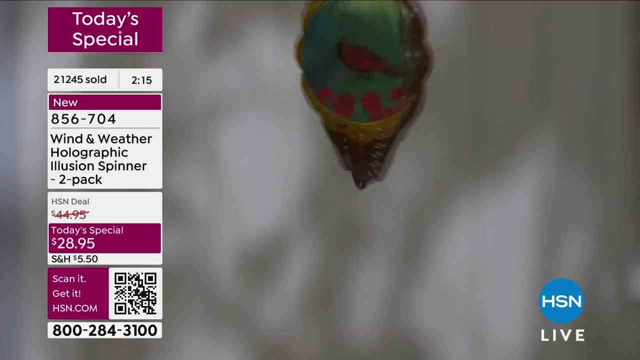 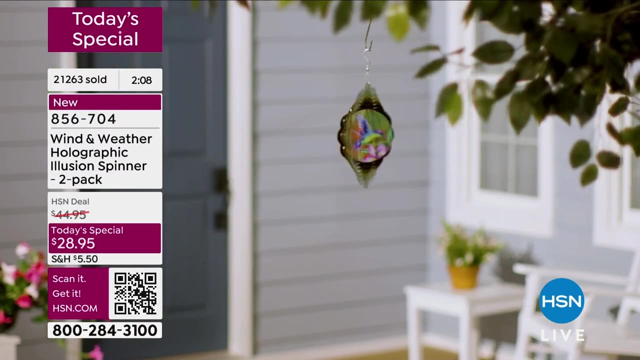 They're exclusive, They're only available here. Remember, they're made of the high quality powdered coated steel. So this is it? paper or plastic or something inexpensive? laser cut metal, Actually, laser cut metal- Beautiful. A lot of you have been to art shows and you've you've seen this level of quality. It. 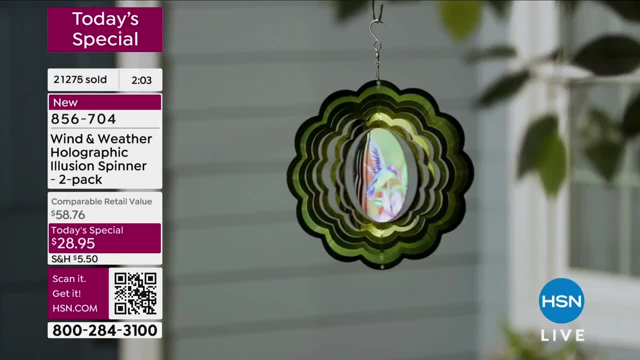 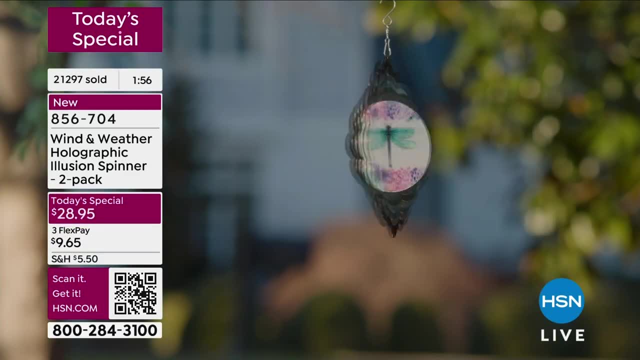 can be very expensive to purchase products like this, And we're so thrilled to be able to partner with wind and weather to bring to you this holographic illusion spinner. We've never done this before. We're thrilled, You're, you're. this is virtually half off, Um, but you do need to make. 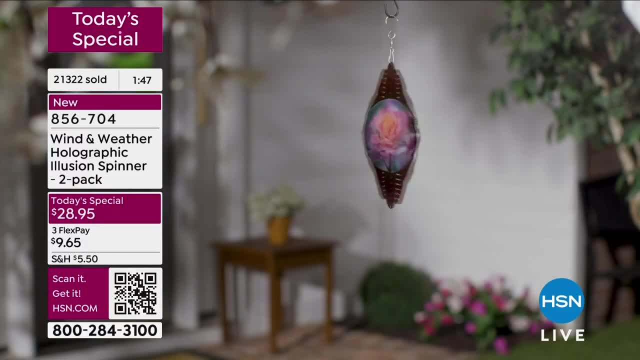 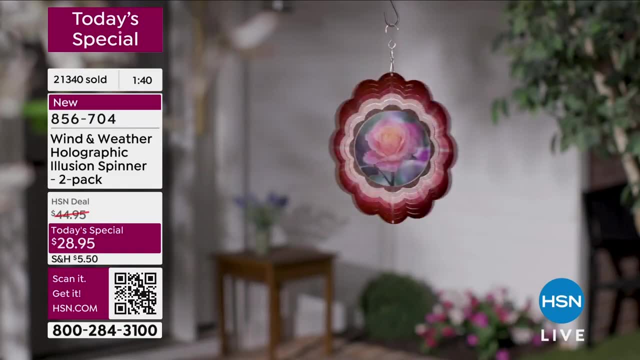 a decision and you have to be fast. Um, Yvette only has one more show and it's a limited presentation, So please go go for it. Um, just sendcom shop the QR code. Um, I'd love to go down the aisle event. I think we have a minute. 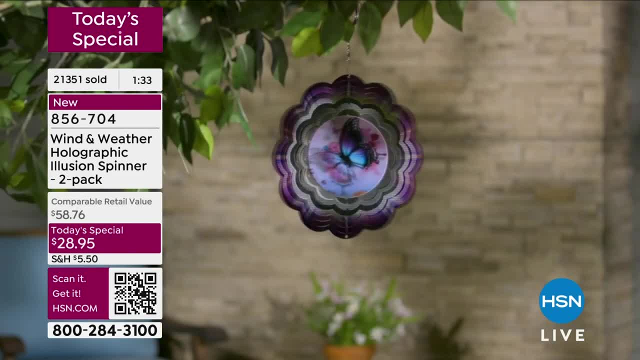 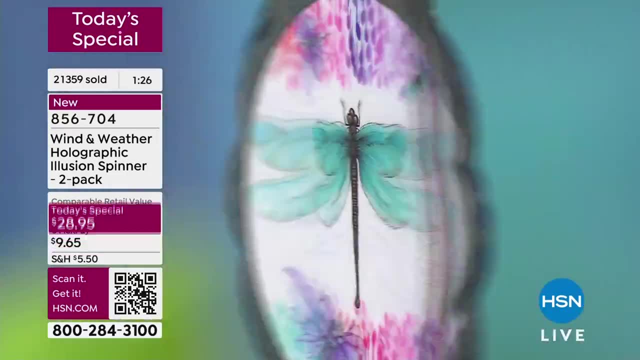 to kind of show everybody once again. I'm going to take my little fan here and just do a little bit so you can dragonfly. So here's your dragonfly, There's your blues, some silver, you got some purple in there. Um, the dragonfly is a symbol for positive change. I love that. And then you. 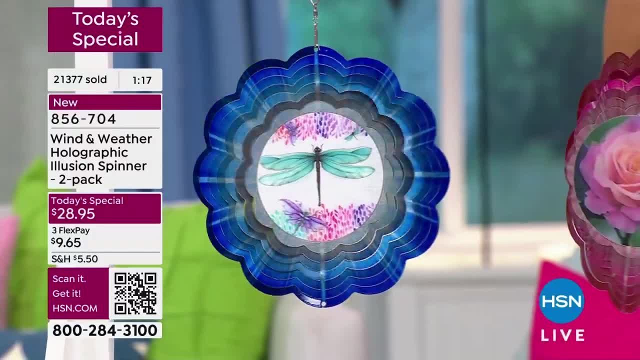 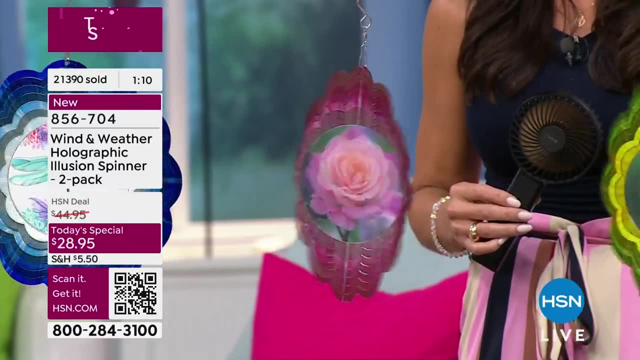 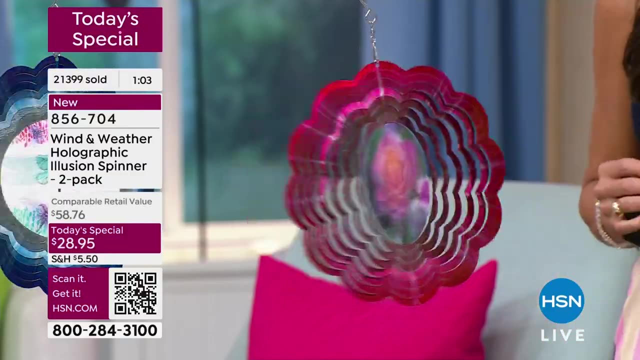 have your rose, which I just love the way the rose just blooms in front of you. So, and you know, for mother's day, isn't it? wouldn't it be nicer to give her a couple of these roses instead of roses that are going to die? and this is much more affordable as well, I think. I think. 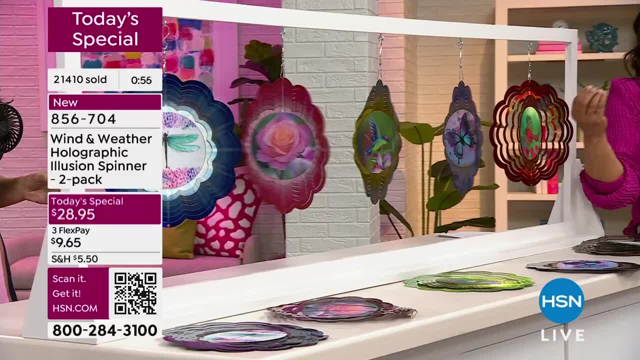 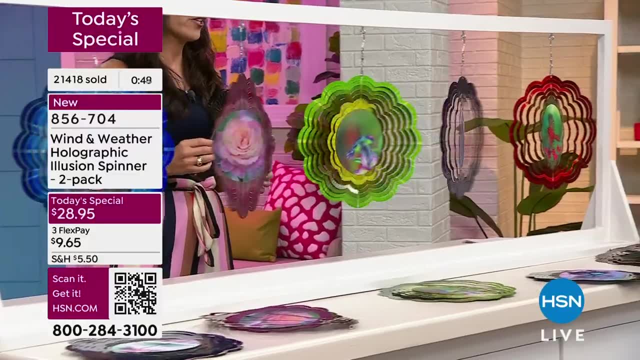 that's a good point, because every time someone's someone looks at this, they'll be reminded of you. We know that our hummingbird has sold out, but let's go to the butterfly. The butterfly will be the next to go. We know, you know your butterfly girls. I guarantee you you have a. 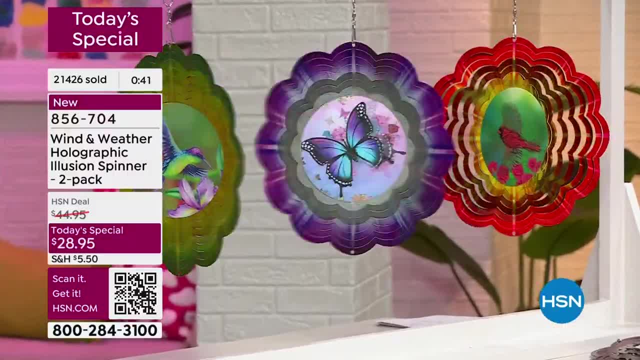 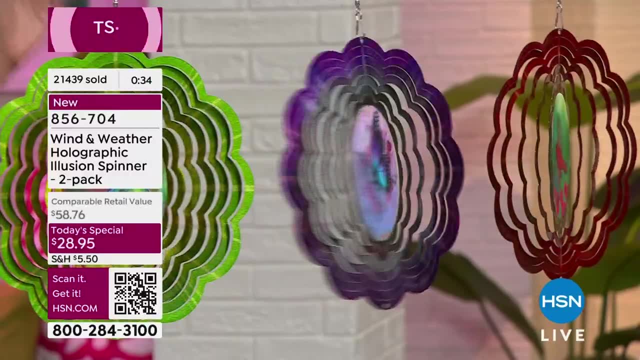 right a friend or family member that love butterflies. Oh my gosh, They would go mad over this. They love purple. I mean, I love butterflies too. I mean they're, I mean they're all. it's just hard. You know a story real quick, which reminded me So. 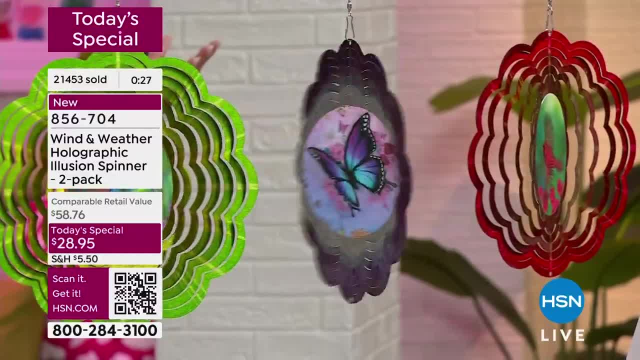 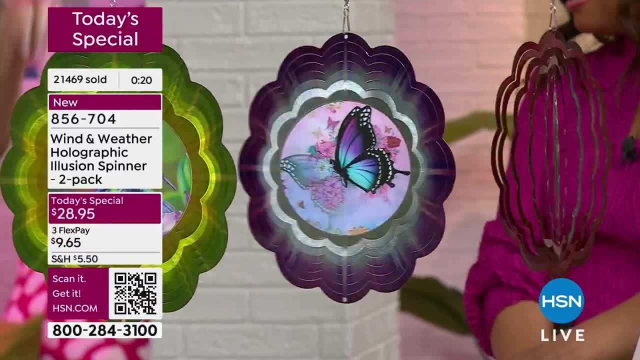 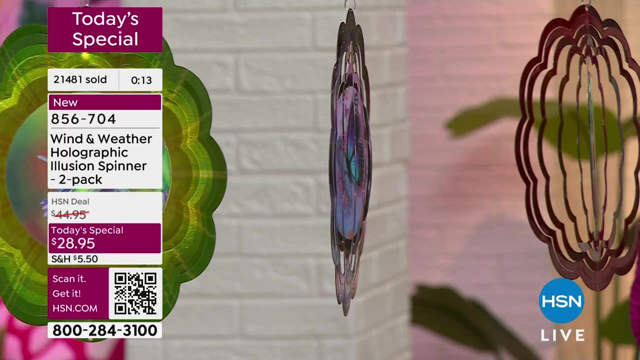 one of my good friends' daughter's getting married and I guess these days showers are themed, So the the bridal shower was themed butterfly. She picked up a couple of these, hung them on the table where the desserts were. It was stunning. I mean, how about that? 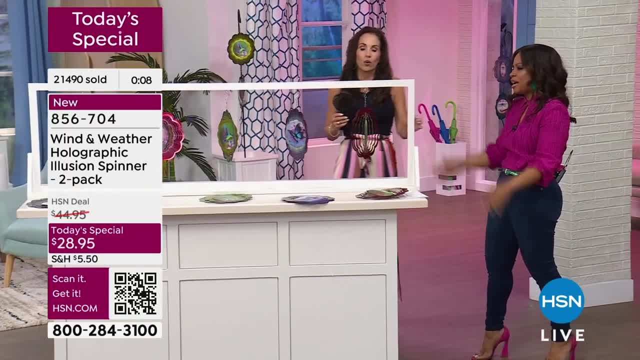 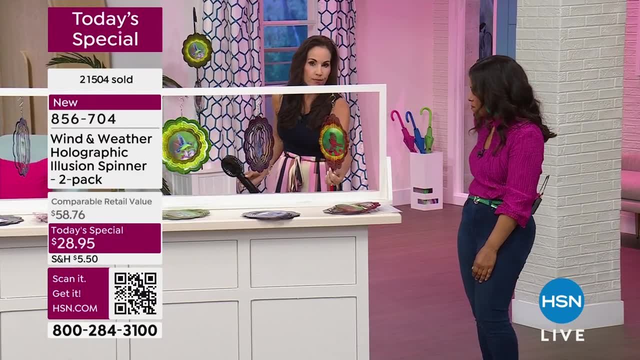 I think it's great. Yeah, And Cardinals are incredible, right. I think this would be beautiful for Christmas, you know, because we always like Cardinals and Christmas. So put this out in the snow and just incorporate it into your holiday decor. We always love our. 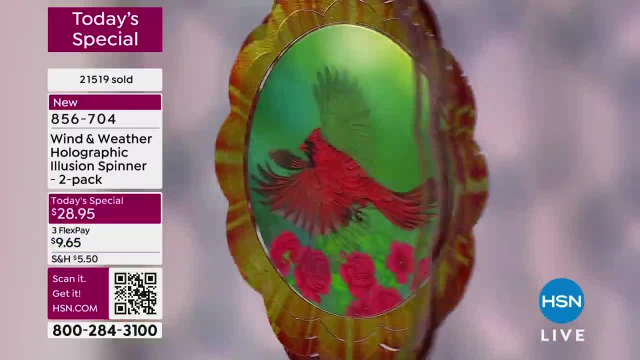 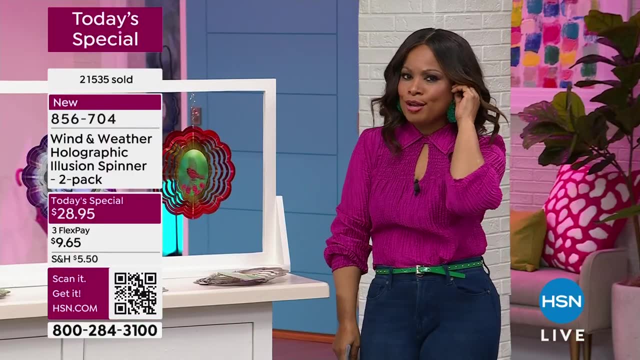 Cardinals. Well, we're going to leave it there. by the way, if you notice the shepherd's hook by Yvette, that is actually available. It is a separate purchase, but if it's something that you'd love to, oh, it's sold out. I apologize, Oh, nevermind, It was available. 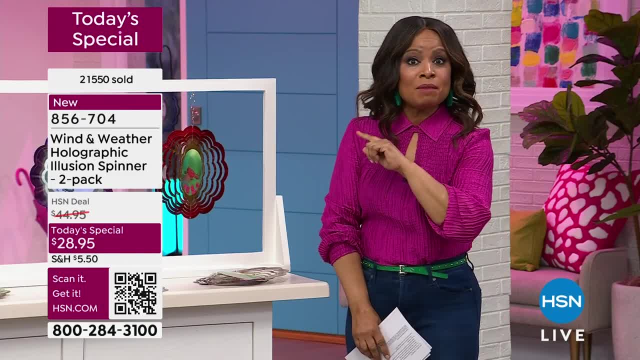 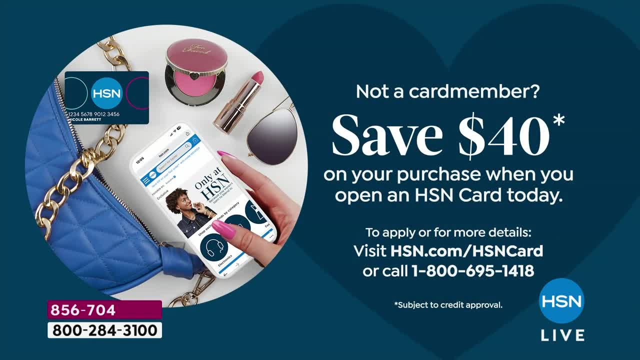 9 pm. That will be your final chance to shop with us for our today's special. If you want to have the best chance at getting that butterfly, you'll need to continue to call in, because there is just in the hundreds in the butterfly. So I don't want that one to sell out, especially if you'd love to. 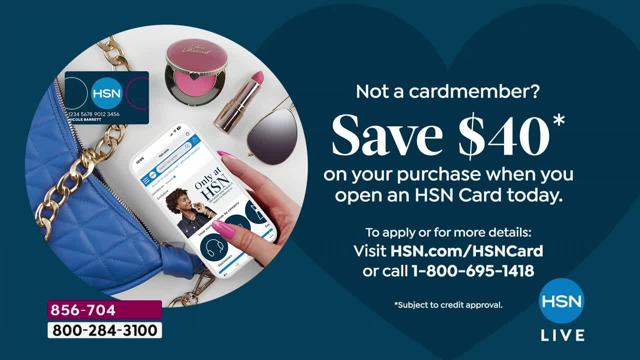 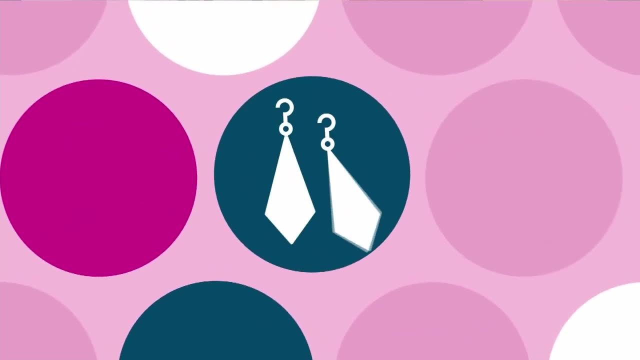 buy it. Hey, don't forget that if you're not an HSN card member yet, you can save $40 when you become a card member. Most people that apply are approved and it's easy. Give us a call at our toll-free 800 number or go onto the website at hsncom. It's finally Friday, Definitely one of our 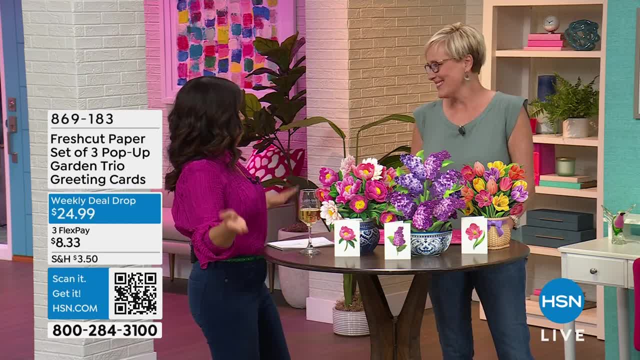 favorite days of the week And I hope that you're off for the weekend. I'll be here all weekend and I'm thrilled. It's fun here. It's not a bad place to be for the weekend. No, I'm looking forward to. 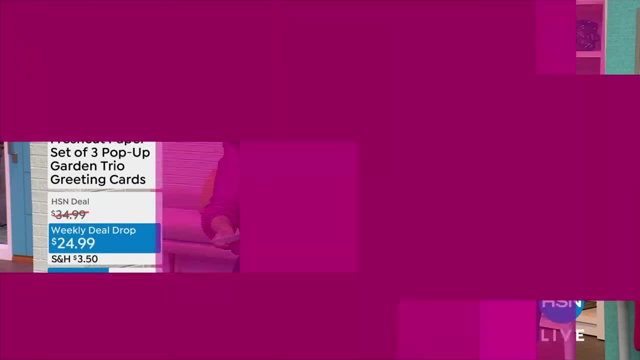 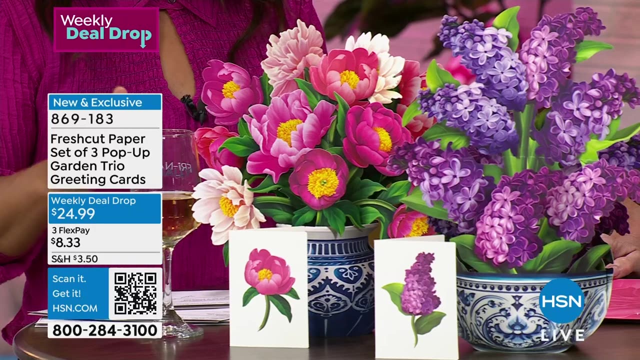 it. So this pretty lady happens to be our one and one of our crafters and you bring to us all sorts of great crafting products. But today Leslie Bracken is bringing to us our fresh cut paper, And these I so nicely into our today's special because you're not choosing everything that you see. 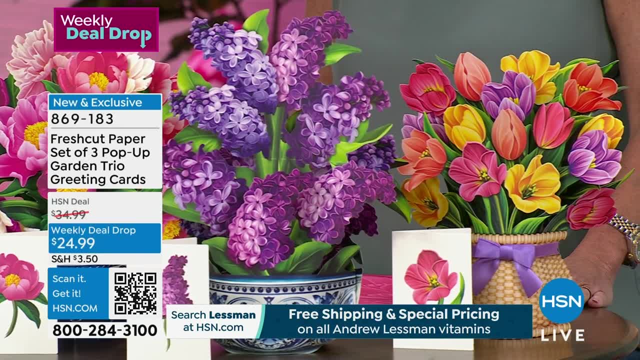 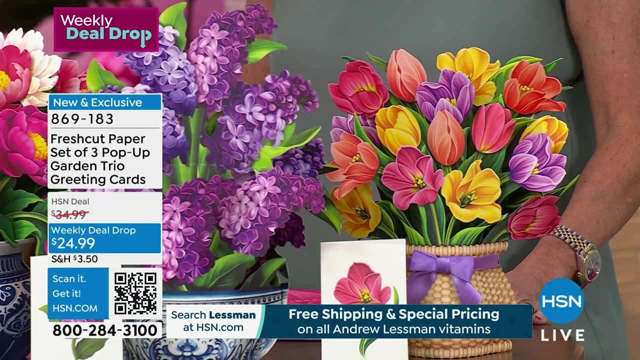 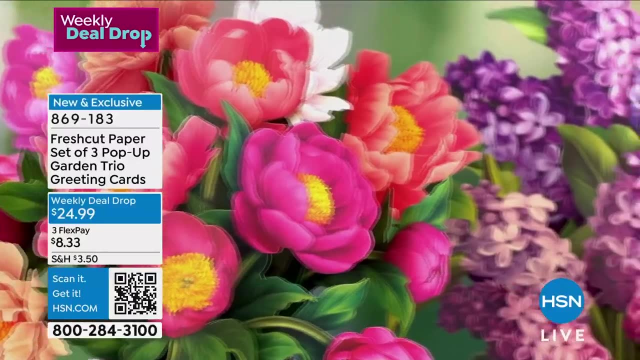 before you will be coming to your home as a weekly deal drop of $24.99.. So I checked online and Mother's Day is exactly one month away from today. Did you hear that? kids One month from today, And I think about all the mother-like figures that are in our lives, or it could be. 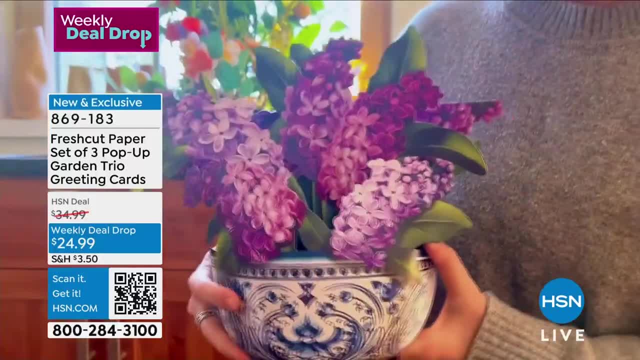 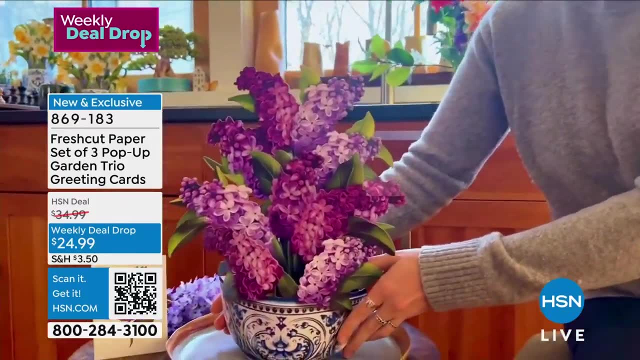 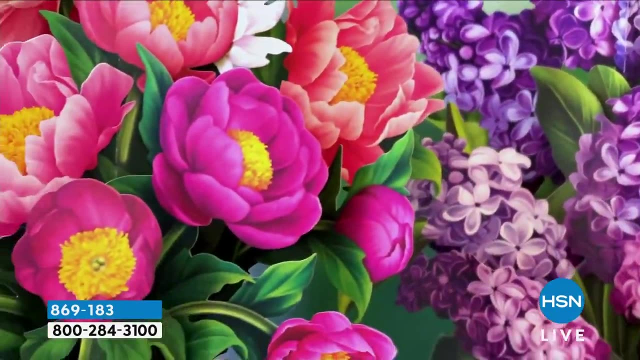 your daughter-in-law or your goddaughter or an aunt or relatives, but look at what you're getting. Oh my gosh, I love this child, All three. So talk to us, because this, this looks beautiful- floral bouquet. it's a pop-up bouquet And, by the way, so this is our brand new. 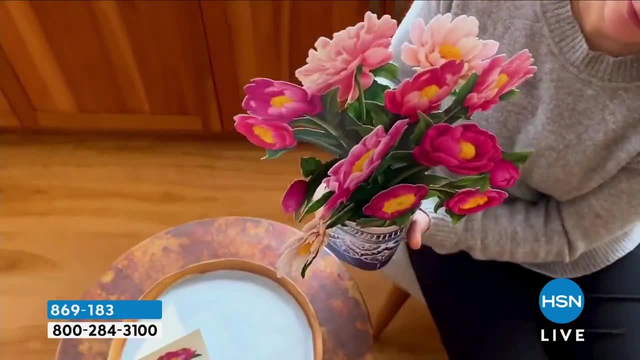 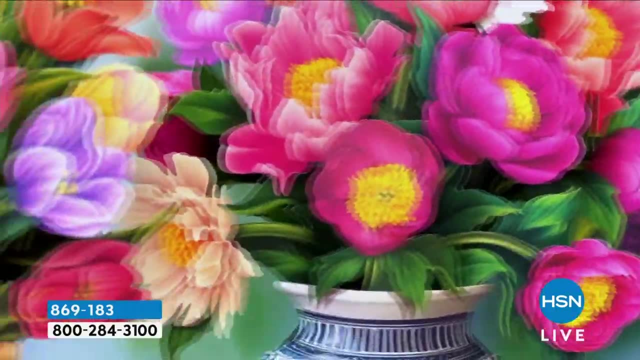 trio. We brought several trios here before and they are all. every single one of them are customer picks, almost total five-star reviews. every single one of them. And this is our new bundle We're bringing to you. You're getting all three of these. I cannot stress enough. All three of these are: 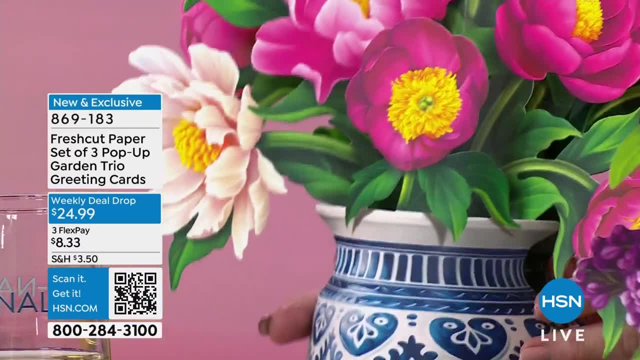 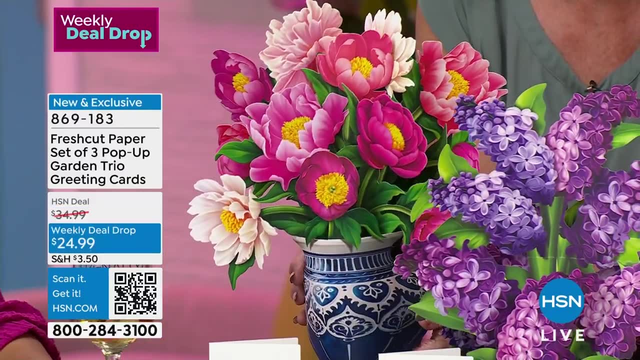 coming. you're getting these wonderful peonies that are in this incredible like french pottery looking pot. it's that indigo and look, i'm gonna tip. i mean, look at the depth. the flowers themselves look three-dimensional, but this arrangement actually is three-dimensional. you're getting 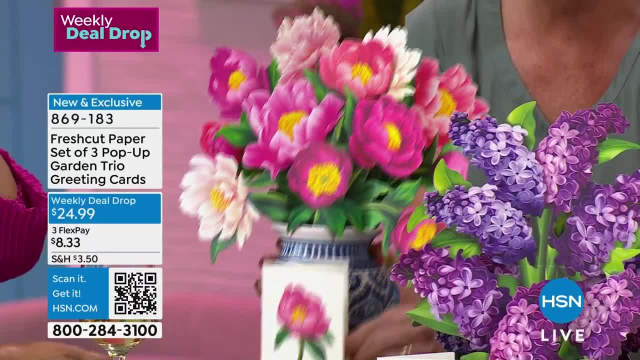 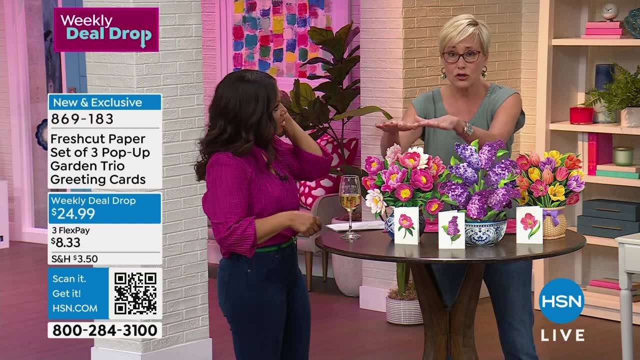 a pop-up bouquet with a blank note card that matches back to it, and it even comes in a fabulous envelope that matches back to it. you're also getting this, by the way, the peonies is like 13 inches tall and about 12 inches wide, so this is a substantial bouquet arrangement. we're also 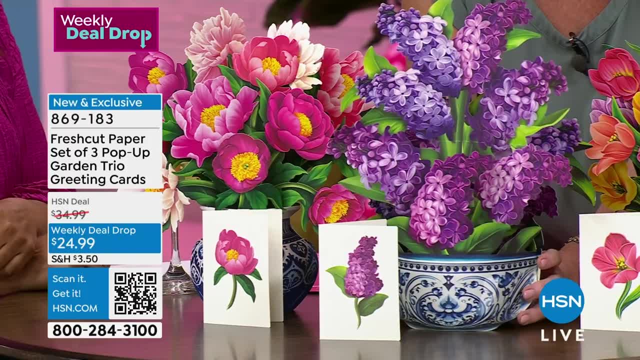 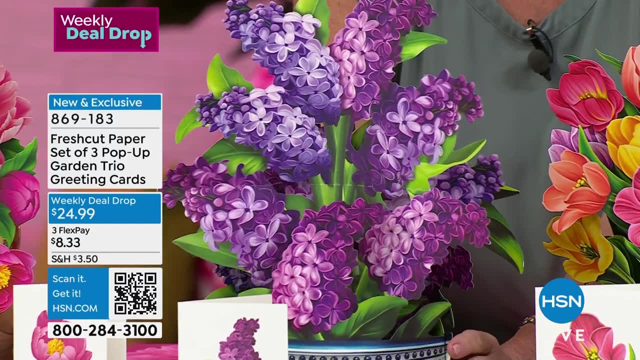 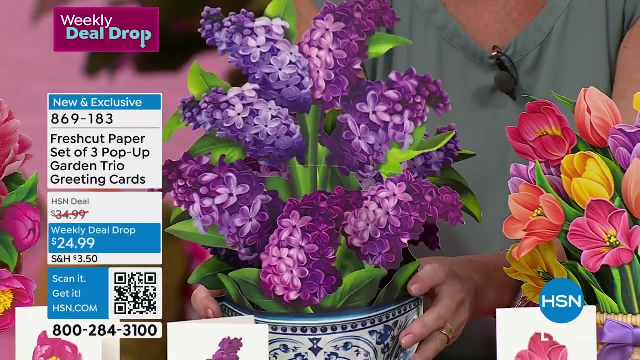 giving you these amazing lilacs- i mean, look at the purples in here right- and lilacs. they are beautiful, they have they're fleeting in the way time that they bloom, so they're not available very often. but they're also very, very fragrant, sometimes a little harsh. so this is giving you all the 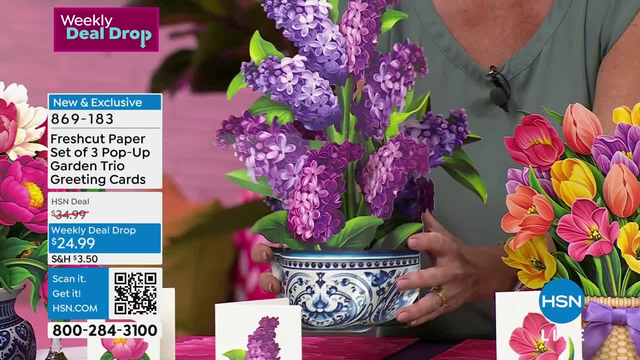 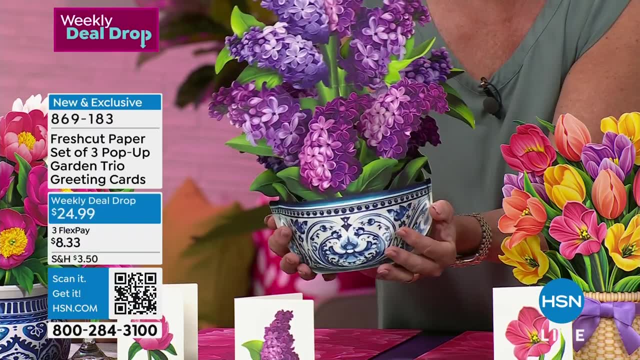 beauty, all the depth of color, all of the drama and spectacle of a lilac with the height- and this is 14 inches tall, so this one's really high- and this wonderful french again looking porcelain bowl that it's in but it will never. it will never die, it will never. 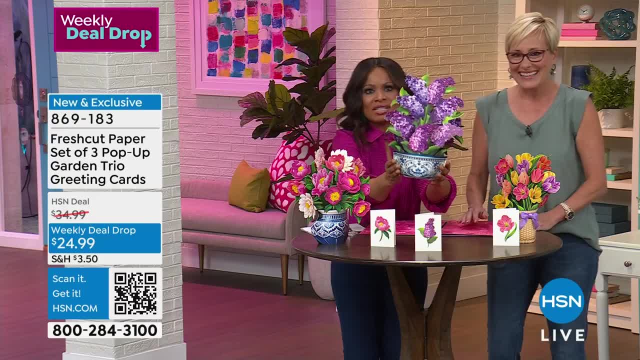 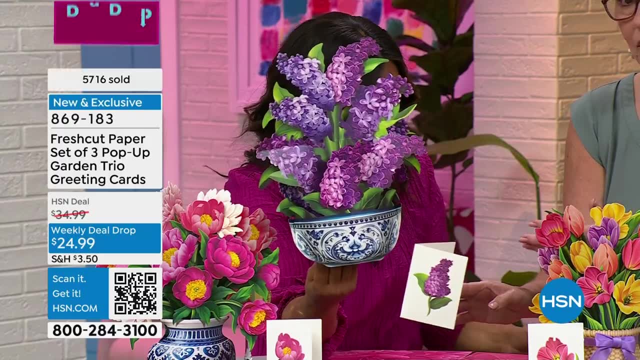 wilt, it will never be too strong. i mean, can you that alone? is that not gorgeous? and it also has again. each one of these has a blank note card. so we're talking about mother's day- it's coming around the corner, we're talking about that, but it's also teacher appreciation week is coming. 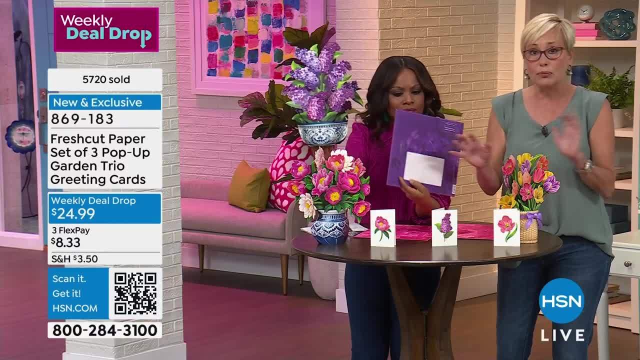 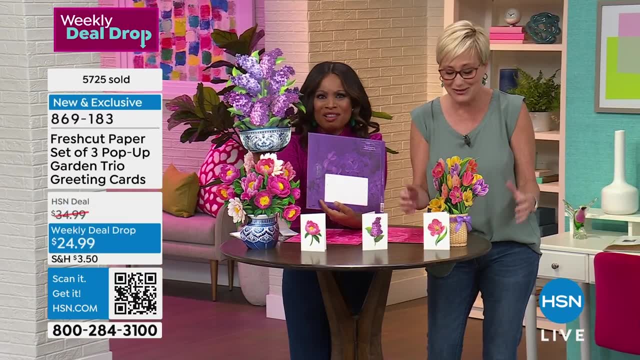 graduation season. think about. each one of these has their own personality and you're getting all three, so whether you're keeping them for yourselves- and i know from the reviews that a lot of you are doing that- because when you get them there, you just can't believe how spectacular they are- 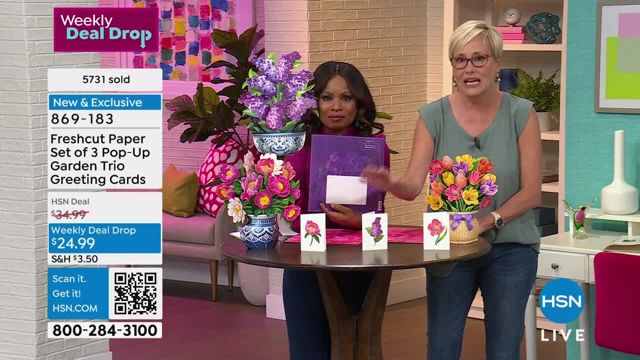 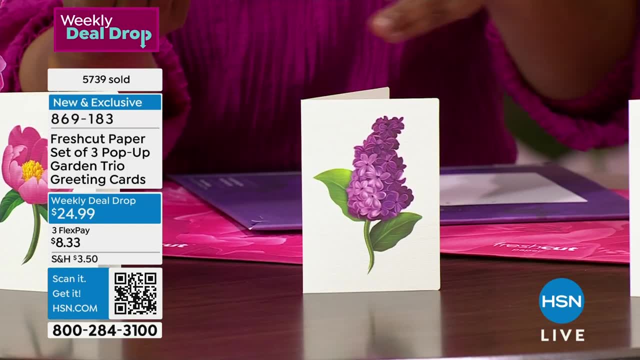 or whether you're giving them away. it's going to be received any time of year for any kind of sentiment, because you're getting the blank note cards. and when are flowers not appropriate? no, they're always appropriate and flowers. we love our live flowers, but they can be very expensive, as we 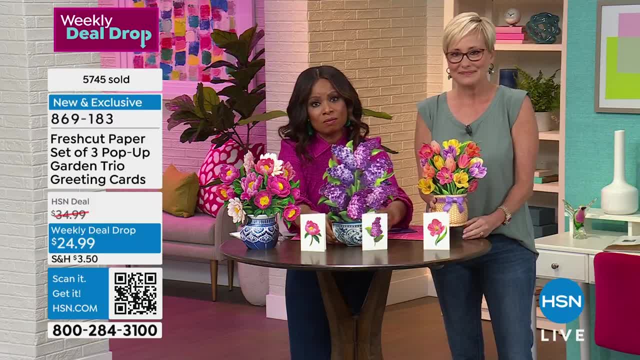 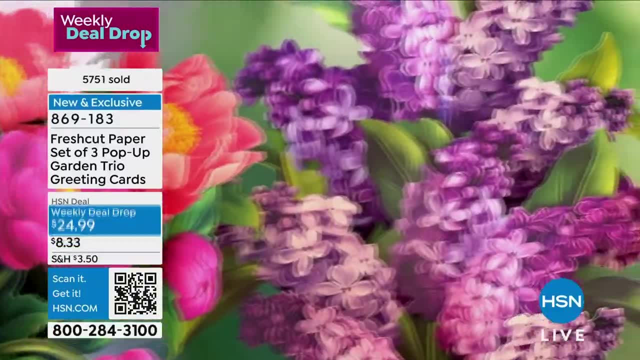 know, and we do know that after a week or so they do start to wilt and they start to die and you do have to give them a little maintenance. with these they're perfect and they'll last and last and last and last- over 5700 of them. 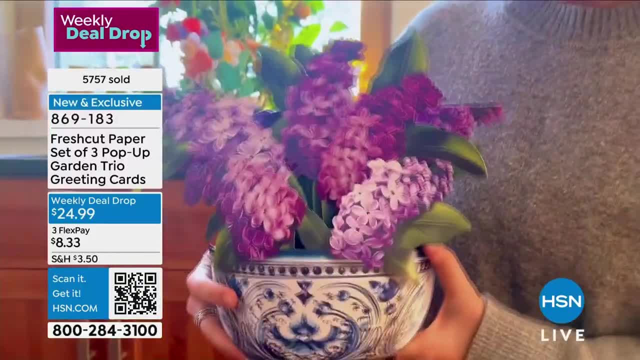 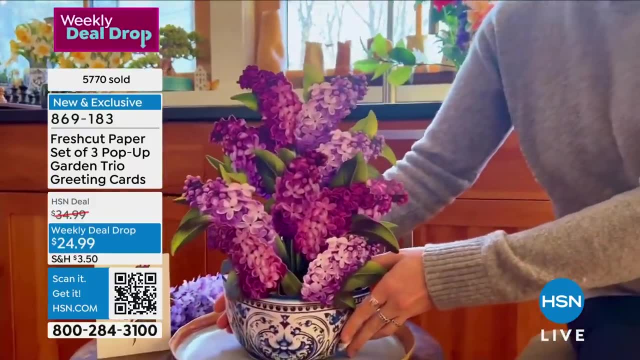 are gone. absolutely. you'll be able to put this directly in the mail and mail this to whomever you'd love. i would not wait. you're looking at 25 off of our price. that weekly deal drop will not last. i've had the great pleasure of working with you, leslie, and bringing many varieties. they just 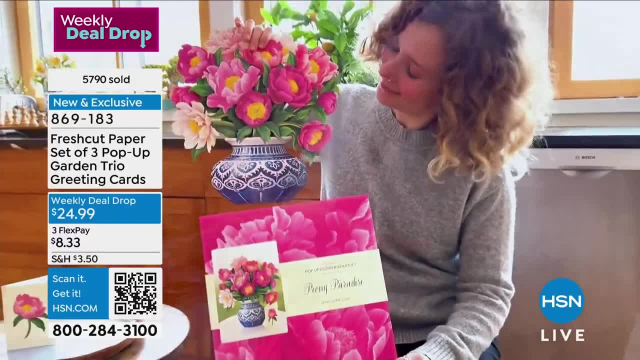 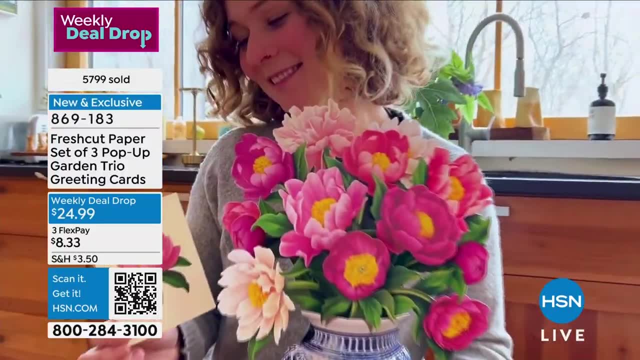 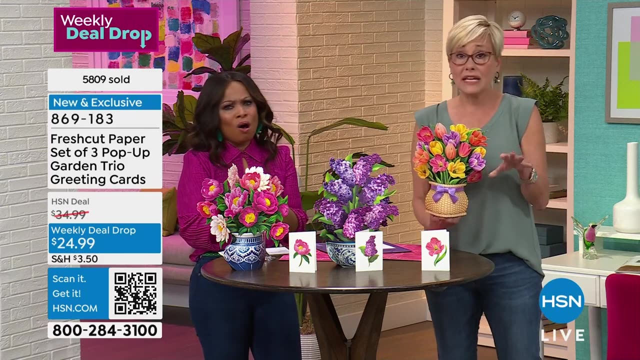 keep getting more beautiful. right, they are incredible, i will say this. as beautiful as they appear to be on tv, when you get them in person, oh my goodness, imagine someone that might be in an assisted living facility where they can't get fresh flowers. so many of these assisted living. if you're in critical care, if you have someone in, 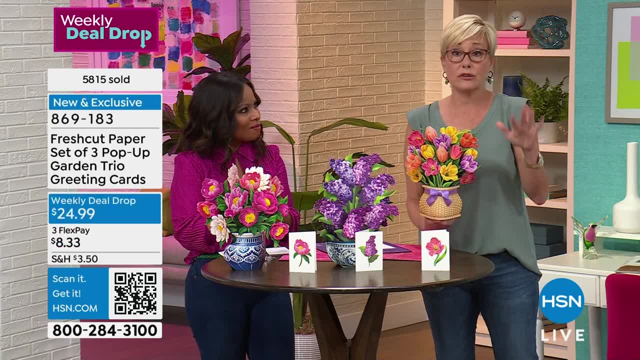 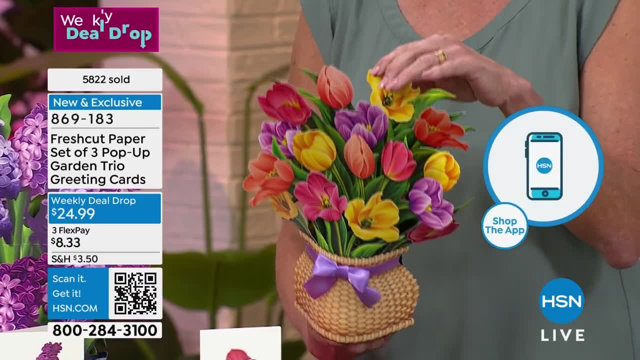 critical care or assisted living facilities. a lot of them- critical care units- will not accept fresh flowers. a lot of the of the assisted living facilities don't like them because they have residents with allergy issues. so this can go to anywhere you can get them and you can get them. 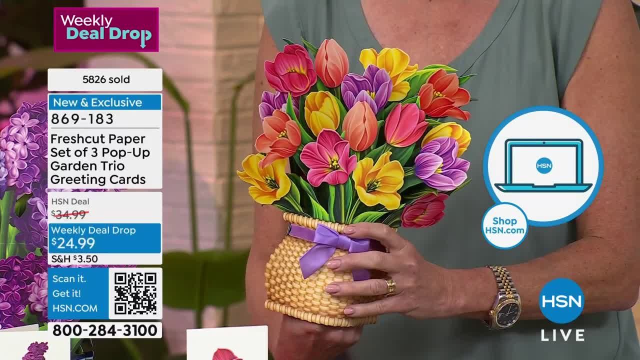 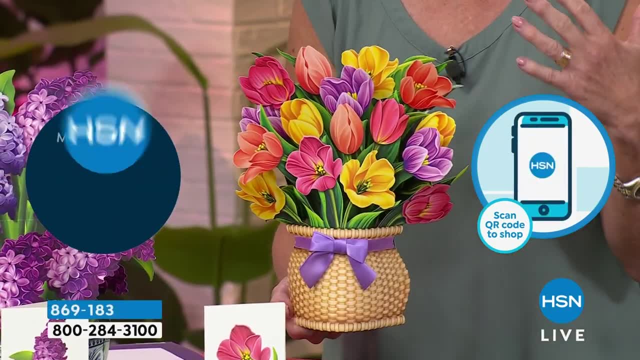 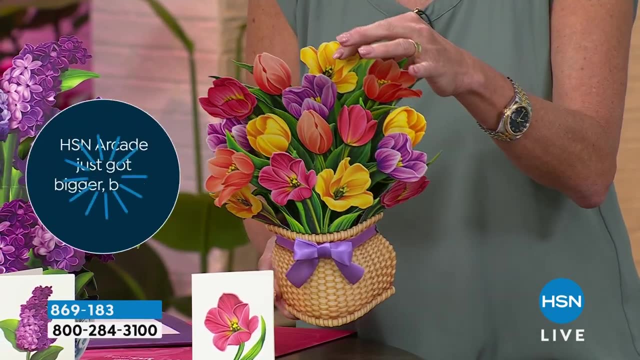 anywhere, and it's giving you all the glory and loveliness of fresh cut flowers, but with none of the hassle, none of the pollen, none of the stinky water, none of the expense, because by the you're getting this beautiful and this is the, the tulips which i love, this is the essence of spring, right. 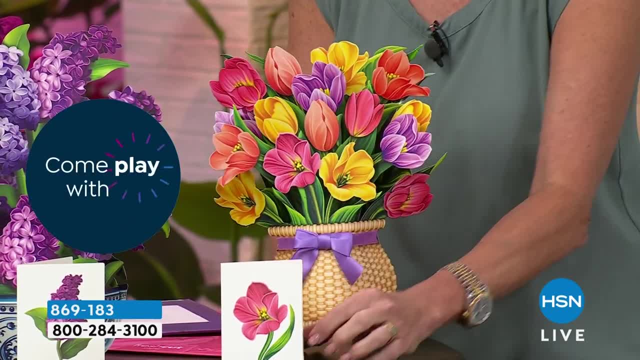 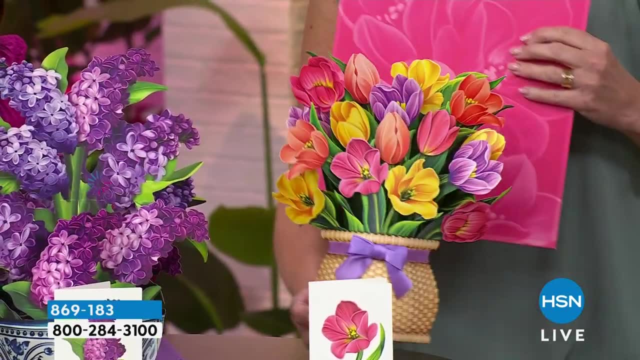 here, but you're getting the beautiful pop-up bouquet with, again, the blank note card that matches back. so this is anyone, anywhere, any sentiment, the big envelope that it comes back, that matches back to it as well. that's an art piece in itself. this does take four forever. 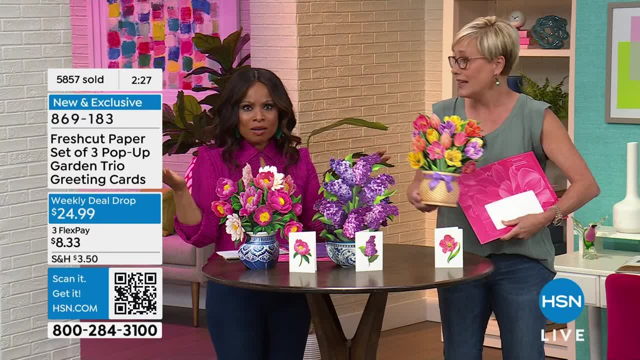 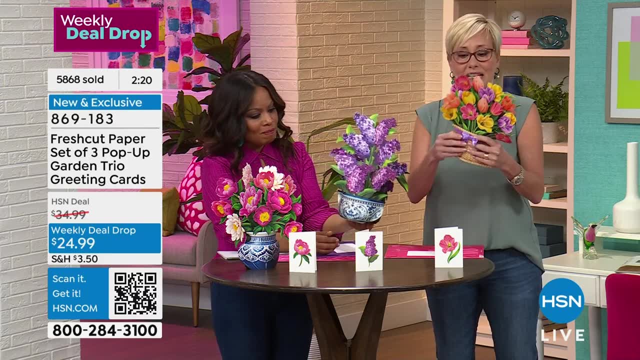 stamps. this is, this is postage you have in your drawer, so you're not schlepping to the post office and putting things in a box, and if you're keeping this for yourself or for whoever gets it, it's, it's folding flat, right, so it's coming to them flat, just like this. the, the, these, um, wonderful tulips. 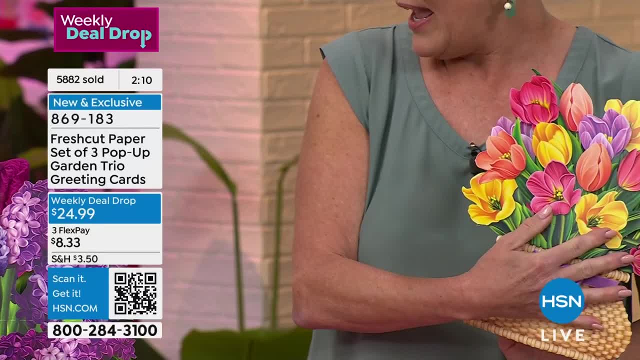 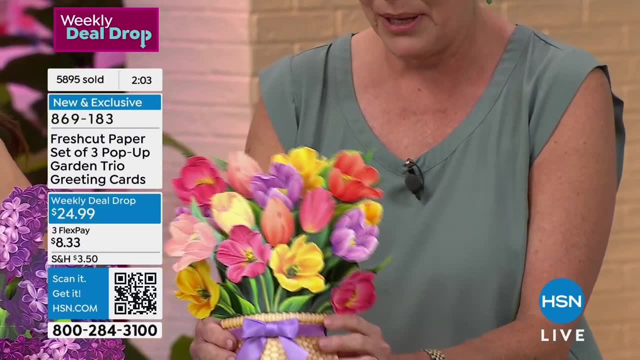 are seasonal, so i would love to like put them away and bring them back out in the season when it's springtime, and you can do that because they fold flat and it's this great little pop-up that makes it stand straight. use them year after year after year. 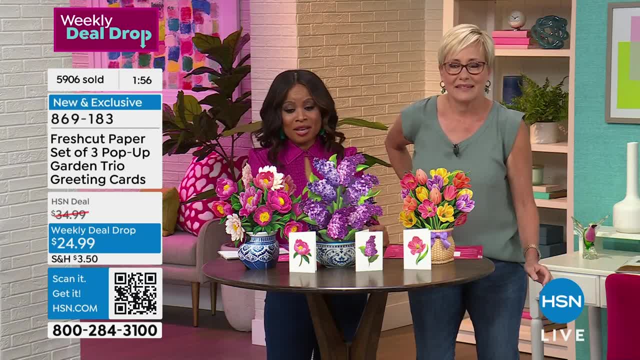 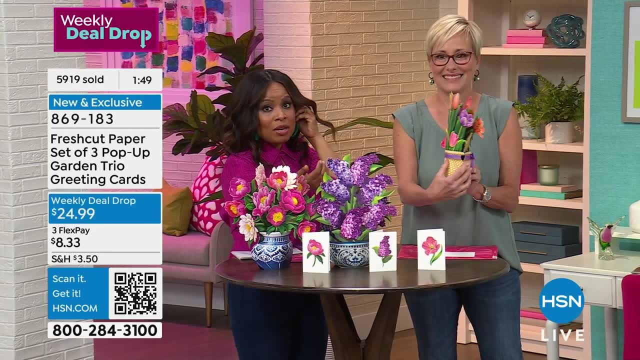 if you just chewed again, remember you're getting everything that you're seeing here, so it's not that you're choosing. and listen, we- we all- have purchased cards- holiday cards or birthday cards- and we know how expensive they can be and i'm sorry, i'm busting. very expensive, i'm working. 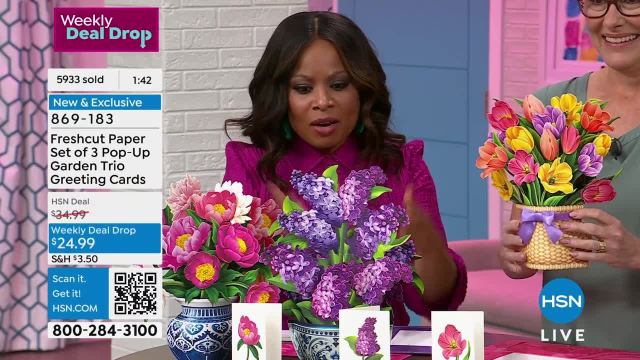 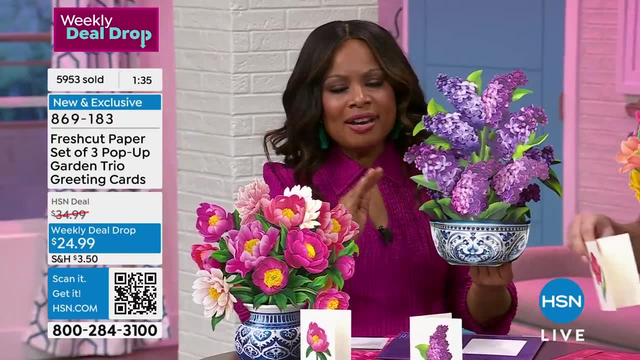 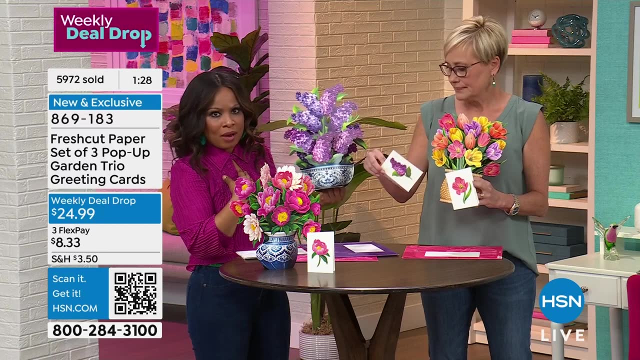 with a new one tonight, so this one isn't my normal one, but they can be very expensive and we've all done it. i know i've paid eight dollars for a card before nine dollars for a car and paled in comparison to something like this, and even the note cards will take your breath away. 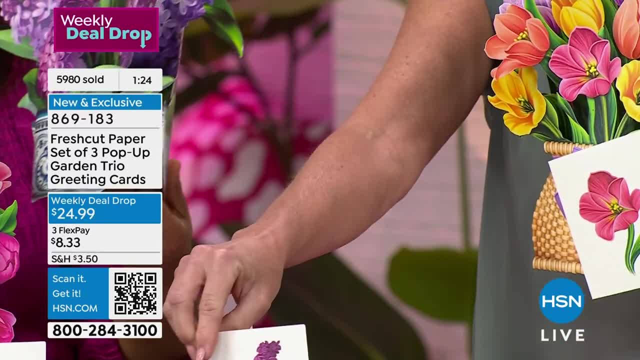 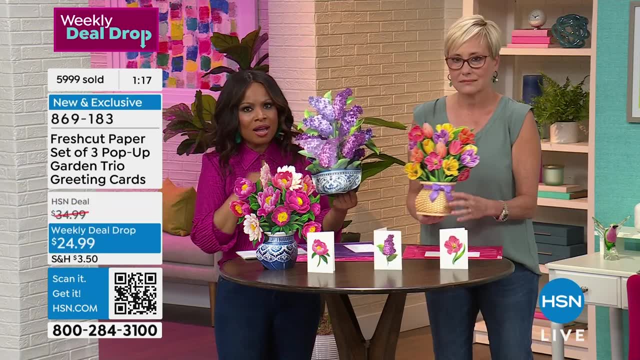 because they are so beautiful and stunning, and i love that you're getting all three: maybe one for a teacher, one for someone that might be going through a little tough time, one for a great neighbor that did something really lovely and thoughtful for you. you have these available, they. 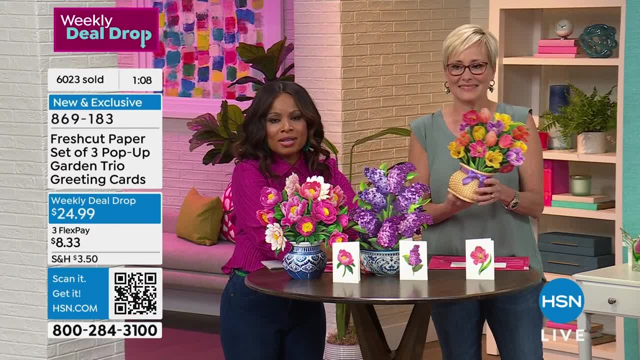 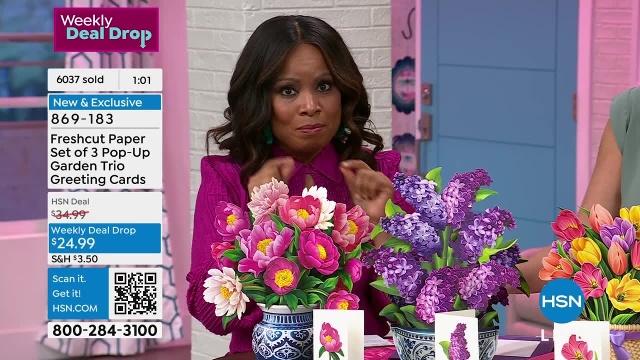 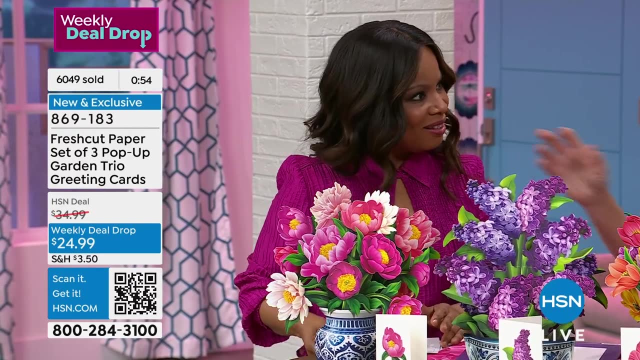 are at the best price that we've ever offered. that's why we call them a weekly deal. drop you off, and a lot of you jumped in on this. don't forget, mother's day is exactly one month away from today. perfect mother's day, perfect mother's day. perfect teacher appreciation- great like so. 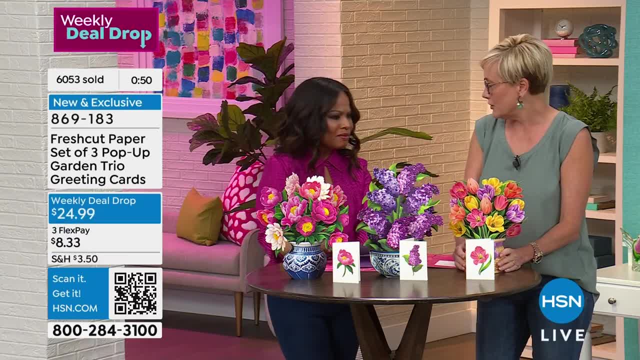 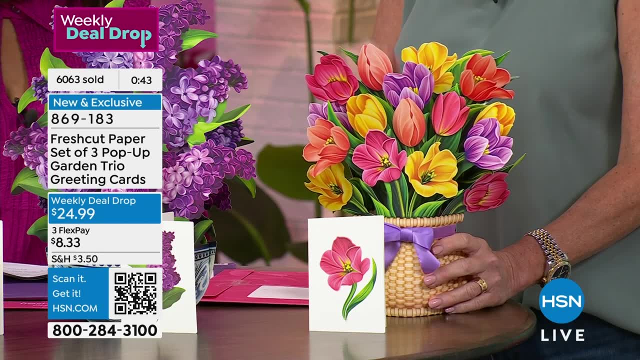 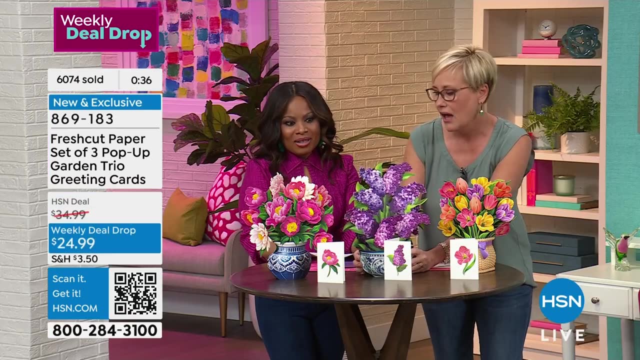 the. the tulips actually symbolize unconditional love and new beginnings, so i actually gave these to in a wedding shower and a baby shower this past week because it's the perfect for new beginnings and unconditional love. oh, it's a standout. are acceptance, um, their, that's what they resemble. so do you know someone that's going through something that needs that? 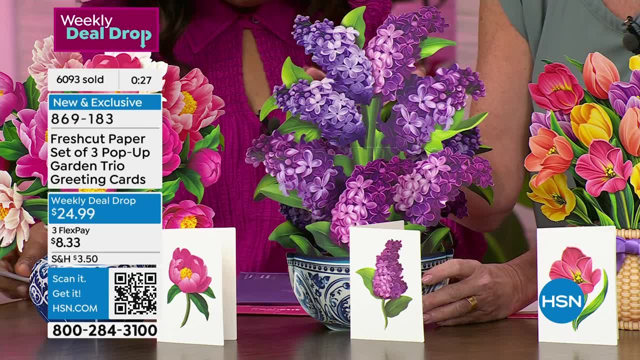 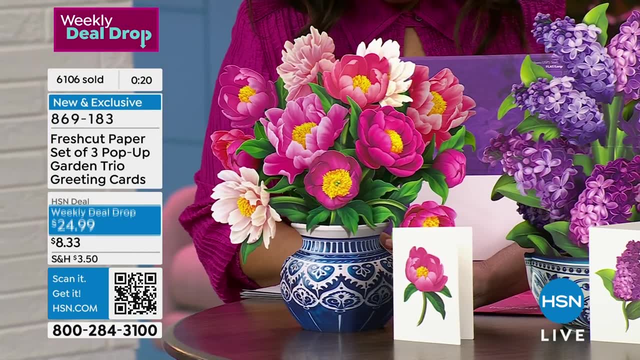 little boost of confidence, and they have the drama of the purples to go with it. this is the perfect arrangement for them. and then these incredible, vibrant, i mean just they look like fluffy, they're so thick and rich. these blooms, the the art on them is so amazing, as well as. 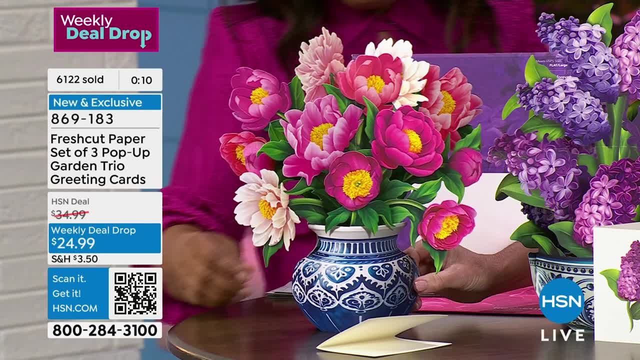 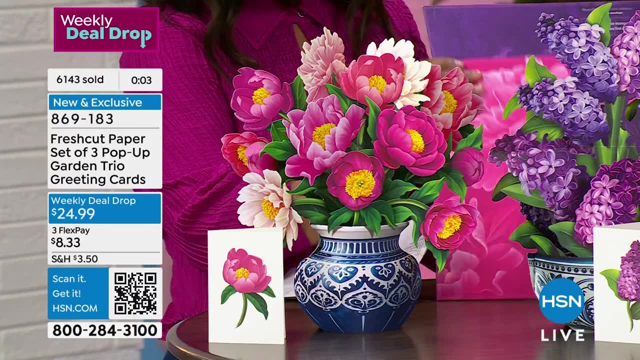 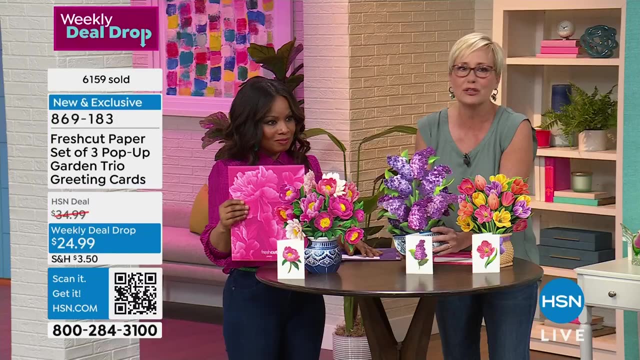 them being three-dimensional and 360 degrees and they, they are absolutely kind of bounce right out at you. you're getting these blank note cards. so again, it's any occasion for anyone, they match back and really for the price of a card you're getting a gift, an art item, everything and believe me, look at the reviews of our past product- all. 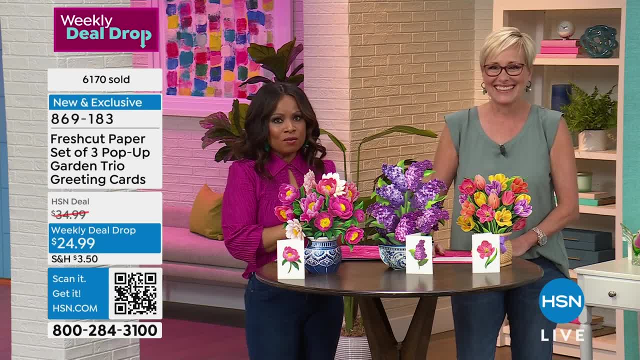 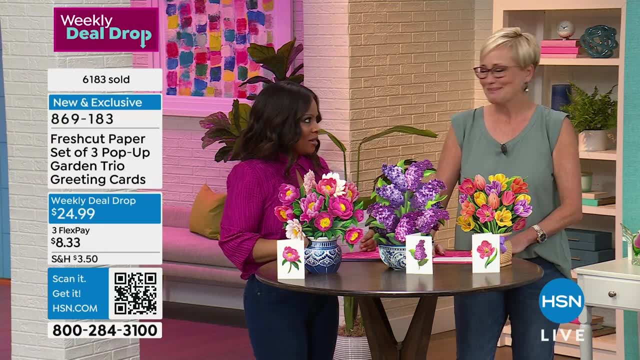 right, everyone, they don't last. and here's your shot. if you'd like to order, let us know. we'll be happy to get them out to you. the price goes up on sunday, so please order as quickly as possible. leslie, always great to have you here. always great to be here. all right, we, in fact, are going to be. 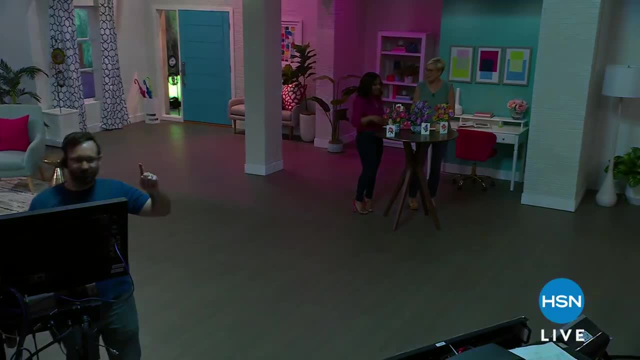 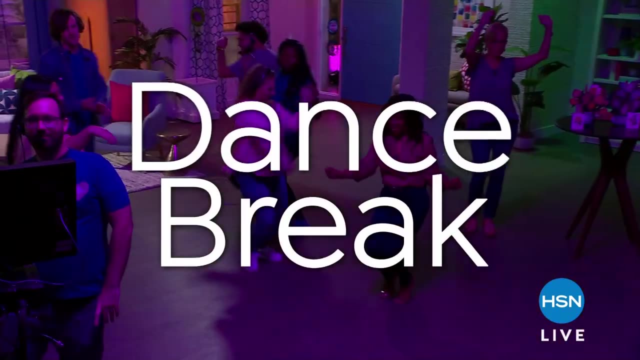 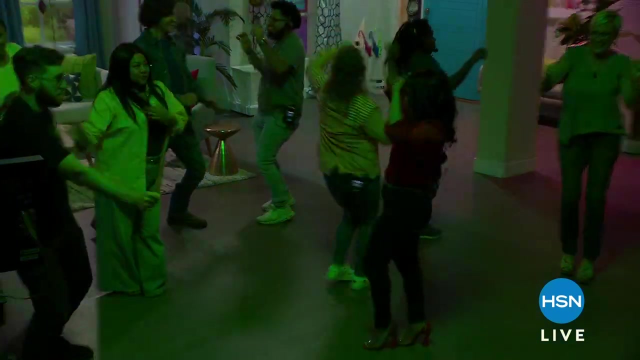 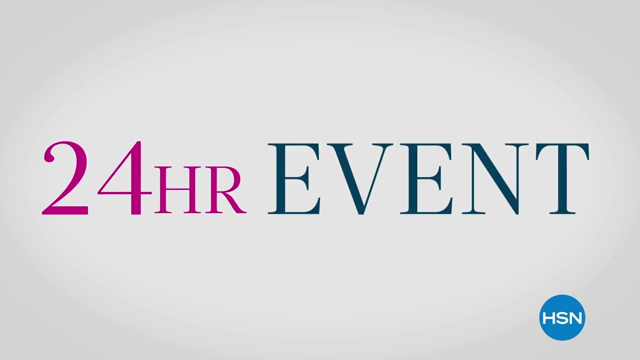 heading over. even more fun during a break, right? oh, it looks like we're gonna do a little, i think. well, attention, all crafters. get ready for an exclusive 24-hour event just for you. it's hsn's crafters appreciation sale- from scrapbooking to paper crafting and even home decor, and it's all on sale. 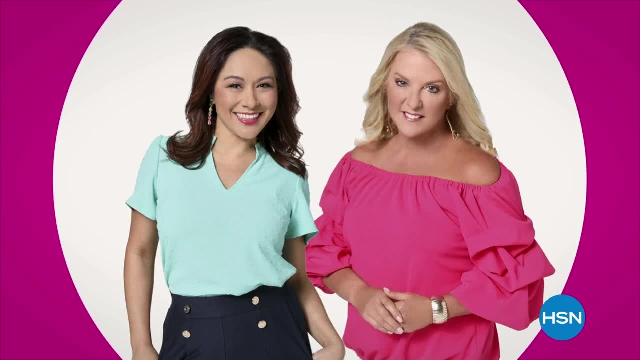 plus, join hsn so we can keep you entertained and go out something extra Sciences: everyone hope this was fun and clear value. keep spinning goes to everyone with it. heinz, you make some good work. we'll be back here next time. thank you now craftinistas, tina and suzanne, for the premiere of up close and crafting: live our first ever. 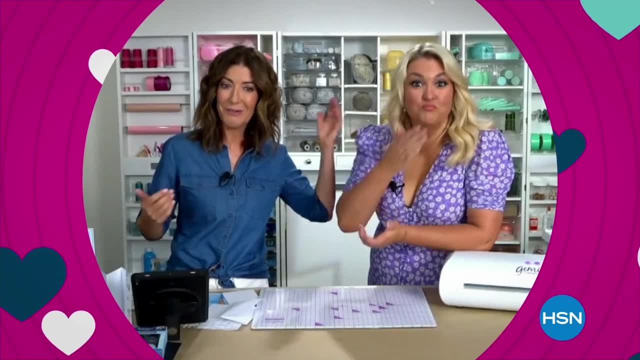 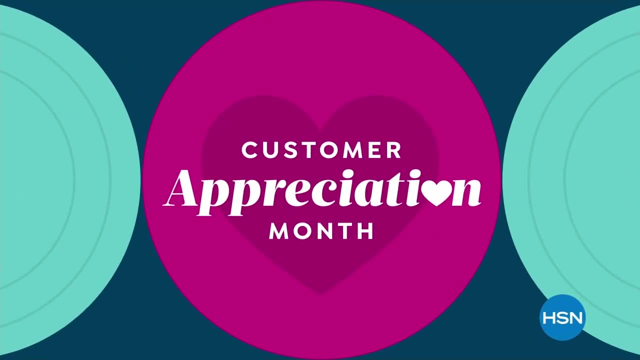 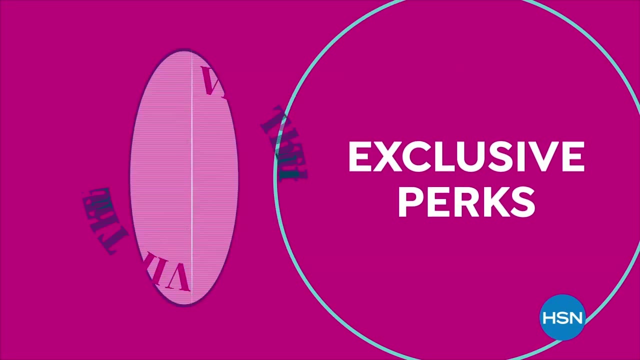 hands-on crafting event with your favorite crafting experts and lovers like you. it's a 24-hour crafting extravaganza only on hsn. it's customer appreciation month and it's all about you for the entire month of april. we're showing the love to our hsn card vips with exclusive perks, like vip. 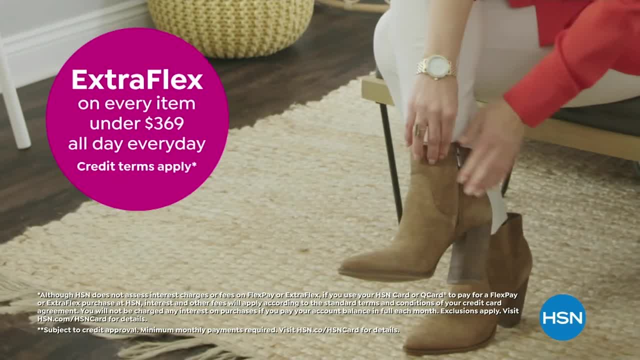 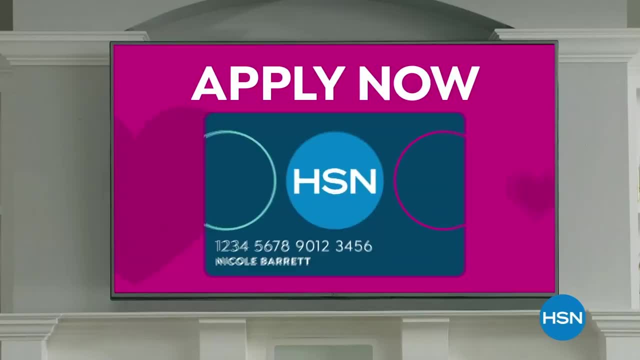 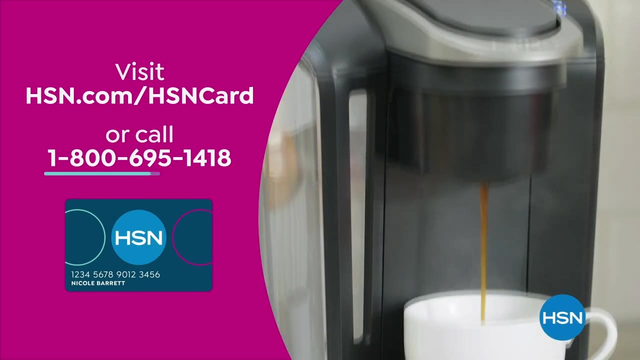 thursdays: get a special offer every thursday in april, plus extra flex on every item under 369 all day, every day, or vip financing on so many items. not a card member. apply now and instantly get 40 off. when you're approved, visit hsncom, slash hsn card or call 1-800-695-1418 for details. 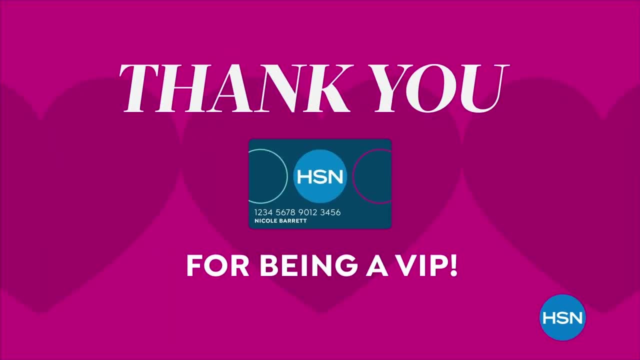 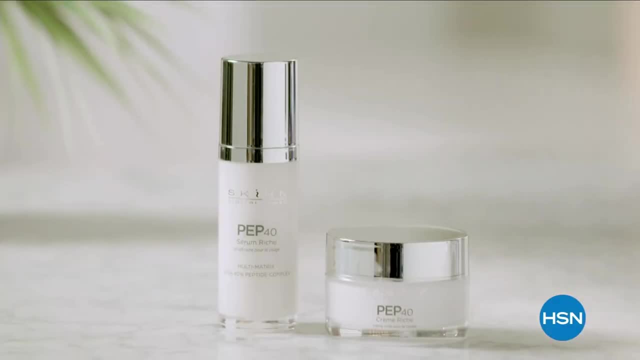 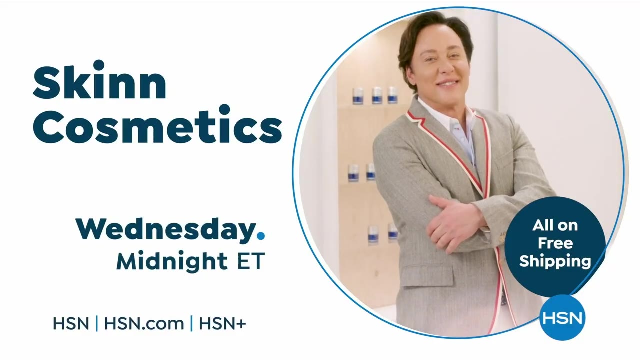 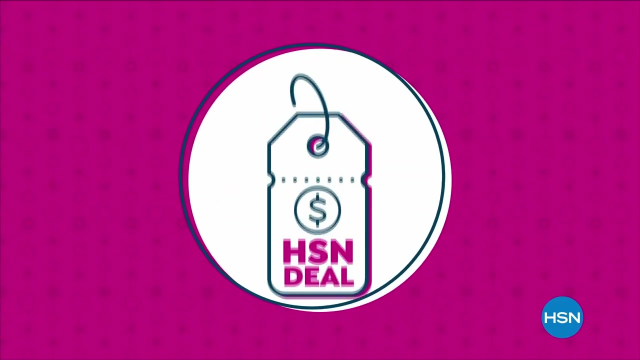 on our exclusive vip offers. thank you for being an hsn card vip. we understand every woman's skin is unique. we offer you beauty solutions empowering women to achieve healthy, radiant looking skin. genuine beauty begins with skin. the hsn deal is a great value that we bring to you every day thanks to our 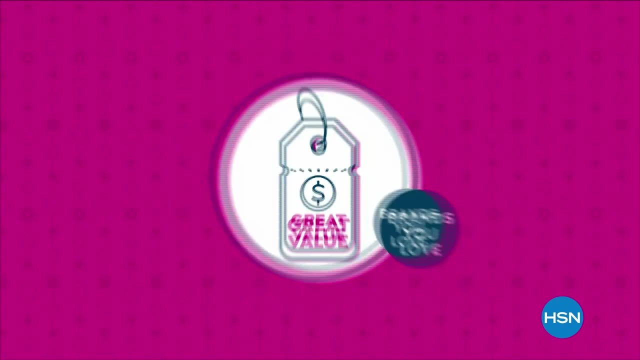 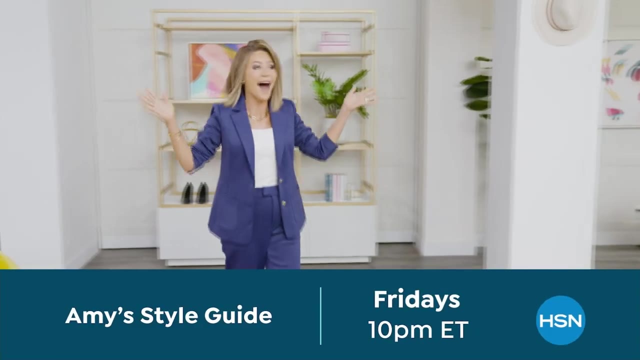 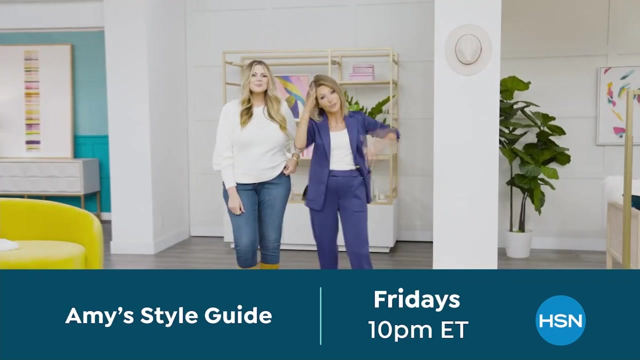 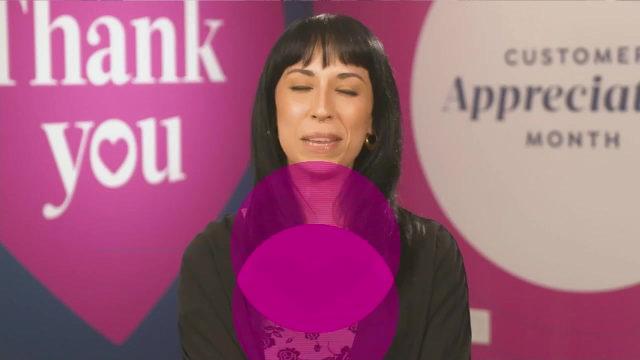 long and valued partnerships with the brands you love most. we are able to offer amazing products at great values. shop the hsn deal with confidence from us to you. finally, there's an entire evening dedicated to indulging in everything- fabulous. hi, my name is gg laige and i am an on-air assistant producer here at hsn. we actually 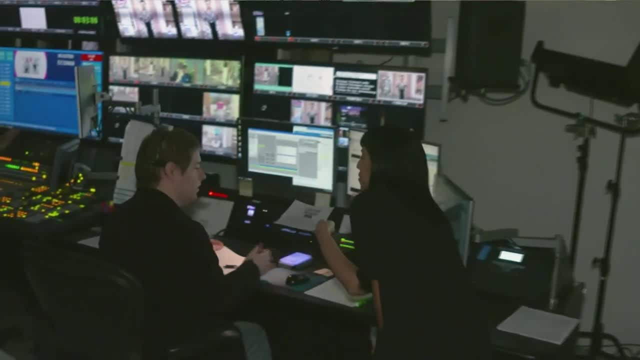 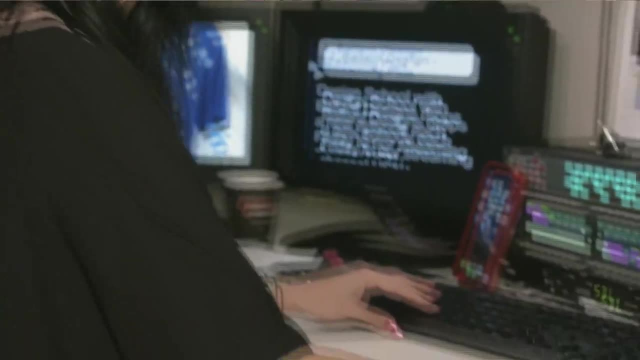 spend a lot of time in the studios running around, but you can also find us in the control room taking testimonial calls from our customers or on the facebook live chat answering questions and responding to comments. we are also sometimes behind the photos and the videos that you're going to see in the future. 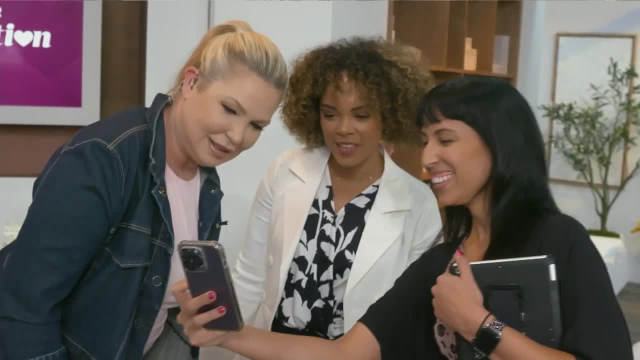 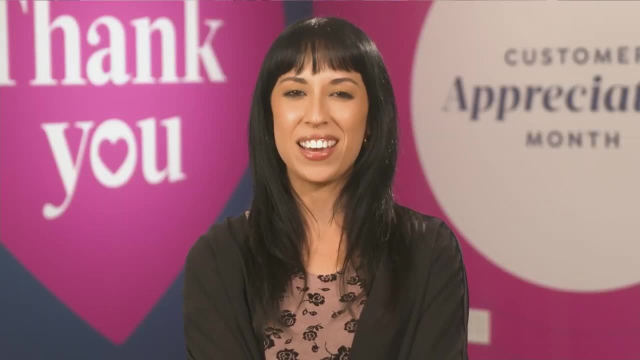 Friday night you can buy some of our products here at Jose and Lybe. fans are also a great means of sharing what you see from your favorite hsn host social media accounts. that's actually the favorite part of my day is when I get to share all the fun and connect with the customers. i love to make behind the scenes magic, to share the fun and 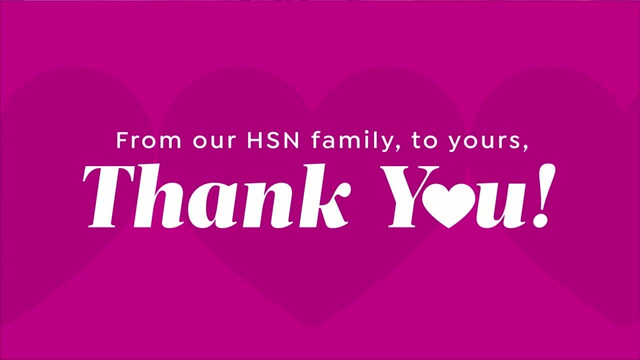 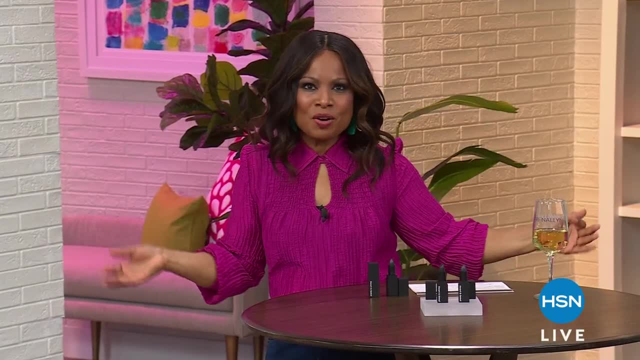 connect with all of you. thank you for being an hsn customer. I love that from mrs Gigi. hi everybody, it's so good to have you shopping with us. it's finally friday, and so this is the show where we kind of let loose a little. bit and have fun and relax on a friday night. we've got some great gems away, but also we have my next set of items, so we probably at, at the end of the day, a nice treat. so give your customers a larry and have a thankful itули and romantic love and stay late till you and us have a great night. 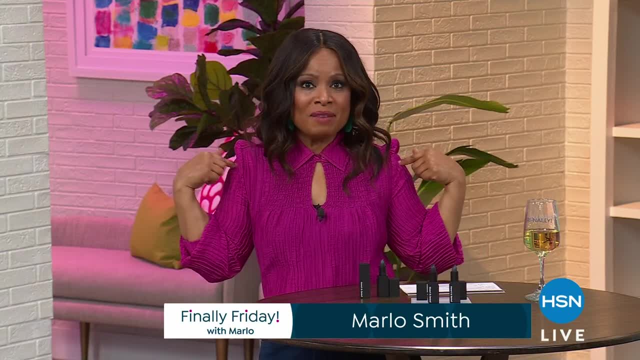 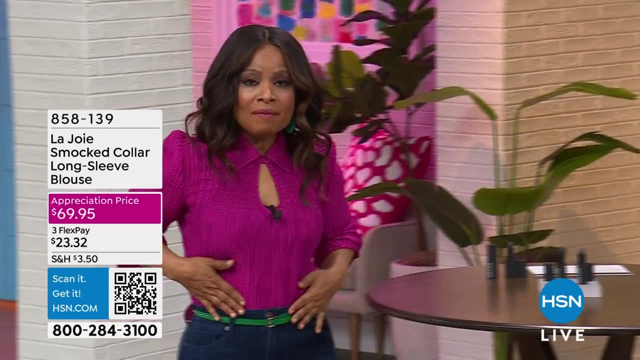 night. we've got some great products that we're going to be showcasing for you. but first i've got to tell you a little bit about the le joie top that i'm wearing. so it's new to hsn here. i'll show it to you. i have it tucked in, but it's really, really cute. it has a little snap here at the top. 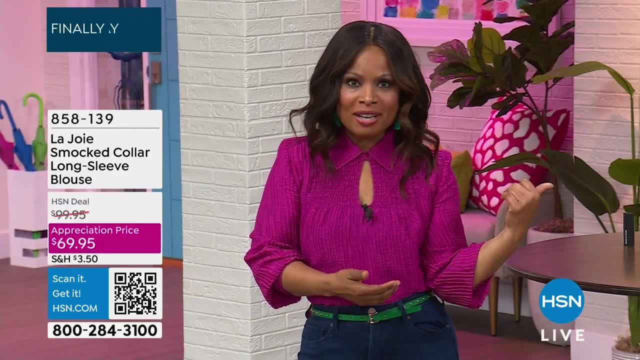 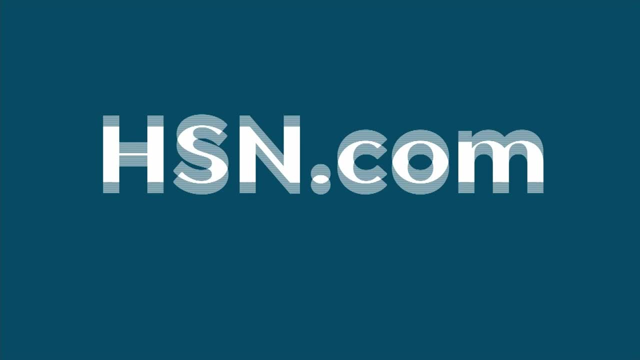 and if you love what the hosts are wearing, you can always head over to our website hsncom and shop the host closet. oftentimes you guys will email us on social media and go, hey, i like that blouse or i like the dress you were wearing, whose is it? so we found a remedy: there's our host closet. 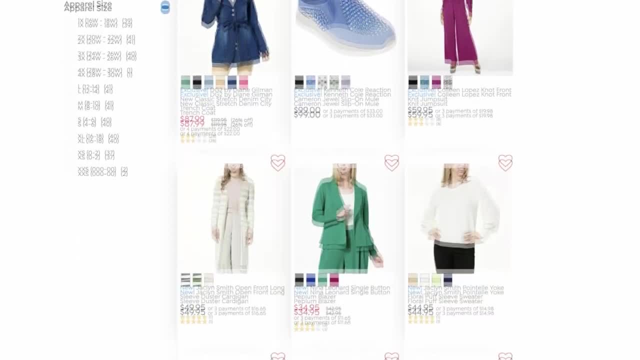 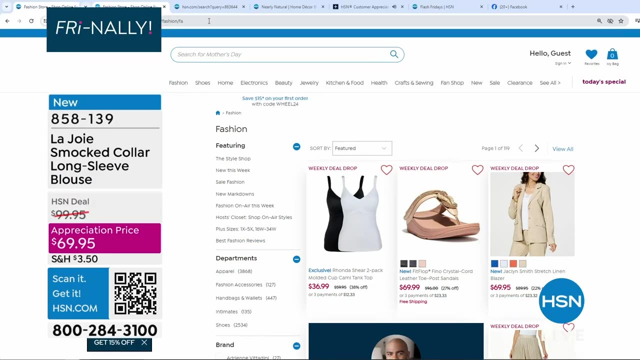 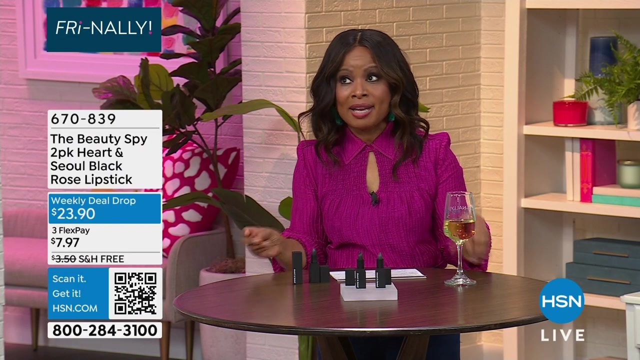 if you like the top that i'm wearing. it's by le joie, i'm wearing it in the festival pink and you certainly can go online to learn a little bit more. let's talk about heart and soul. have you guys seen this? and if you have not, this is incredible. super hydrating, incredibly moisturizing. has sold out. 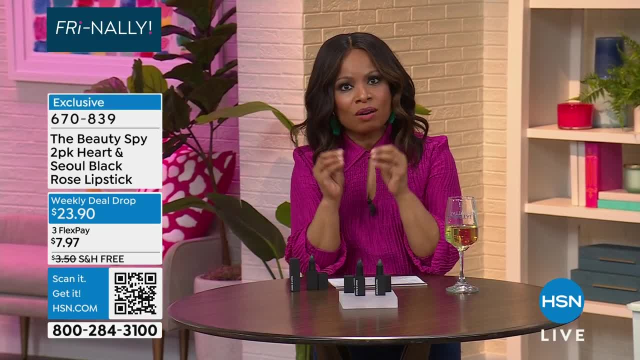 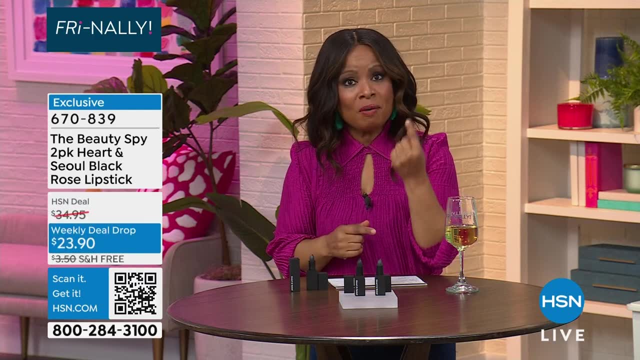 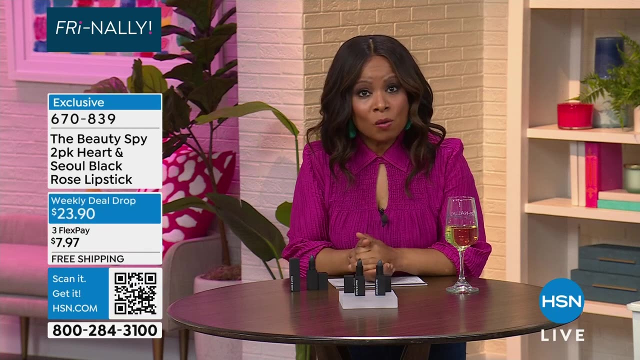 three years in a row. it's made from this rare black rose and and we actually have it here tonight. it's a bogo, it's a buy one, get one. one tube of this lipstick sells for 24. we get to offer to you two tubes for that price, only while supplies last and i. 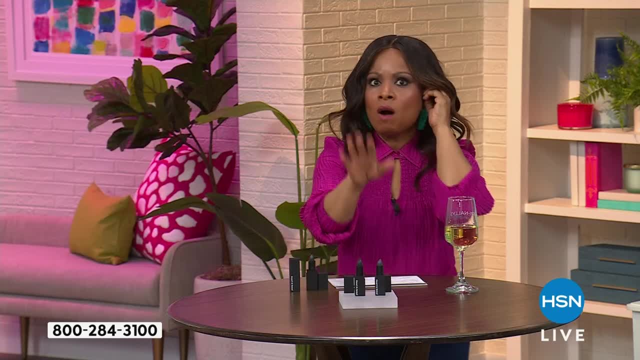 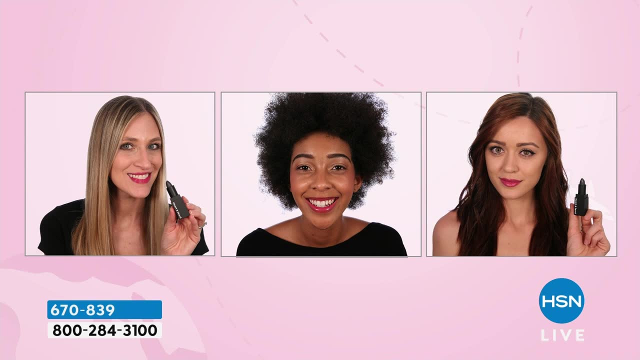 understand. we only have enough for tonight's show. now, when you first look at it, you're gonna go wait a minute. that lipstick looks black. well, you hold on just a moment, because this has such magic in it that it actually is going to work with your own skin's chemistry. 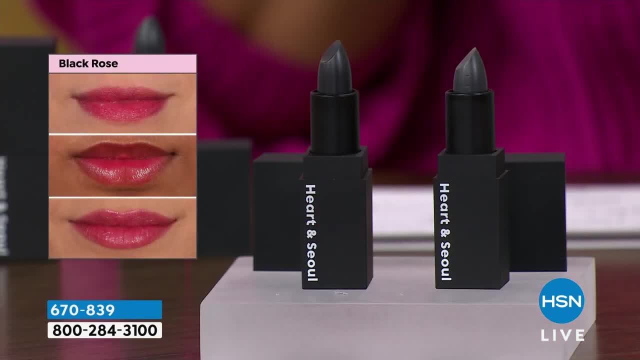 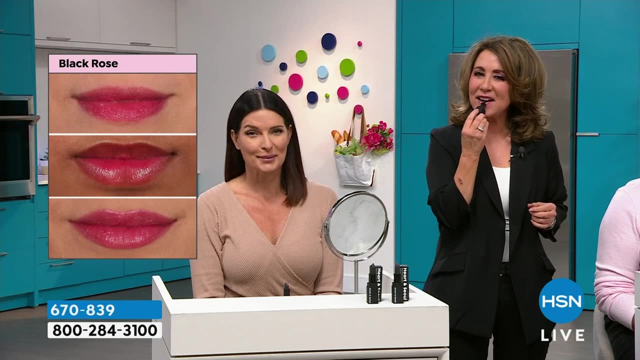 and your skin's skin and it's going to work with your own skin's chemistry and your skin's pH to give you the perfect berry color, no matter your skin tone. i want you to meet our beauty spy herself. her name is chelsea scott. she travels all over the world. she is a beauty expert, has been in. 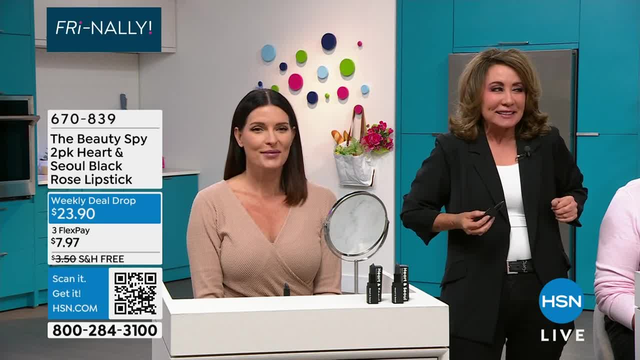 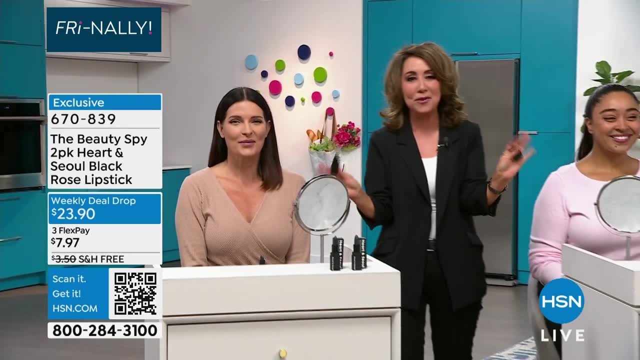 beauty business for more than 25 years. girlfriend, i'm gonna say that i'm coming over next to you. girl, please do, because first of all, may i just say i'd like to be invited to every one of marlo's friday night shows. what you really said? i came in and i said. you said: is that wine? i said: is that? 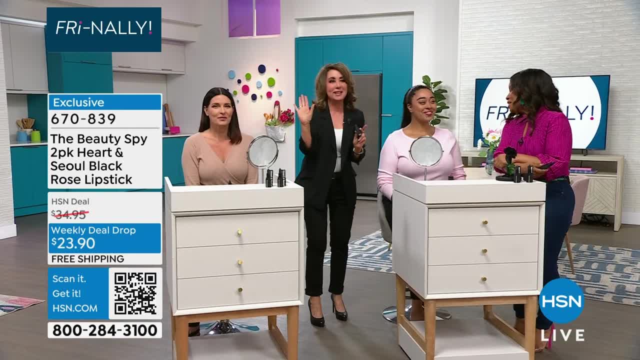 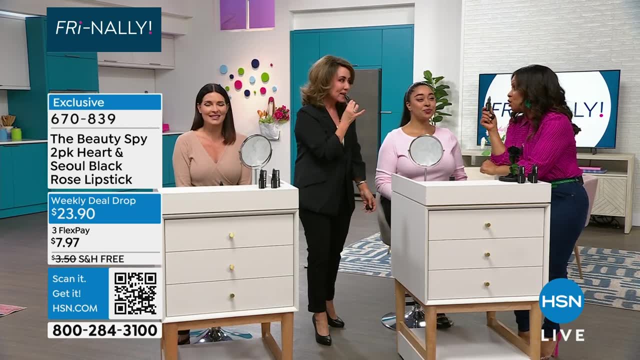 wine. is there a dance party? i'm in, she said she does. she's like wine dance. i'm here every friday show is given. i mean i love it. well, listen, let me just brag a little bit about you. two million, two million tubes of lipsticks by 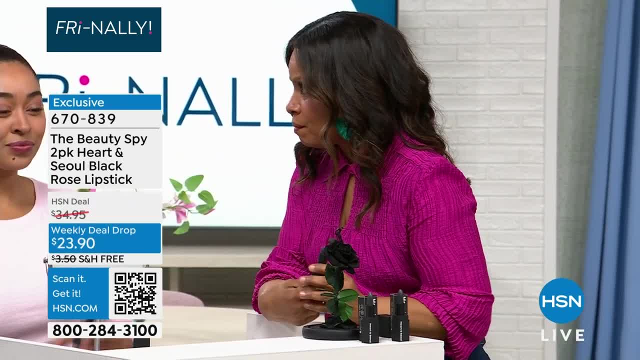 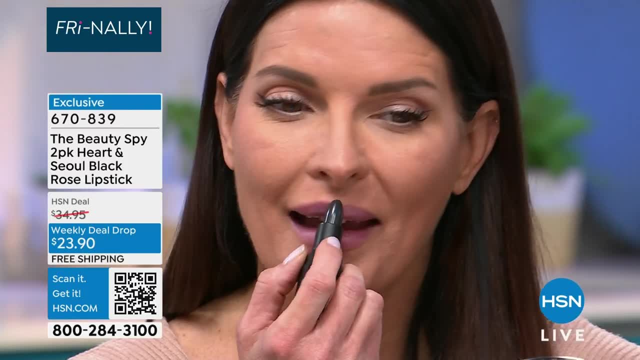 this lady. so what's the magic in this formula? the magic is we're going to take a look at everyone: different skin tones, different ages. the magic really is is that we fly to south korea quite a bit. we spend half of our time there, um, and what's so exciting about south korea is really the 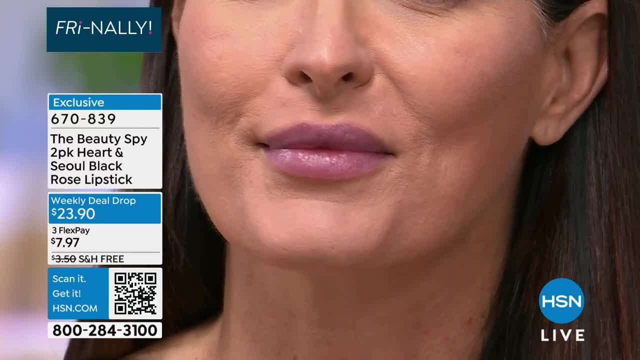 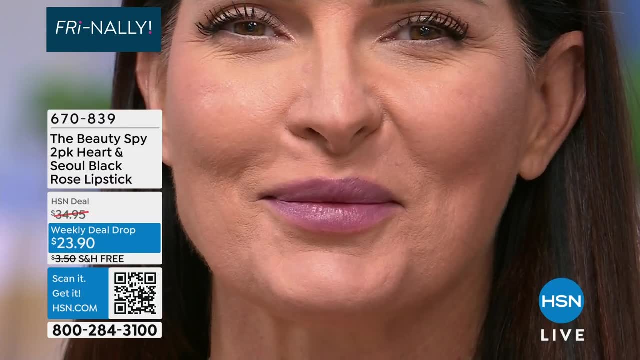 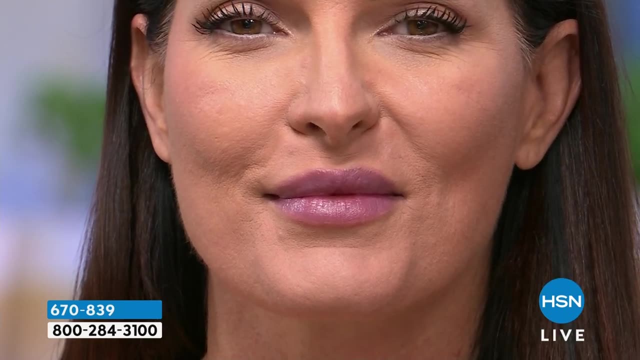 epicenter as far as cutting edge beauty, and they have roses there that are just the most beautiful fields. of these gorgeous roses, they're called black roses. they're actually a very, very deep purple when you see them under the light. we actually extract that oil, the reason why it's ultra hydrating. it helps to fill in all the little. 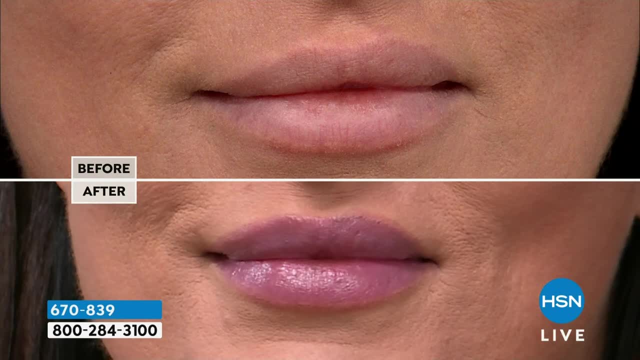 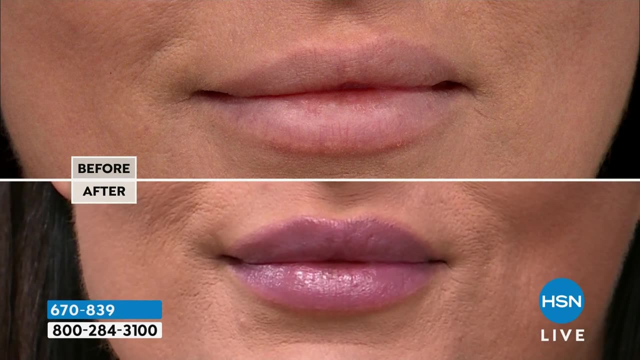 lines that we get in our lips. it really penetrates the lip. so it it's just incredibly hydrating and just makes your lips look pouty, but it also reacts to your own ph. so as you're applying it, you can see here and angie's before her lips are looking a little dry. you see that. 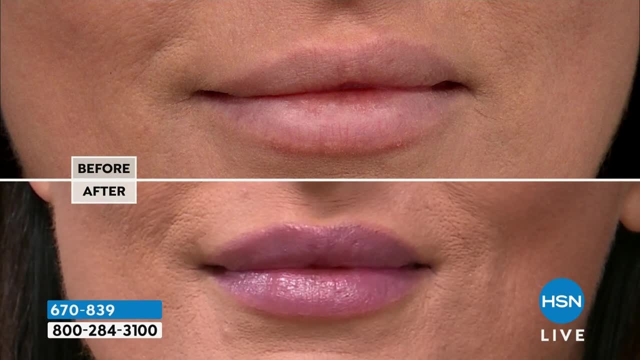 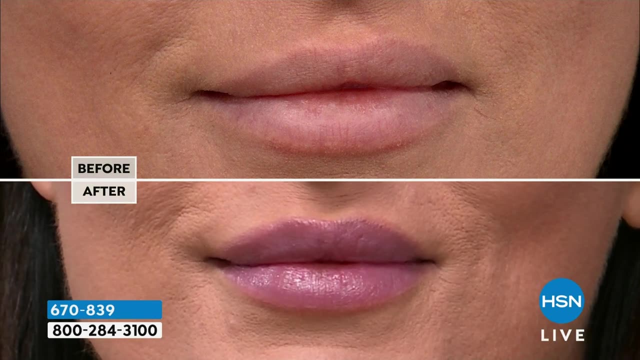 the color looks a little ashy when it mixes with your body's own chemistry. it turns your perfect berry, your perfect um pinky berry shade and it's just a gorgeous flush of color for your lips. so that's why everyone loves it, because my lips are going to be different than angie's and they're. 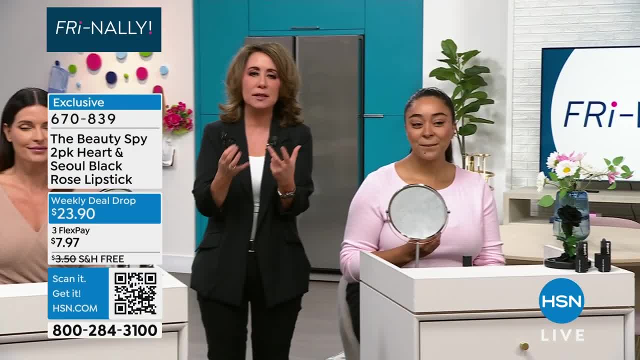 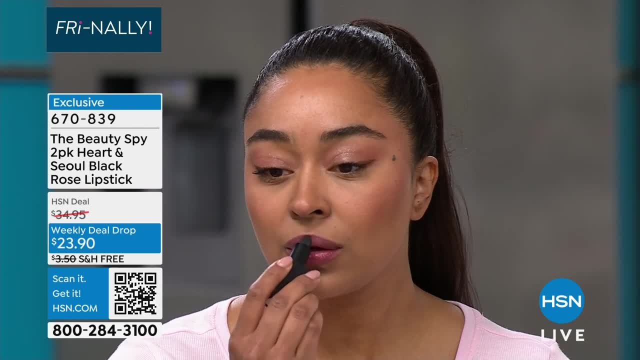 going to be different than kenya's and different than yours. so it really is the first lipstick. i always joke and say it's a lipstick with a little bit of a brain, because it knows what color your lips are just meant to be. i liken it to when you were young: we're running around the backyard. 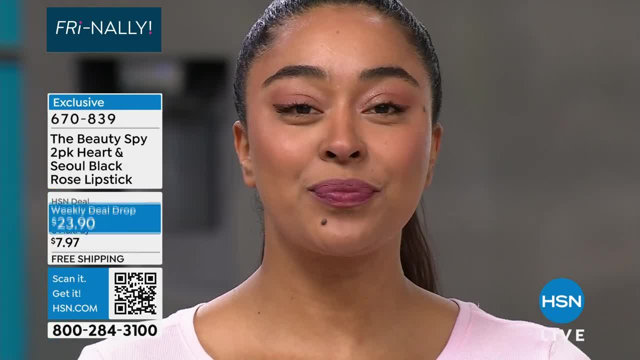 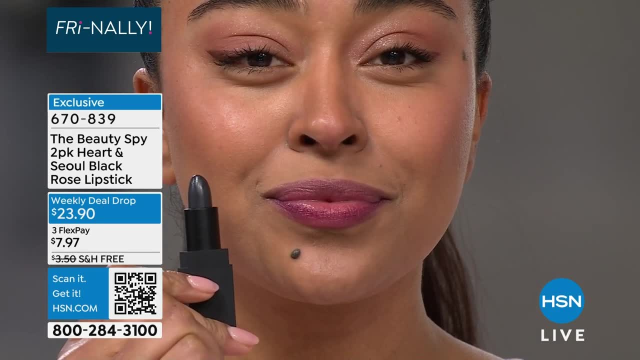 the outside of nature and your lips have that very flushed uh, berry shade. right, you have to pinch. pinch the cheeks, that's what color it comes up. and look at it on kenya. that's so beautiful, isn't it? you know what? it's the perfect color for every skin tone. i think that's what's so amazing. 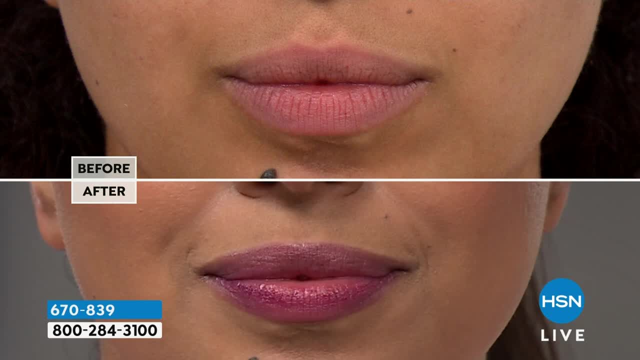 listen, we all have a drawer full of lipsticks and lip glosses that you buy them and you're like, oh, i love it, but yeah, it doesn't work with this outfit or this color. you know, it looks different in the department store. yeah, and you get it home and you're like, what is the? how do i do it? 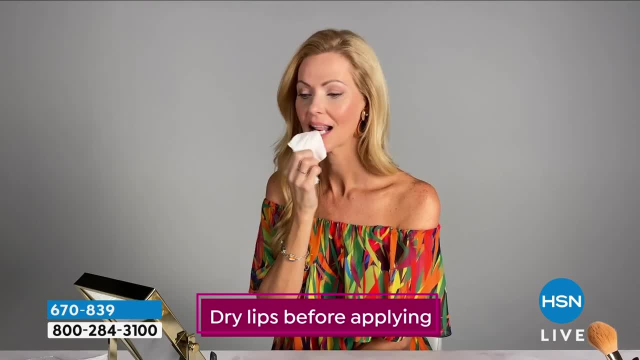 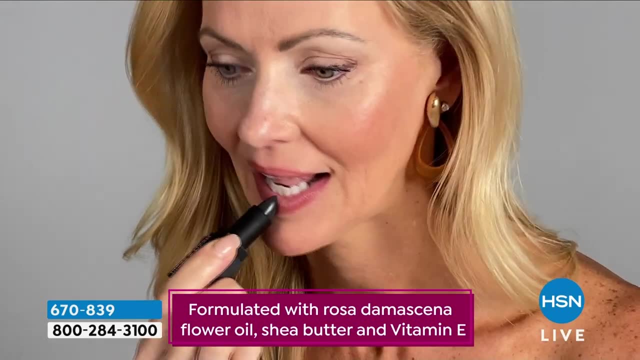 right now. so it's a different color. so you can see, here it's just easy. you're going to apply it to your lips and then you're going to give it a few minutes, right, so you don't need to do anything. but as you're wearing it, it's going to start to develop to your own beautiful shade. so you can. 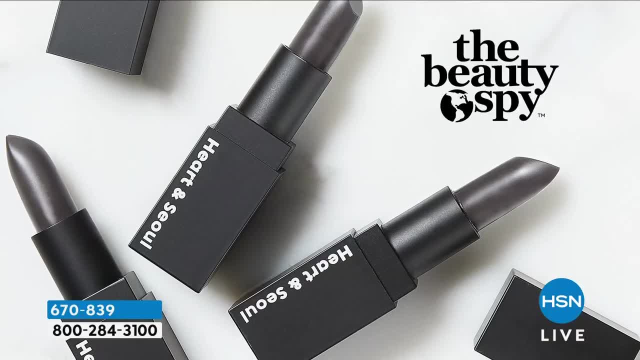 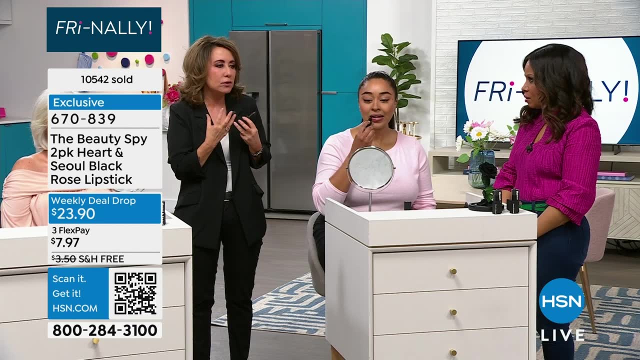 see in the before and after. it's really unique marlo, because this formula is a hybrid between a long wearing stain, um, a hydrating lipstick and a lipstick that is literally, um, going to give you, like, anti-aging benefits. so usually you've got to buy three different lipsticks. you're getting it. 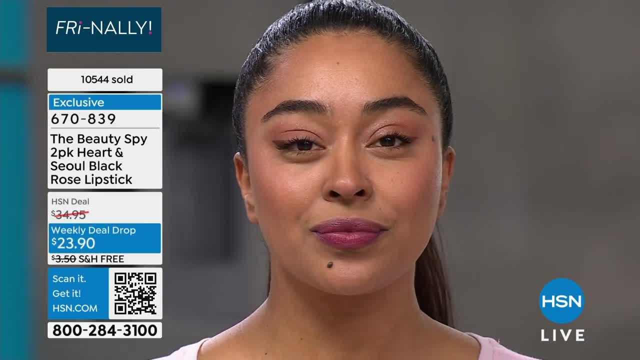 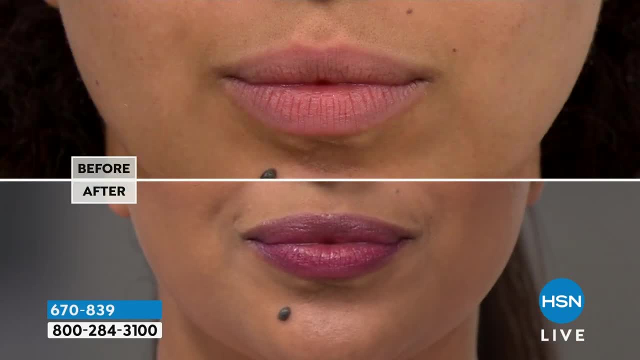 all in one formula. when i say stain, don't be nervous, stain, it's ultra hydrating. so we're going to go here to bo and show you, but i but we're showing a close-up of kenya. i mean, look at, and it's developing, it's using her own. 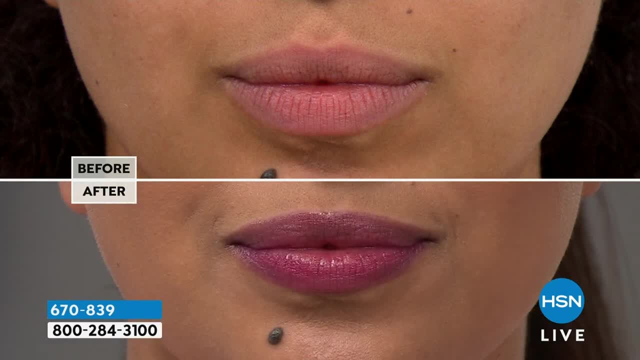 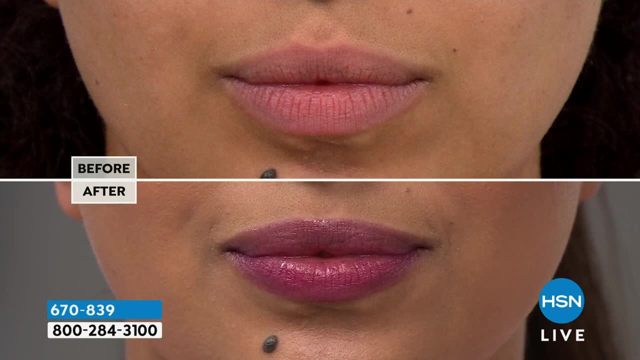 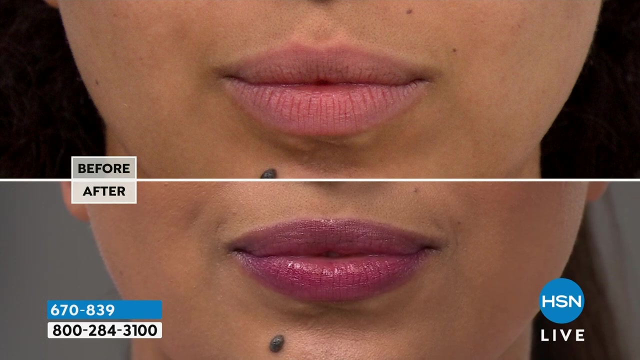 ph, her own chemistry to create the perfect color for her. and guess what? that's exactly what it's going to do for you. it will. you will just naturally look so beautiful. and why buy tonight? it is a bogo. we sell one tube for 24, you're getting two for 24, and it's while supplies last. 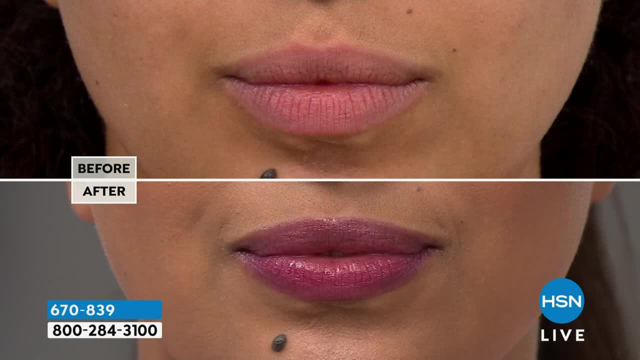 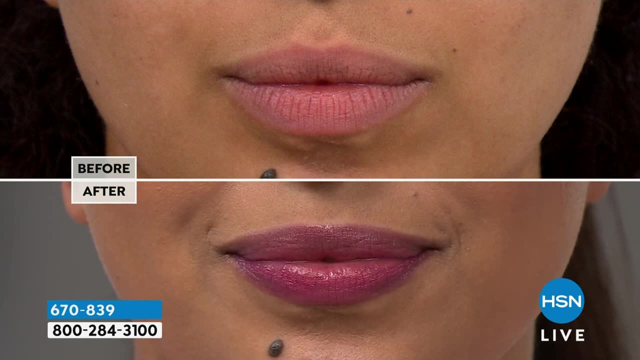 and we don't have a lot of them, so you'll want to buy a lot of them to get in the ordering process. no auto-ship. we can't back order. This is only harvested once a year and sells out every single year. 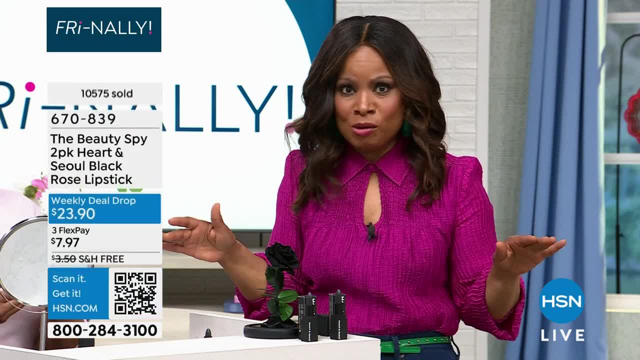 So this is your one and only chance to be able to get heart and soul, and we absolutely love it. Okay, let's go over here because we want to show you this, We want to show you as many skin tones, as many ages, just like I was saying. 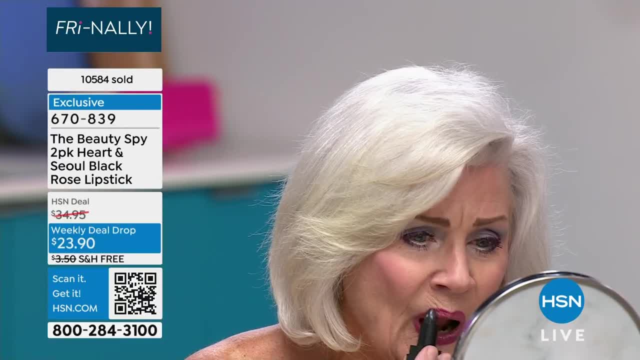 because, like me, I'm in my fifties, I drink out of a lot of straws and I have the worst vertical lines on my lips. So, as we're taking a look at Bo, you can see how on her lips. look at the before. 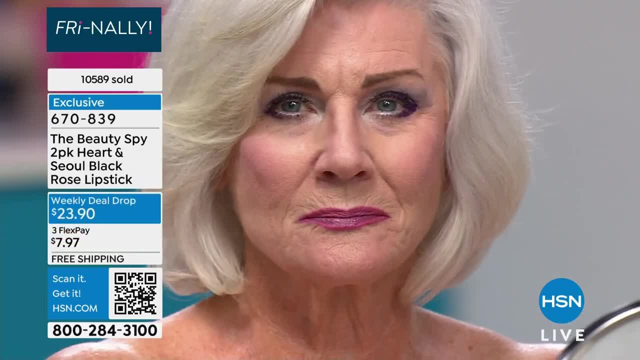 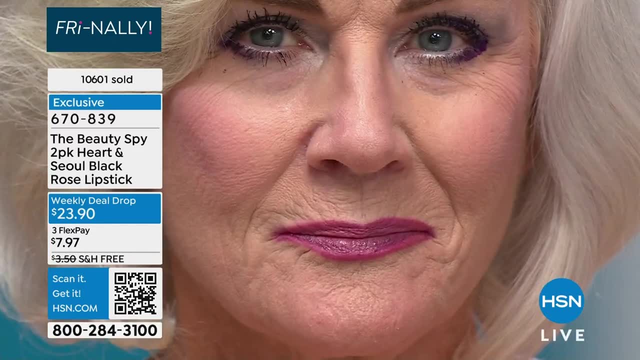 it's incredible If you've got the lines, if maybe you were a smoker, if you're just, your lips are falling from aging. it happens to all of us. Look at how it doesn't migrate. it gets on there. it makes the lips look plumper. 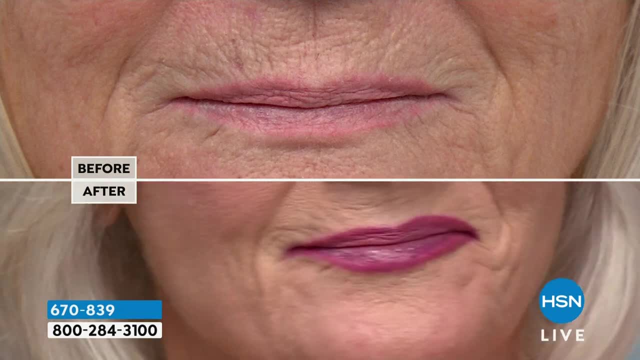 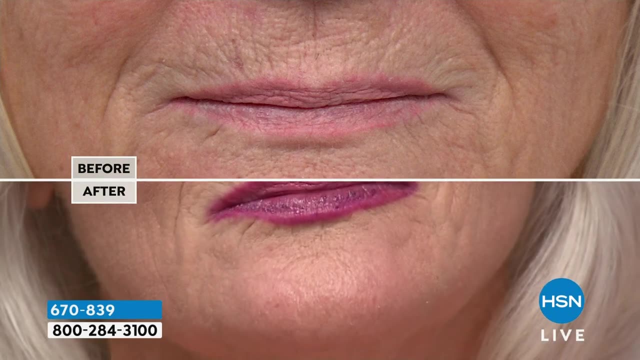 but, Marlo, it's not stinging, it's not burning, it's not uncomfortable on your lips. And look at how beautiful and juicy and hydrated. And on Bo it has this beautiful rich berry shade. that's really her shade. 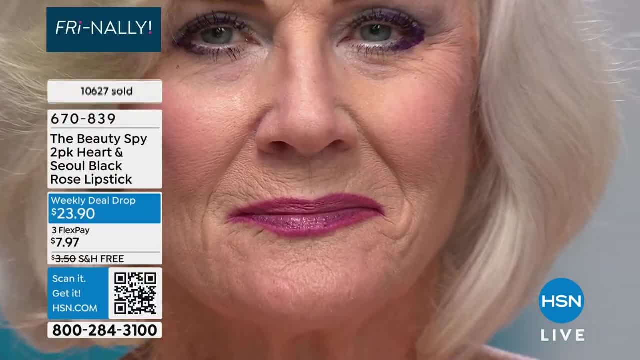 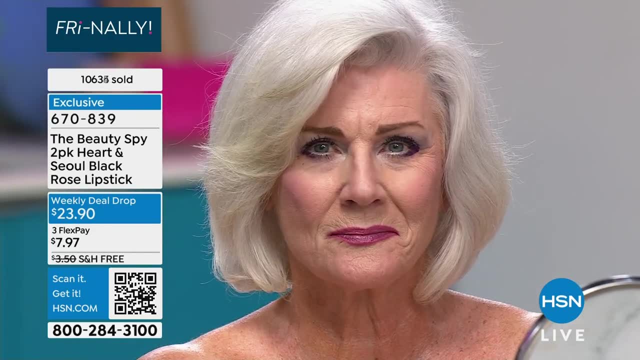 It's just gorgeous And I love that it's never too light or too bright Right, Or never too deep or too dark. Yeah, Because we've all had lipsticks where you're like, oh my gosh, you know, is the lip color entering the room before? 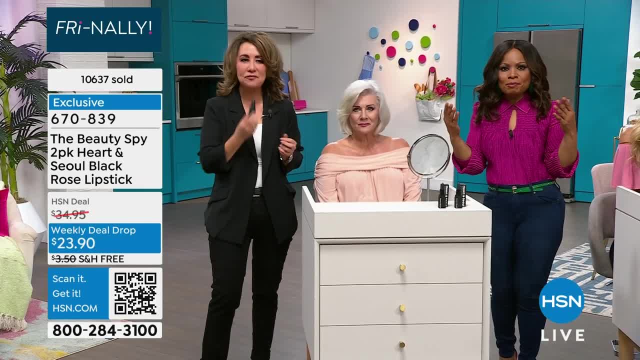 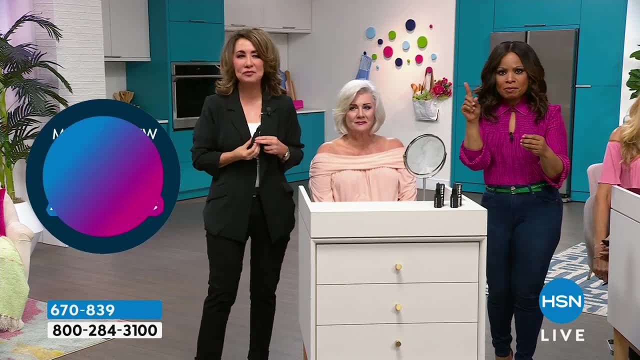 Or if you don't want it to be too dark either. Yeah right, Like, if it's spring or summer, it's always the perfect shade. It is- That's one of the things that I love- right, If you're traveling and you just need one lip color. 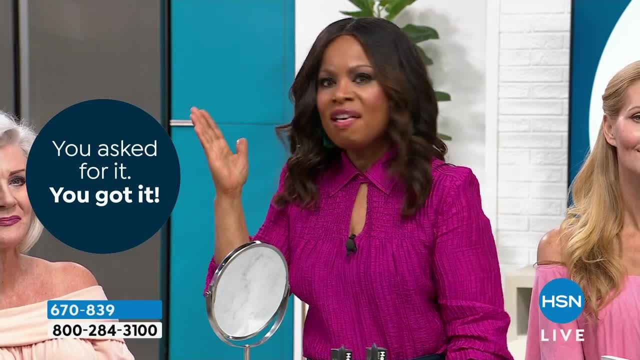 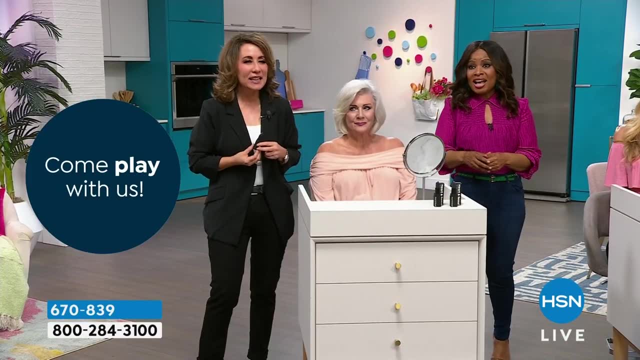 or you just want to nail it every single time. you don't want to have to overthink it. this is what you want. We don't have a lot. this is it. This is it, Harvested only one time of year at over 10,000. 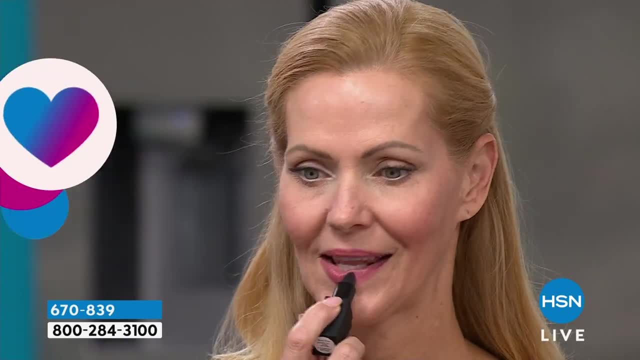 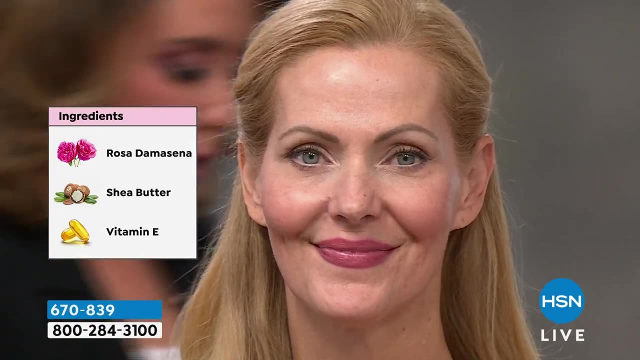 Wow, Okay, So just a final few remaining. Amy's supposed to have this tonight. We don't think it will last, So it's incredibly hydrating It is. So let's talk about the formula, because, to Marlo's point, it's so hydrating. 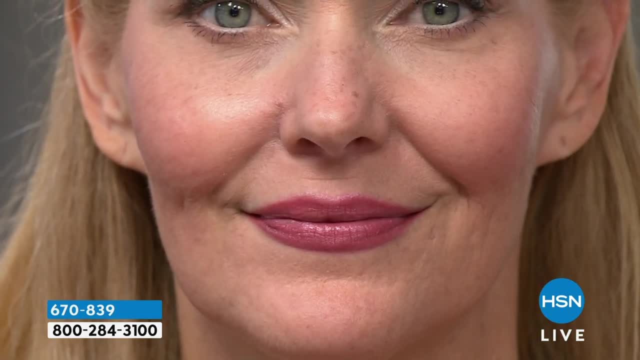 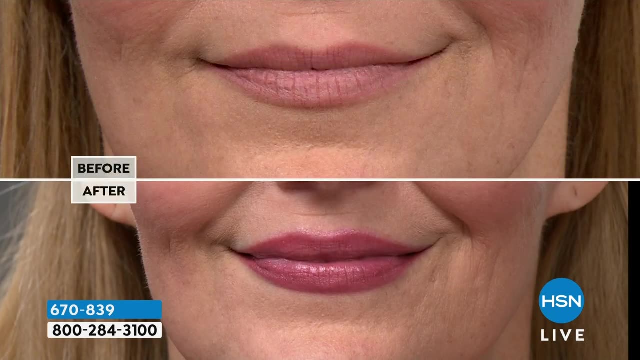 So this formula has shea butter. It doesn't have any of the strange ingredients, like things that you can't pronounce, It's not medicinal And, by the way, it has no odor, like a lot of lipsticks do. You can see here. 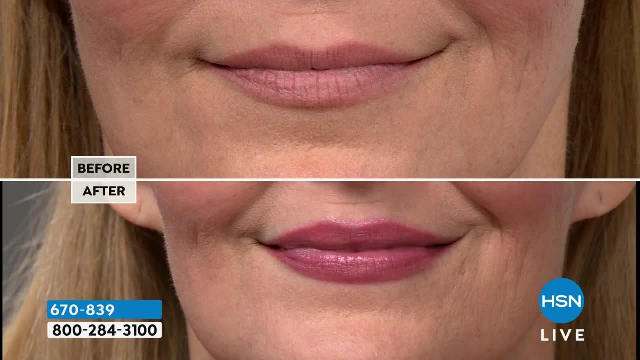 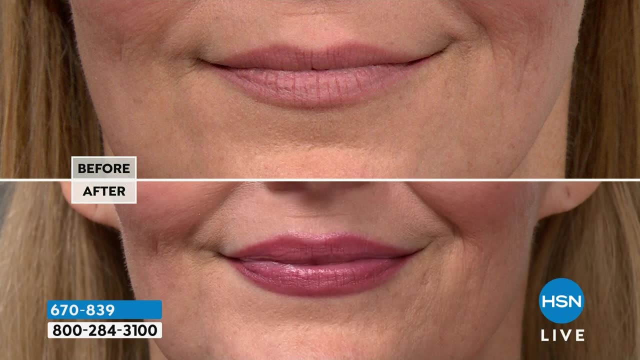 it turns that beautiful berry shade on her lips, but look at how pouty and hydrated and just juicy her lips look. This is that lipstick. So, Marlo, I only know of one other company in the world that uses the Rare Black Oil. 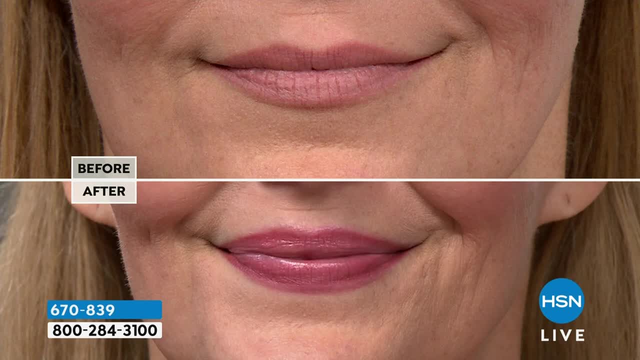 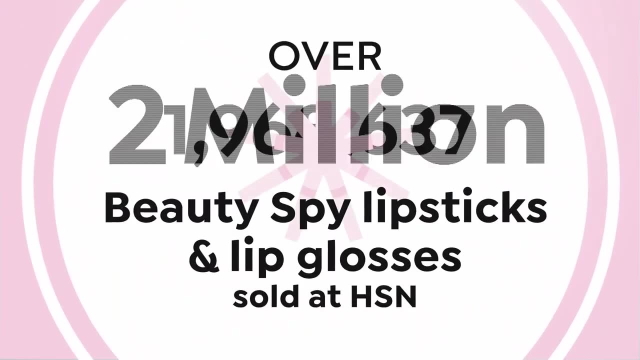 I know It's almost $50 for one lipstick. Yes, I know that lipstick, Yeah. So what's so interesting is we actually at the Beauty Spy, we harvest this oil. We're on the ground and the reason: you guys love it. 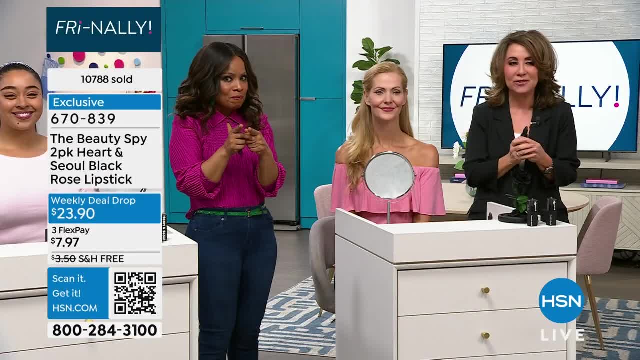 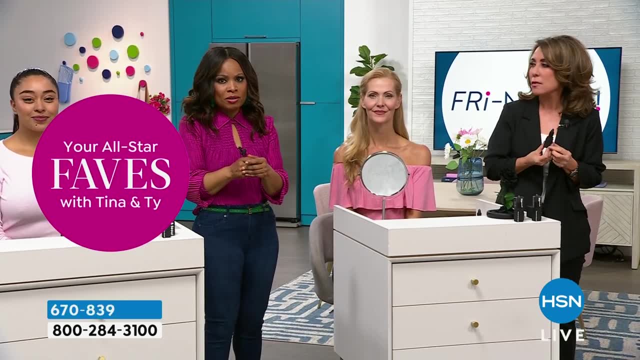 And wow, look at that, That's so. I mean, look at the number. Thank you guys for that. Two million. It's crazy And to your point. I know, and many of you know, that brand of lipstick we're talking about. 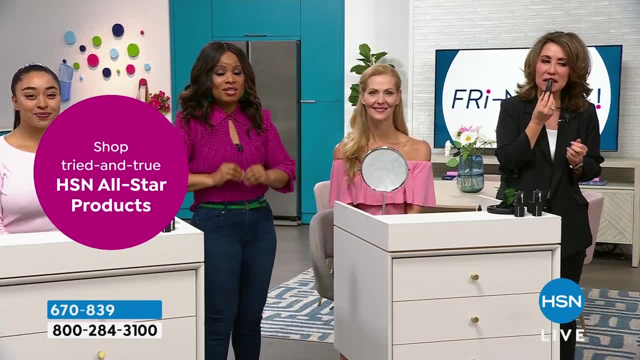 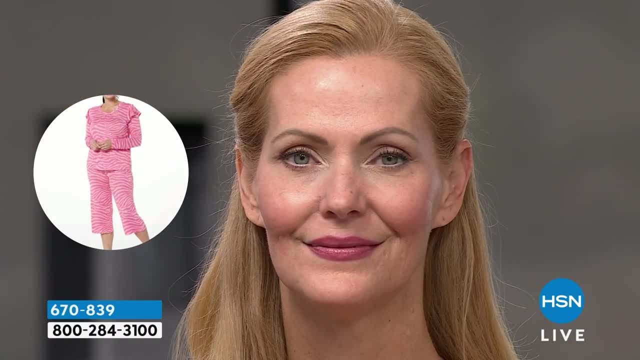 Yeah, It is over $50 for the one tube. This is an opportunity for you to be able to get this at home. You will love it. Always a customer pick, always sells out, And if you look at every one of our models, we're live. 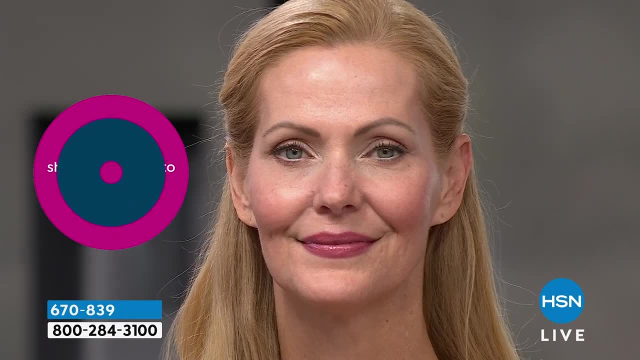 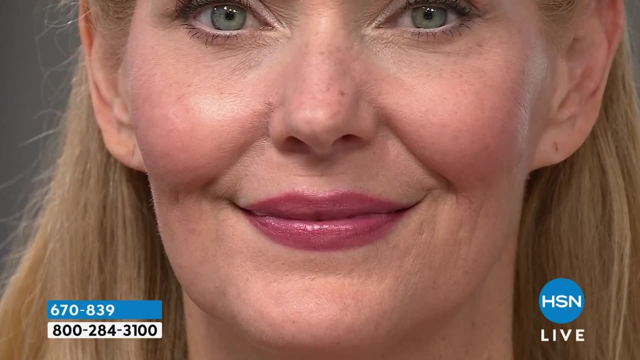 Yeah, Notice that the shade is unique to them, Right? So, everyone, you will have your own unique shade. that's perfect for you. You always look beautiful and natural, super hydrating. That's so beautiful. Going to the gym, to the office, your place of worship. 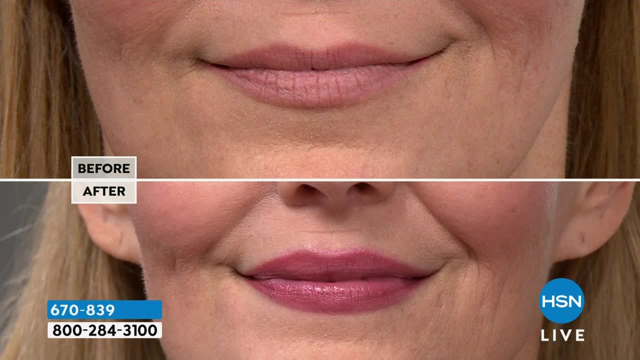 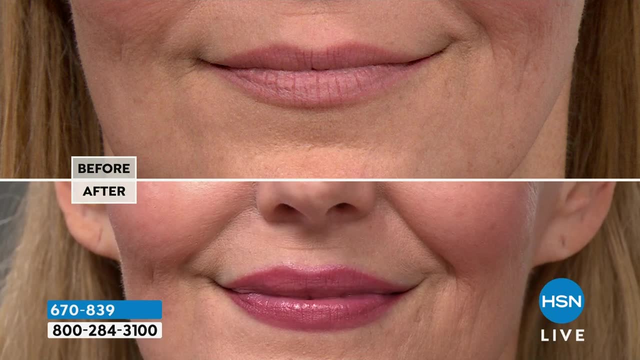 Never looking too overdone, or you know, or your lips are not too bright or too deep, because it works with your skin's own pH balance. Use our express automated ordering. shop our QR code. Remember final quantities. I know that when I spoke to Chelsea, she's like: 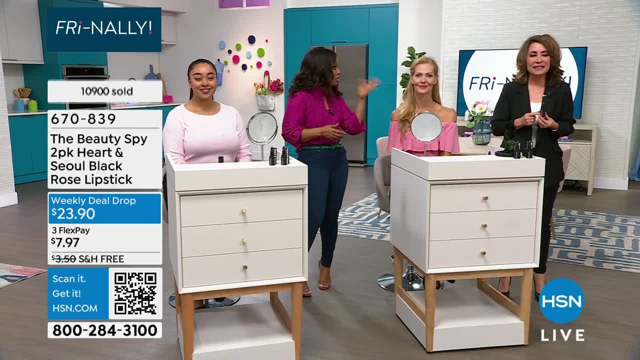 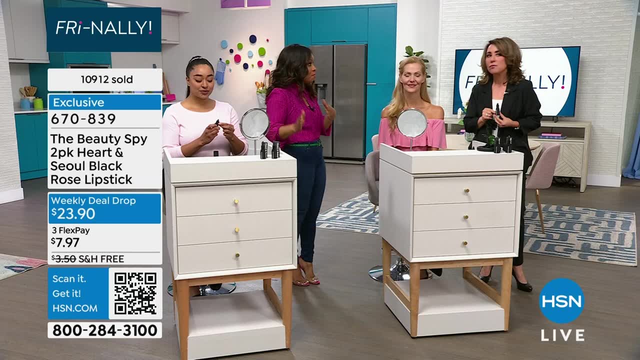 this is not expected to last the weekend. We're so thrilled to have Beauty Spy and Miley Friday. Thank you, I mean you're iconic for all of your beauty products, but that 2 million count number for heart and soul is a big, big number. 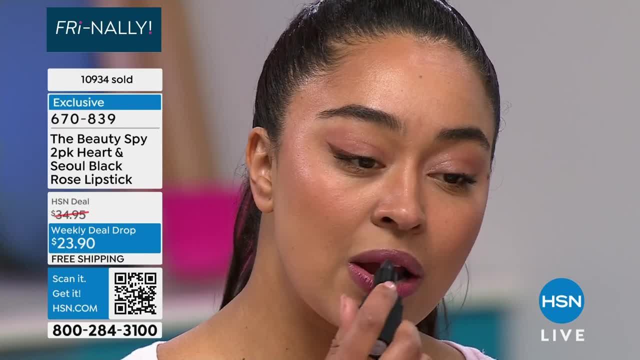 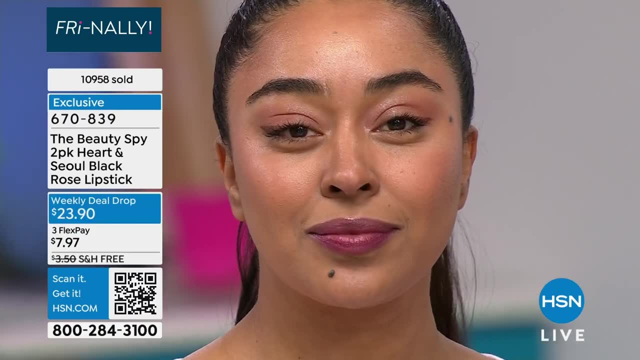 And we appreciate it because it's because of you guys, And I don't know if you know- well, you probably know this Marlo because I've known Marlo for over 25 years now. Yeah, it's a long time, And I started off making lipsticks when I was 17 years old. 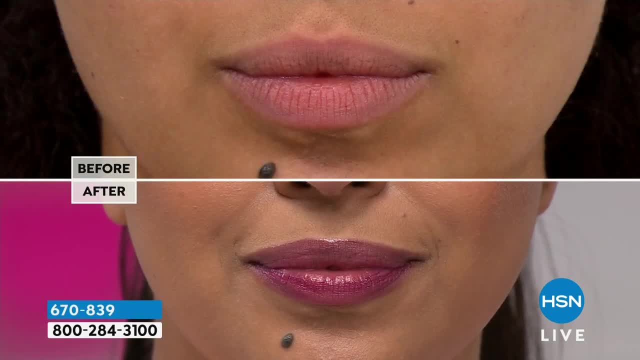 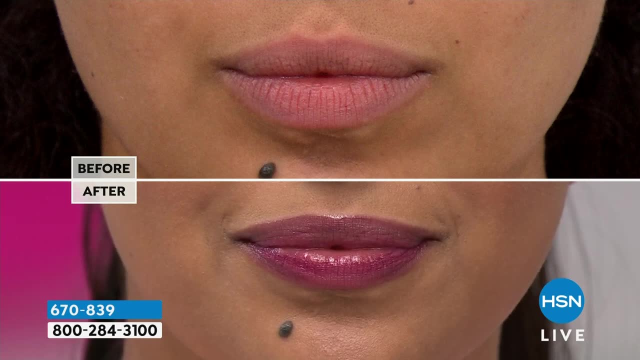 for a dollar 50 an hour in Italy. So lipstick technology has been my passion to share with you guys over the last 30 years, So I'm so glad you're embracing it. Take a look at this before and after. This is not your ordinary lipstick. 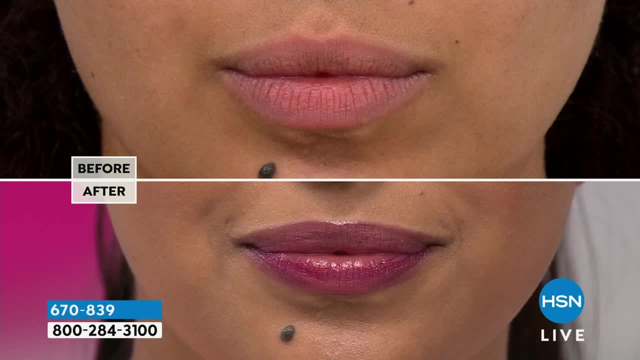 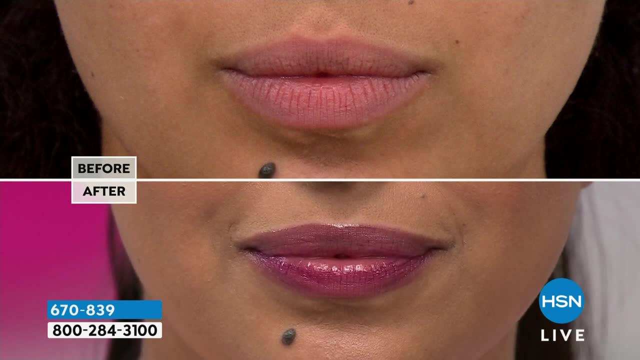 This is literally taking the world by storm because, heart and soul, we have poured our heart and soul into it. You can see the rare black flowers. They're actually deep dark purple. I only tell you that because there's no such thing as black rose. 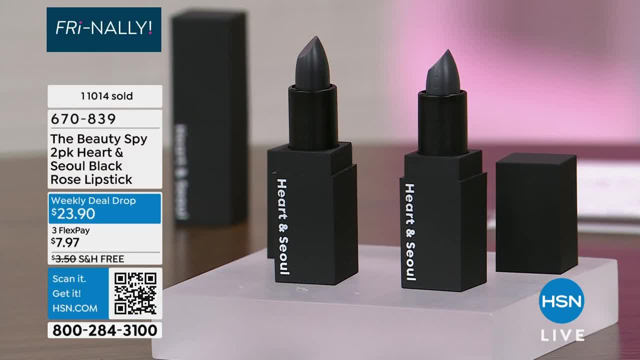 They're actually really dark purple. I just like to be honest about it. But we extract every single piece of these roses. There's fields and fields of them. We're actually gonna show you them. live in South Korea with you on May 1st. 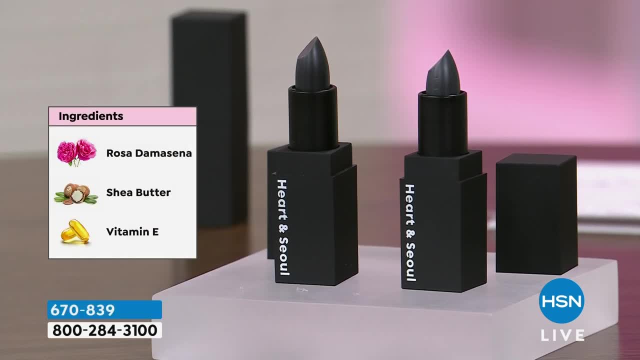 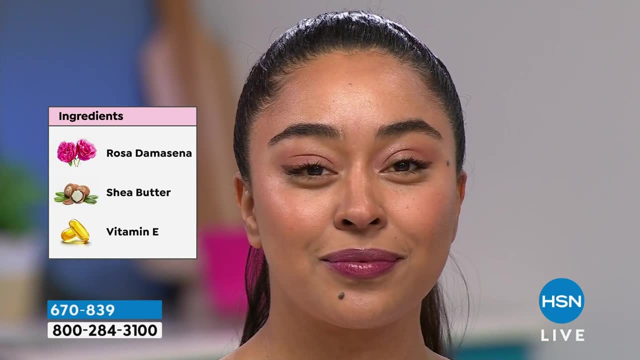 We're gonna be live doing shows from South Korea, So that'll be exciting. But my point is is, if you wanna try this black rose that you've heard so much about and you're tired of using balms that are waxy, that sit on top of the lips? 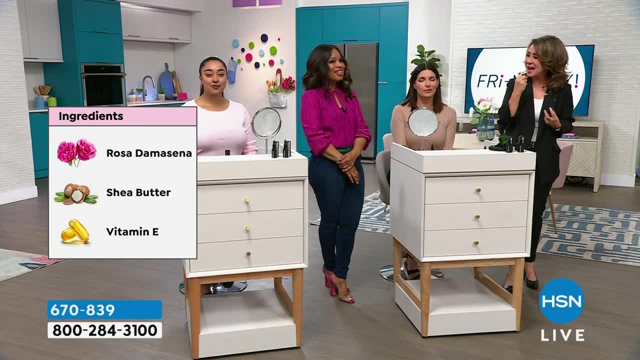 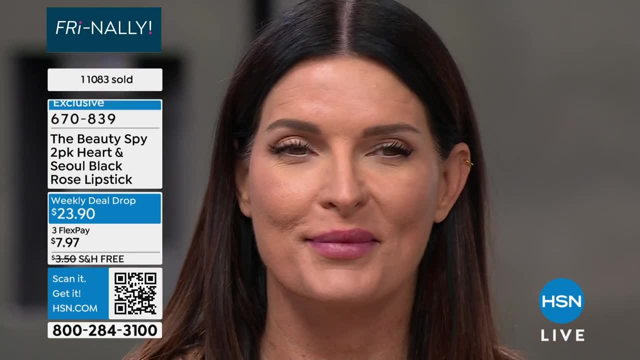 that are uncomfortable. Or Marlo, how many times do you reapply stuff? all day. I agree This. you apply it. It develops to your perfect shade, It's hydrating, It's making your lips look younger, It's giving you the look that your lips 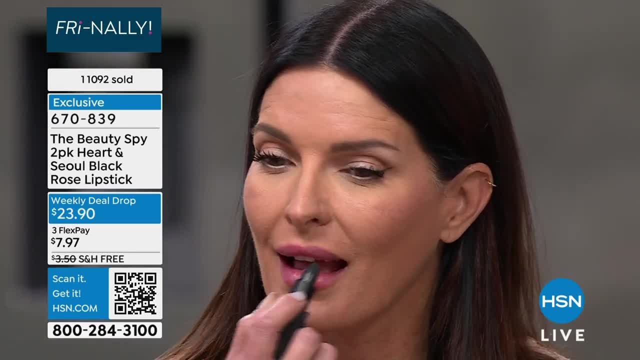 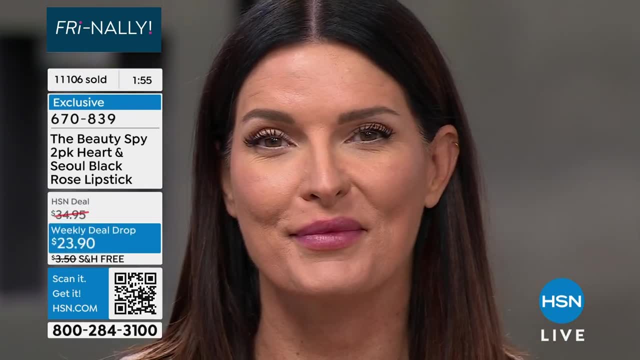 are supposed to be Marlo, And it's easy, And you're getting two and they're individually boxed. It's just the perfect gift. I love that. it's not matte, It's not shiny like a gloss, It's not sticky. 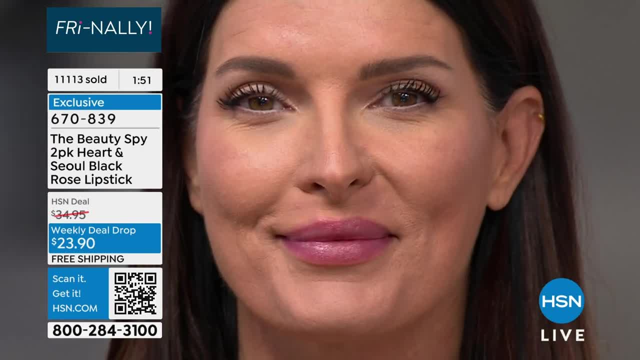 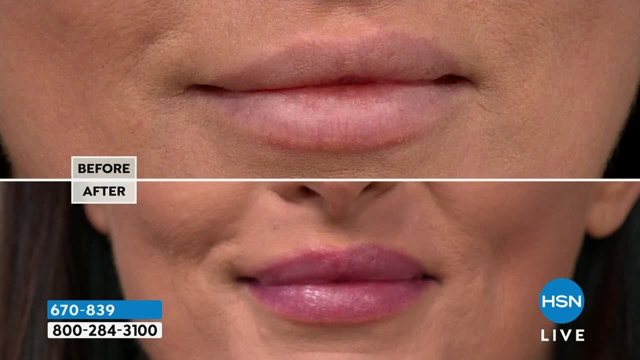 It's not tacky, right. It's just incredibly moist and super hydrating. But look at how natural that color develops. It's such a beautiful color. Look at Angie. I know, Go girl, You gotta get that wine and get the dance going over here. 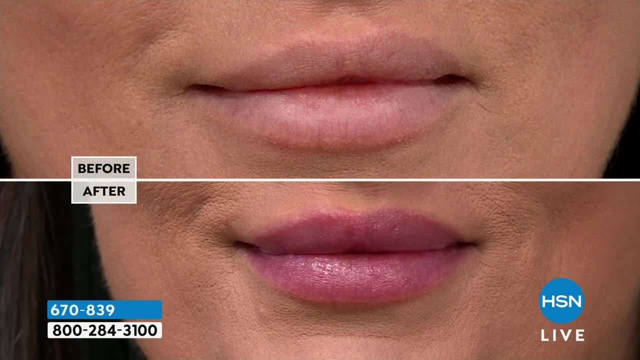 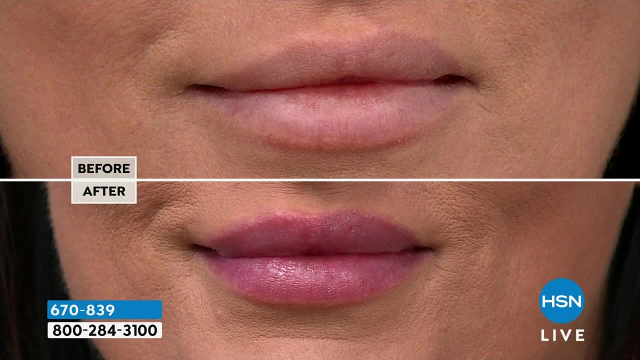 You just naturally look beautiful. That's what I love about it. A little bit like your blouse, Yes. It just naturally develops into this really beautiful, beautiful color. that's perfect for you. If you haven't already gotten into the ordering process. 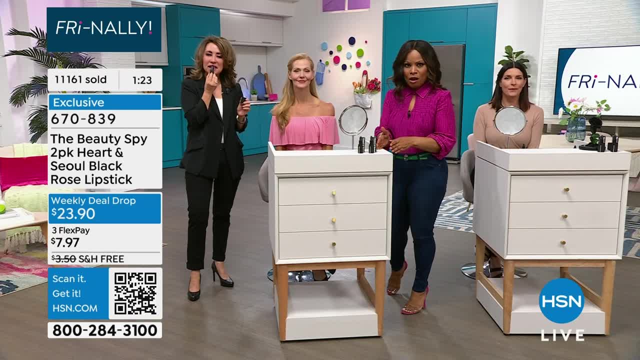 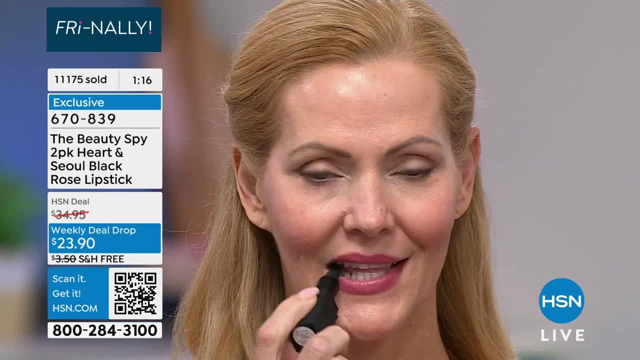 you'll wanna make a move because these are always incredibly popular. We've shown you that 2 million mark of how many of these lip colors have sold. This is the home stretch, with over 10,000 gone. Remember it is a buy one, get one. 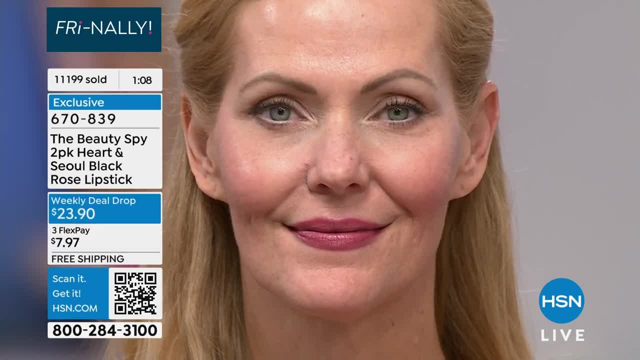 And every skin tone. blonde hair Doesn't matter. Dark hair right, Deeper, darker skin- It works on everyone. Yeah, I mean listen, we're all women. We all do the same thing. I'm just like you. 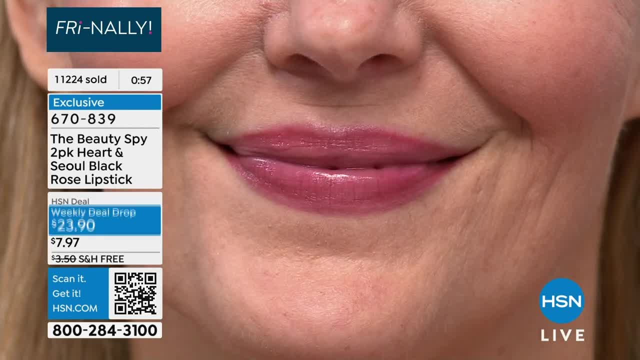 I go to the mall, I try all the TikTok trends. I got it all- Marlo- And what I have is I got a big bill and a drawer full of lipsticks that I've never worn because they don't look the same. 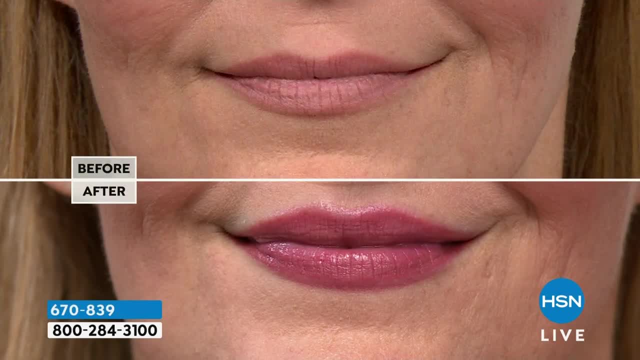 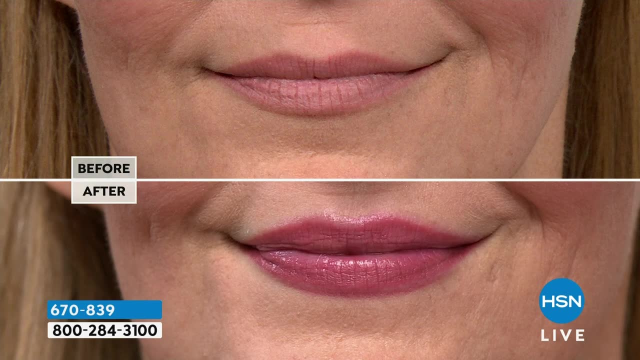 when you get them home, After someone in a store tells you this is your color, Let the lipstick actually choose you. Stop worrying about what everyone's telling you to do. This lipstick thinks for you, It tells you. it shows you with your body's own chemistry. 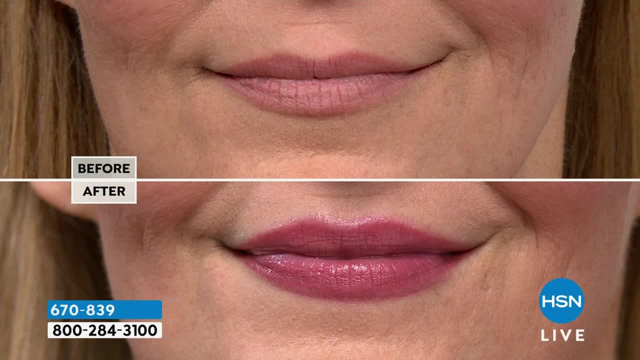 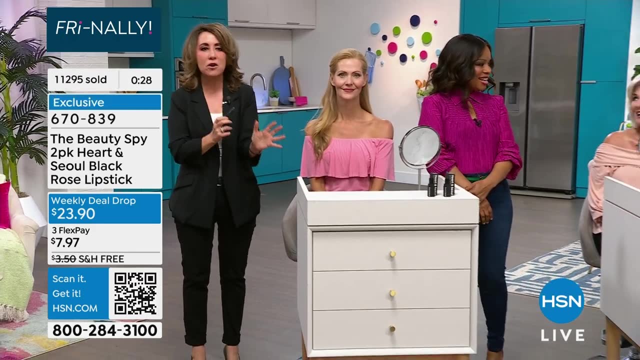 It's not hokey, It's got no weird smells, No animal testing, which is great. And look at the difference in everyone's lips: Marlo and myself, and Angie and Beau- we're all different ages, tones, everything- And it's one lipstick that you guys love. 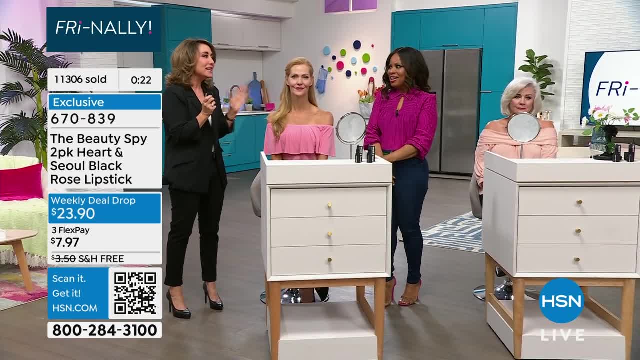 So I get very passionate about it, because we can only do it once a year. Yeah, So it isn't like we're not sneak peeking it again in December. It won't be back until 2025. And I know it's almost gone. 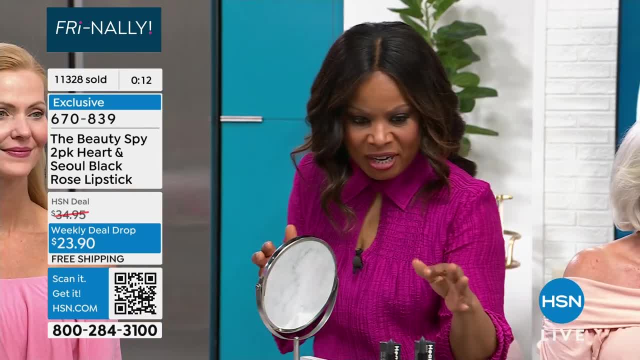 I don't know. when you first look at it, you're going: oh my gosh, what is this? Right? It's so dark, right? It looks like black but- So cool As soon as you put it on. 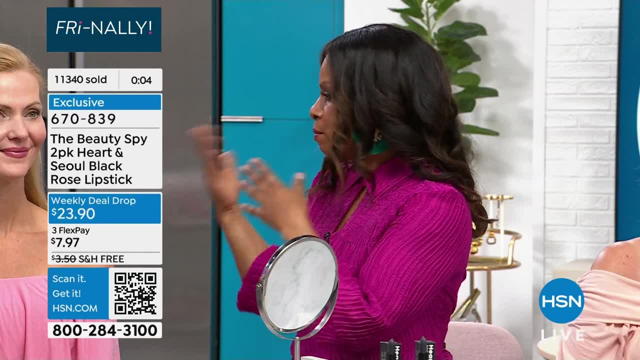 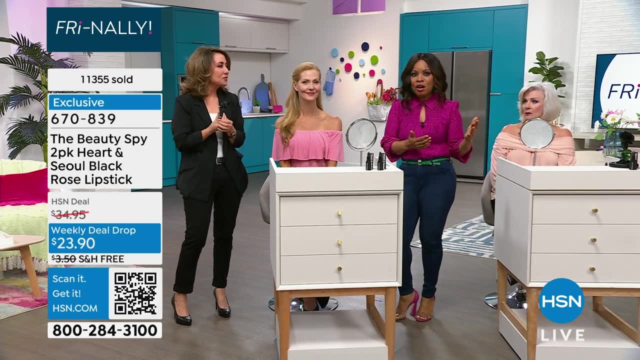 you'll see how this color just develops. That's perfect for you, And when I look at you like it's a little bit lighter on you because it's working with your own skin's chemistry and pH balance And it's a little bit deeper on others. 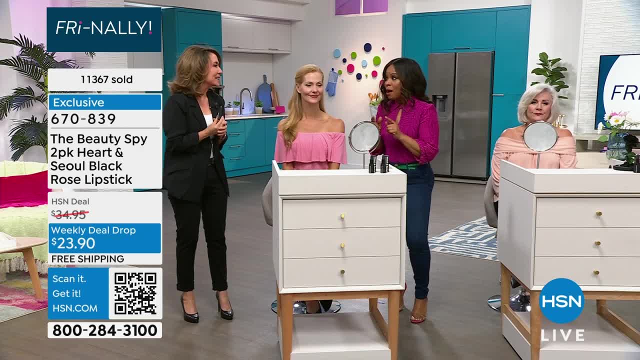 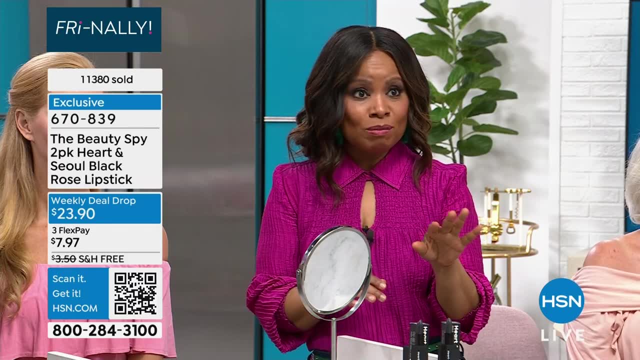 but it is absolutely stunning. Well, Chelsea, we're gonna be wrapping it up. We're so proud. Are you up to have it? Okay, I understand. whatever's remaining will be with Amy in the 11 o'clock hour. Don't wait. 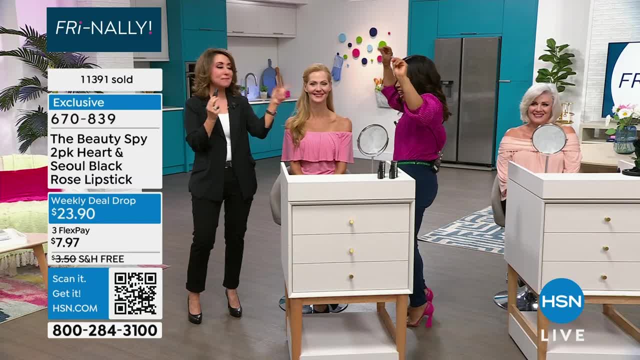 You'll have your chance now. Can I do a little dance with you, girl? I'm coming back, I'm coming back for you. I bring in the wine. I have a date with you Friday night. Oh, I can't wait. 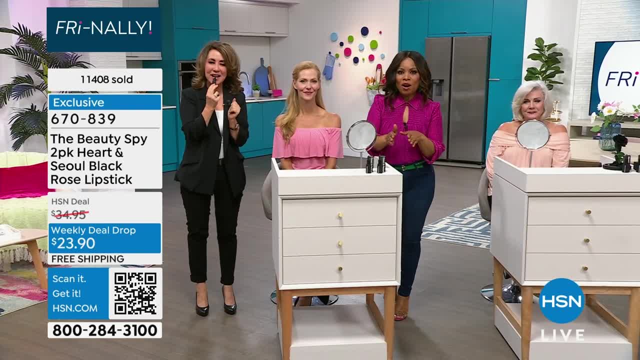 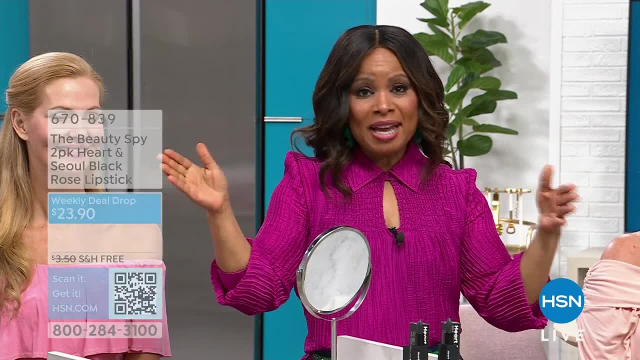 Any Friday you wanna pop in. you certainly can Thank you, Marlo, If you want. your heart and soul definitely continue to shop. Thank you so much for your phone calls there. Let's talk about when to watch. You don't wanna miss any of Chelsea's show. 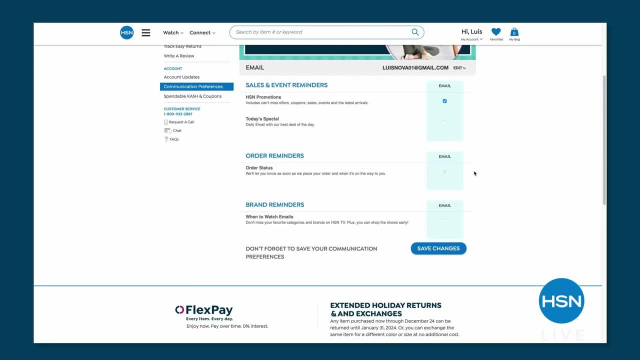 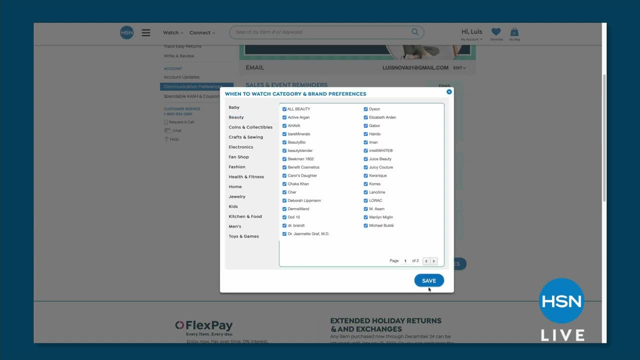 We know, of course, her as the beauty spy, and you can sign up for a beauty spy and when to watch. We have over 350 brands and we certainly are inviting you to be able to select your favorite brands and we will be able to email you. 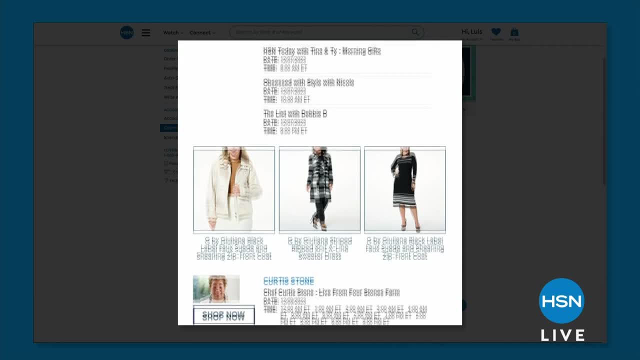 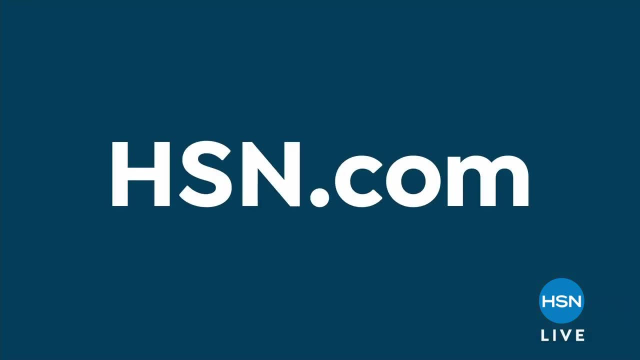 and let you know when you're going to be able, when they'll be on the air. So that's gonna be a lot of fun. So here's: what you need to know is that we, in fact, are going to be moving on. 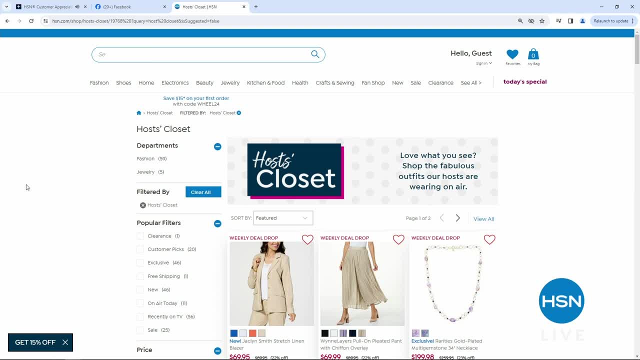 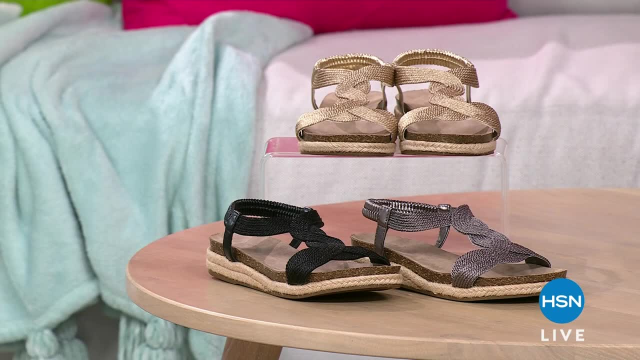 and we're gonna be introducing everyone to Casey Bates. Casey happens to be our Kenneth Cole expert, and Kenneth Cole is a world-renowned brand that so many of you know. In tonight's show, we actually have two different styles from Kenneth Cole. 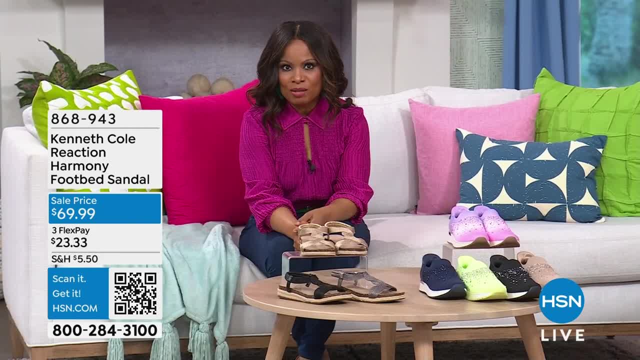 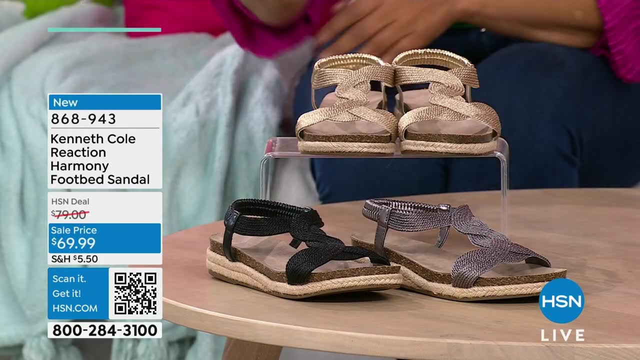 You're looking at the first, which is a sandal that is brand new, that we have in three different colors. We have the gold, we have it available for you in pewter, and then we also have the option offered in the black. 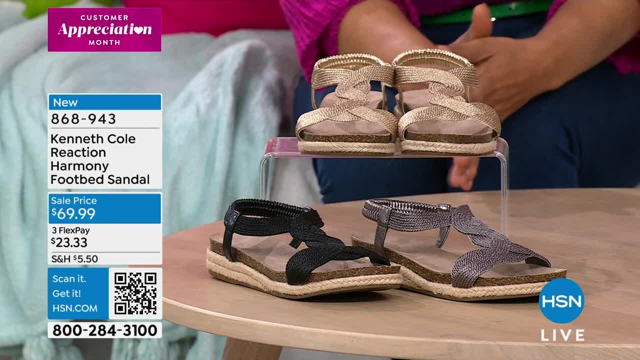 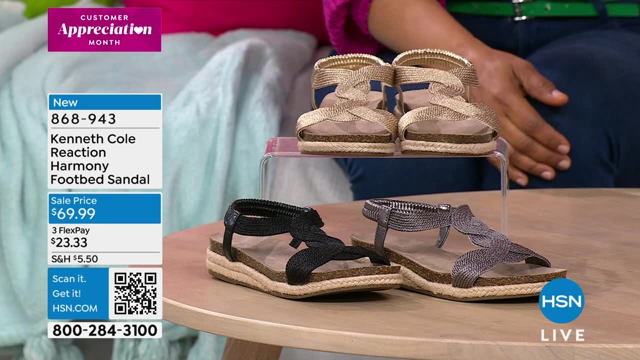 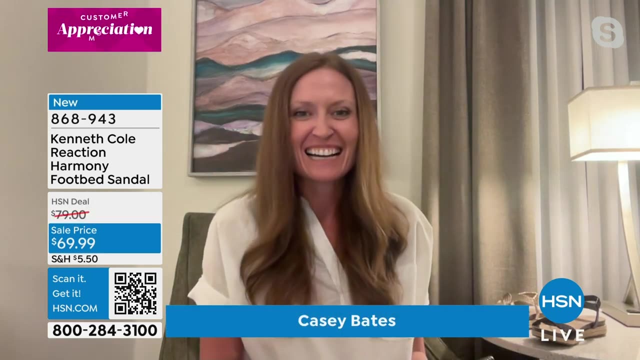 We share these with you in sizes in medium width and sizes five through 11.. And, Casey, I wanna take a moment to welcome you into the show as our footwear expert and as our Kenneth Cole expert. Happy Finally, Friday, Yay. 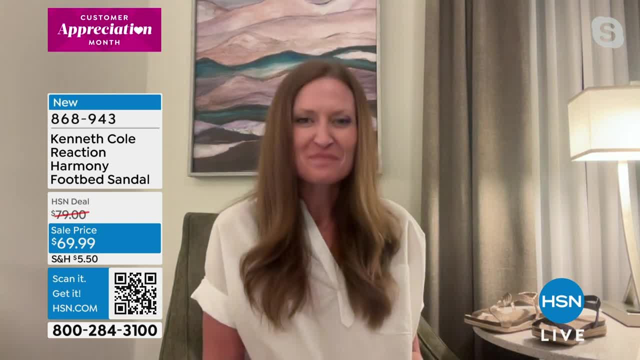 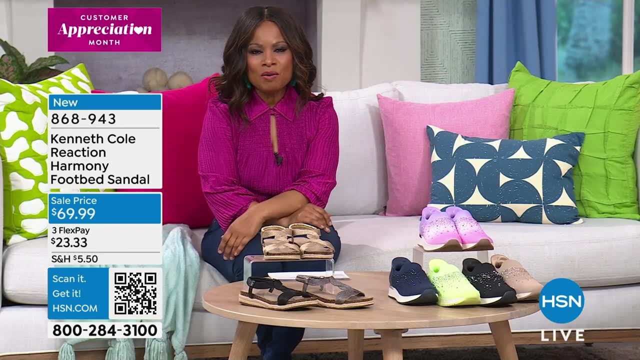 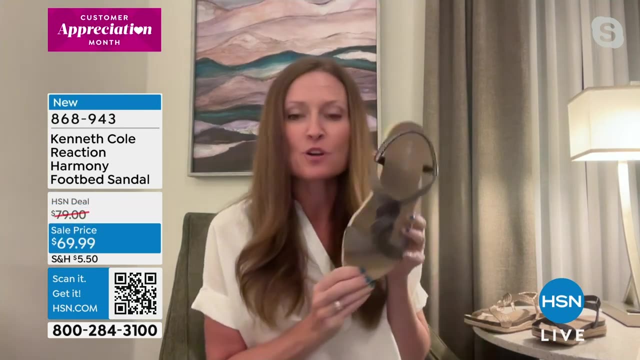 Well, welcome. Let's tell everybody a little bit about this great sandal that's brand new, with this wonderful footbed that you and the entire team are bringing to us tonight for the very first time time, Very first time. I got these overnighted to me yesterday. I'm actually out of town right now. 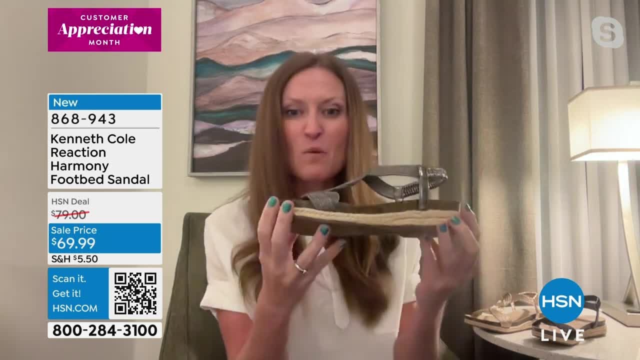 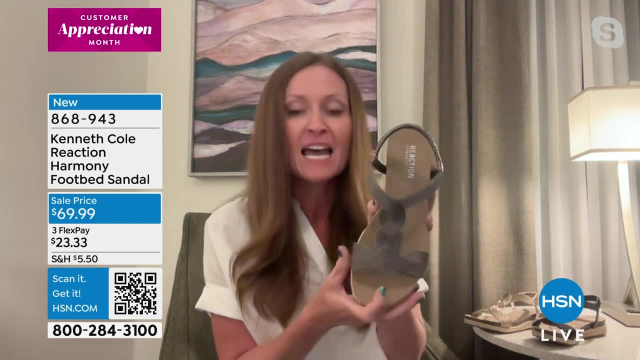 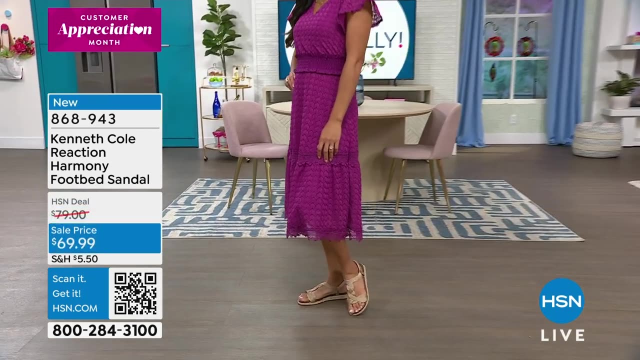 I said I have to have these If we are launching this. I want these in my hands because they are gorgeous. I'm so excited to be launching these tonight. This is the Harmony And in traditional Kenneth Cole fashion- comfort and style. you get both, which is so exciting. How beautiful are. 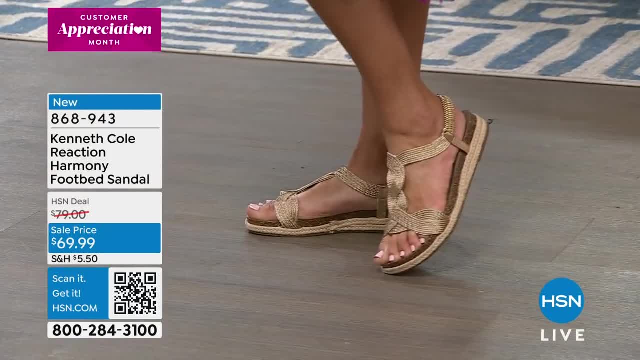 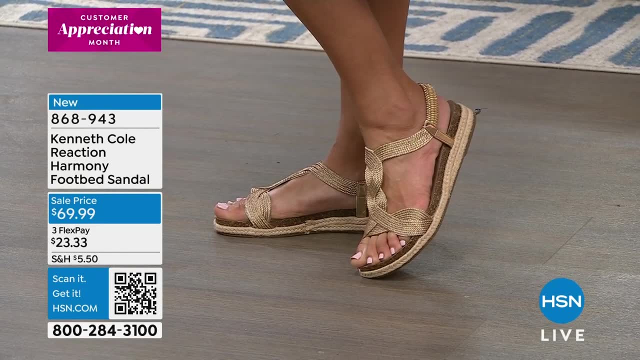 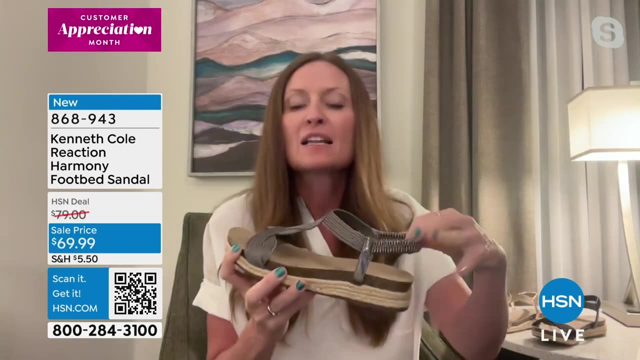 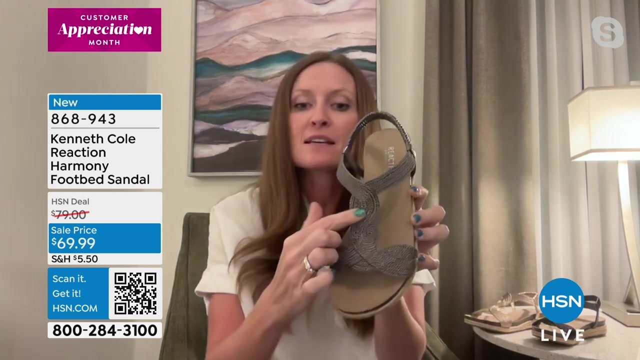 those. I love the style of this strap. The T-strap is so on trend and we have that beautiful woven metallic. It's just such a gorgeous sandal and it's comfortable. So you have this elasticized slingback, which is so nice. It makes for easy on, easy off, And this is a woven fabric, but on the 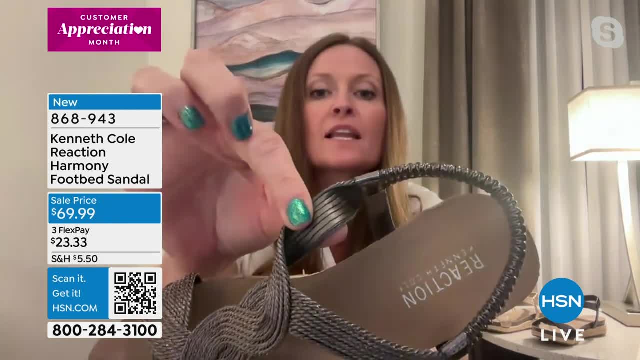 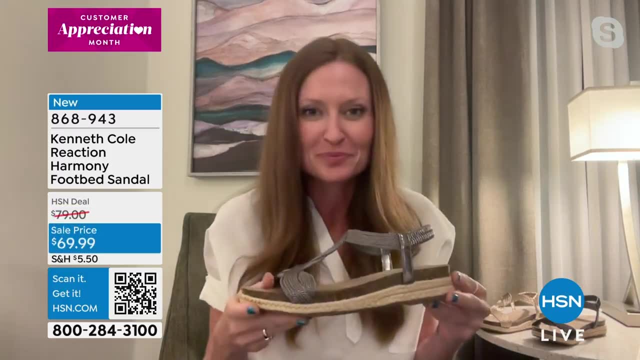 inside. it is so, so nice, So smooth, And I love that. It is like butter soft, So you're not going to feel it at all on your foot. This is just such a gorgeous sandal. Oh my gosh, We're going to show a closeup of this gold, and it's. 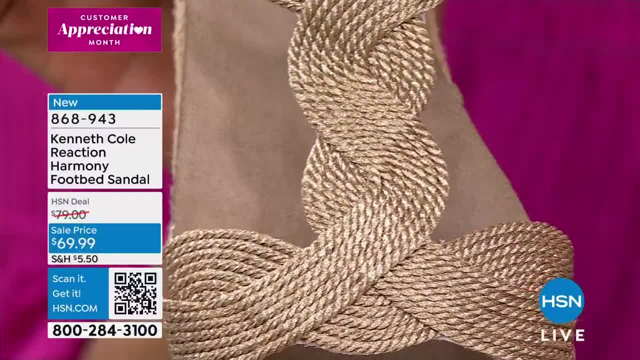 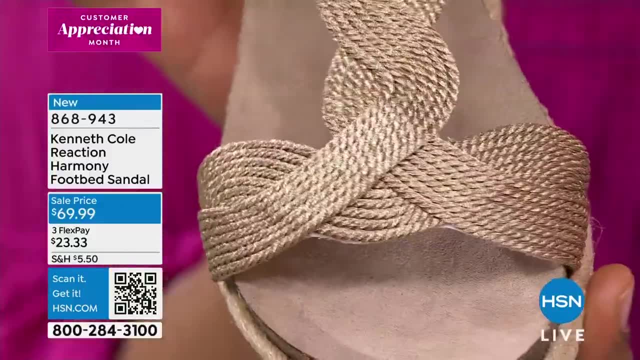 the perfect gold color. I mean, I know, I know, for all your dresses, all your maxi dresses, all of your your trousers. I mean, that is a. it almost looks like a Cleopatra sandal, doesn't it? But 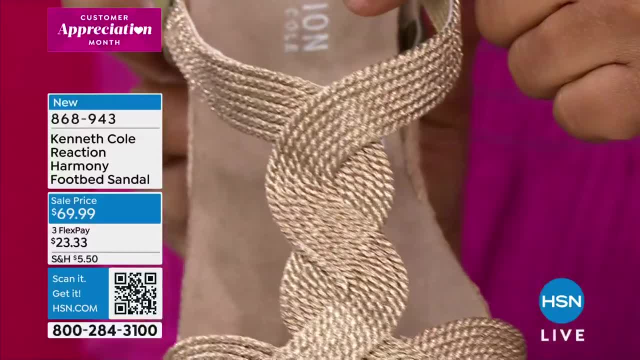 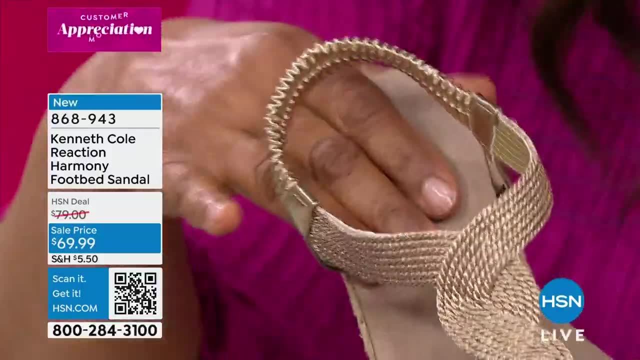 that it looks so rich with that individual braided look that goes all the way up to your point in the back. You just slip the sandal on, So that's going to be nice. It's nice and soft. And then even look at the footbed. This footbed is 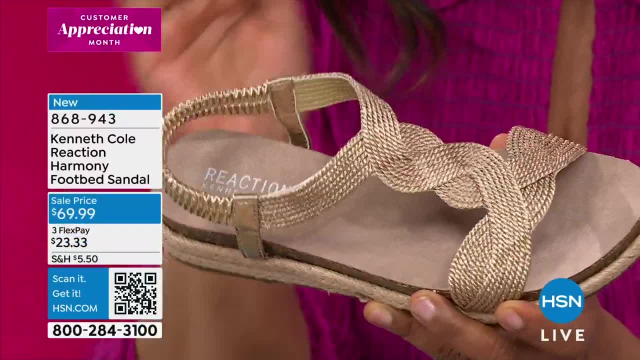 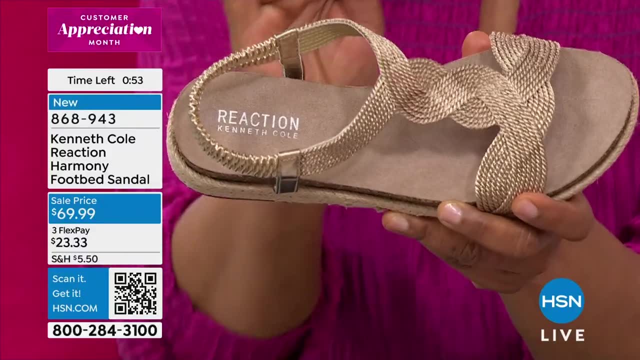 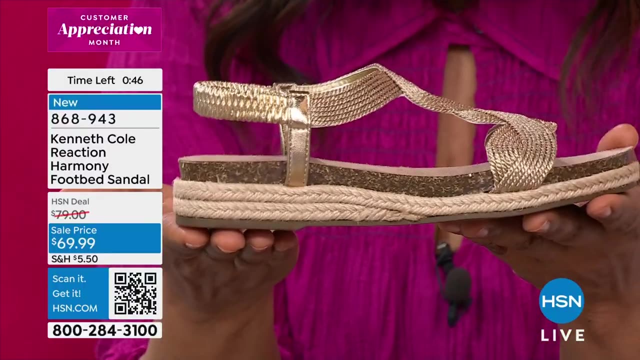 made with a micro suede sock. So even in the three different, three digit temperatures that some of us will face, unfortunately, coming up this summer, your feet are going to be nice and dry and comfortable on that footbed. I'm going to just turn the sandal on the side because you can see. 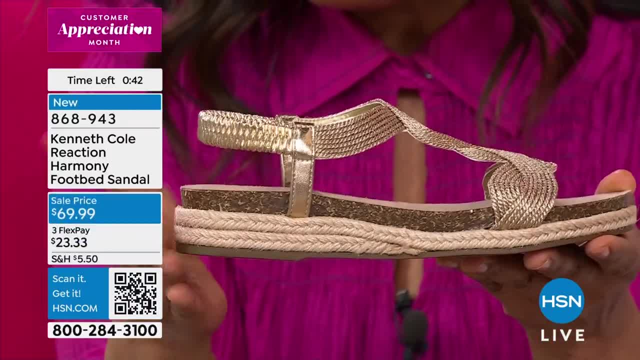 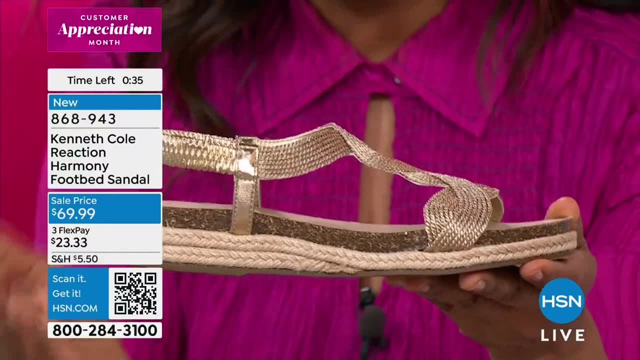 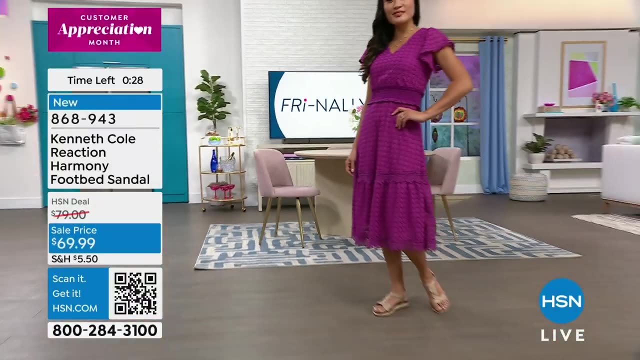 that you've got that little bit of a lift in Casey. That's so important because we know just having that little bit of that one inch lift really is so much easier on our hips and on our backs And as we're walking right, So comfortable, so stylish, and look at this blend of texture. So you have. 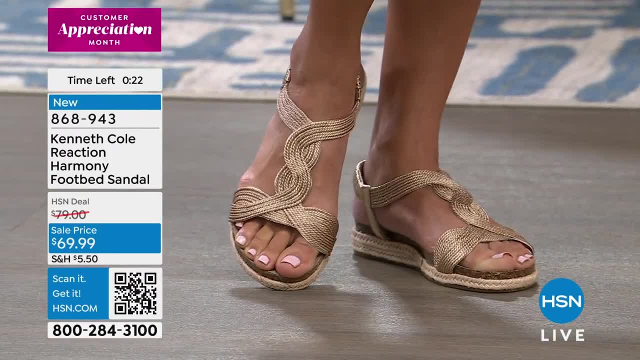 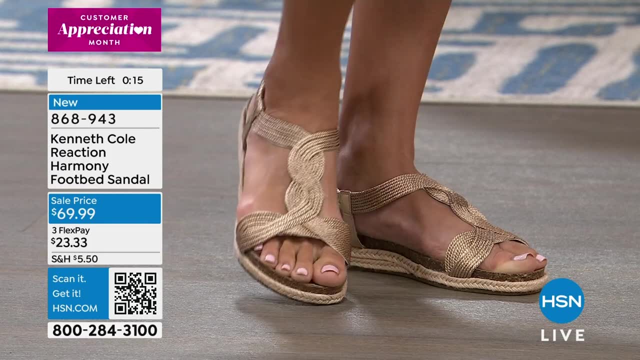 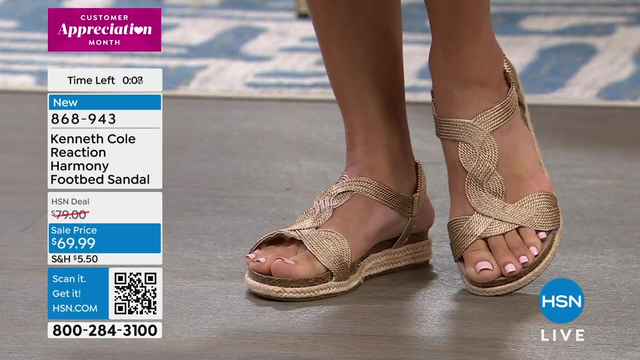 the rope, you have the cork and then you have the woven fabric. So it's really such a visually interesting sandal, So stylish, so comfortable. I cannot get enough of saying how Kenneth Cole has done such an amazing job of blending both Absolutely. I'm going to show everybody a. 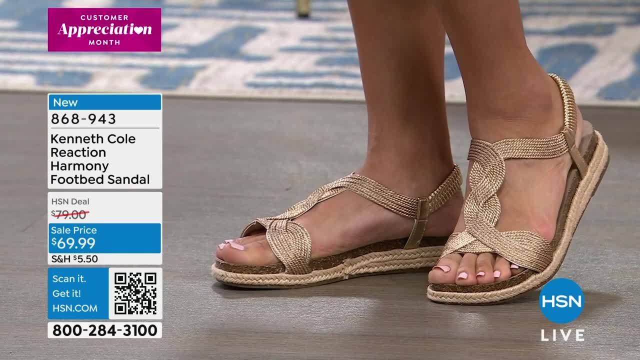 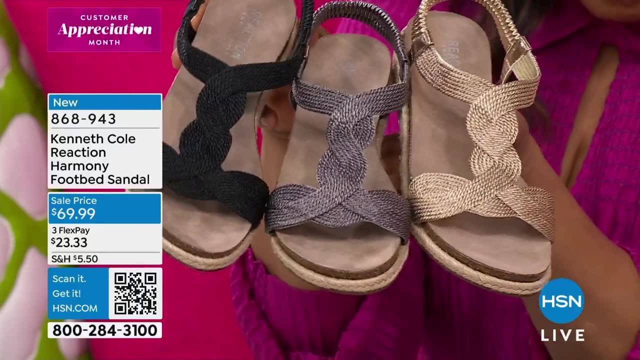 close-up of the three different choices. I am encouraging you to shop. We get to offer these to you on three credit card payments of $23.33.. I have the gold, and the center is going to be the choice that we are calling pewter, And then we also have this in the black, If you're looking. 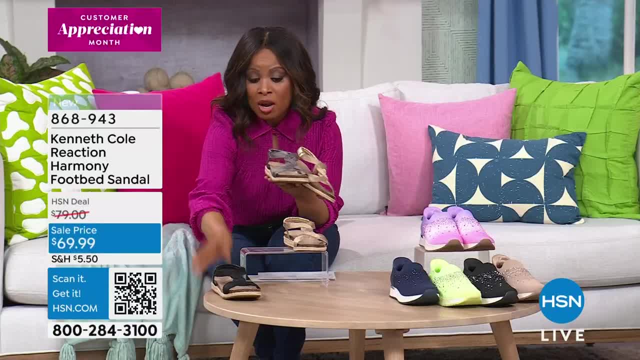 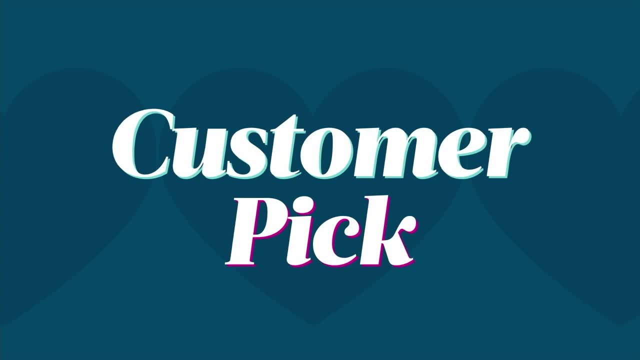 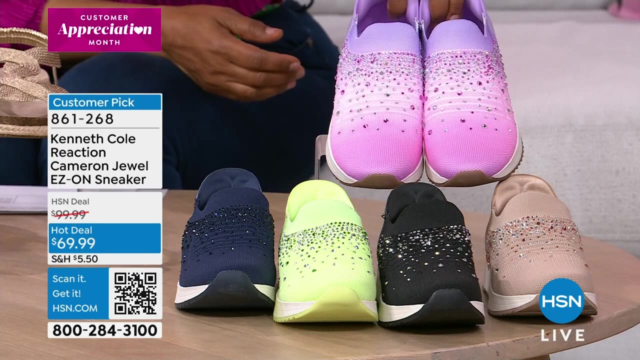 for a perfect sandal. this might be a great choice. We are going to leave it here, but we want to show you that it's. a slip-on sneaker that is filled with all sorts of gorgeous jewels At the very top is one of my personal favorites. Look at that shade of pinks and purples and lilacs. So this 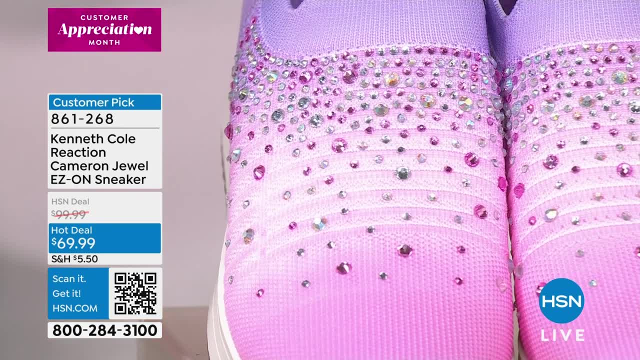 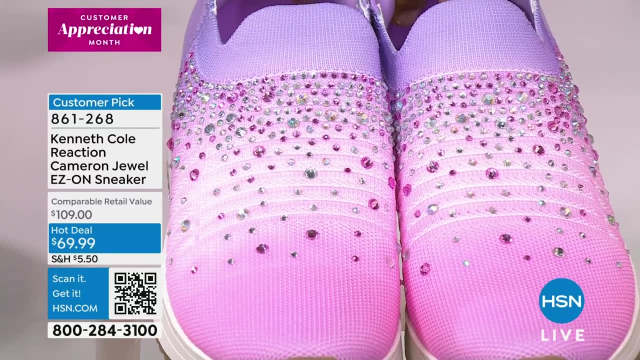 choice at the top is called unicorn. We're offering this sneaker and your choice of a medium width as well as a wide width, And we also offer you sizes five and a half through 12.. So this combination is unicorn. Down to my right, we have an old Navy. 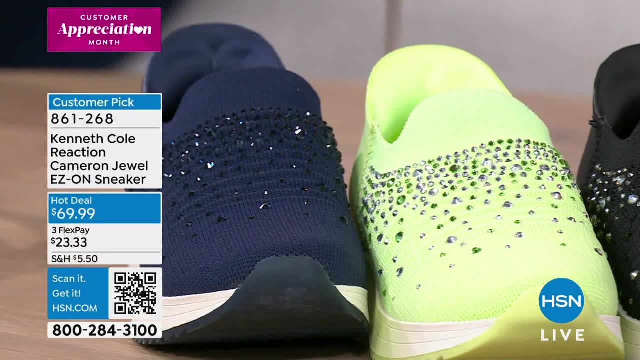 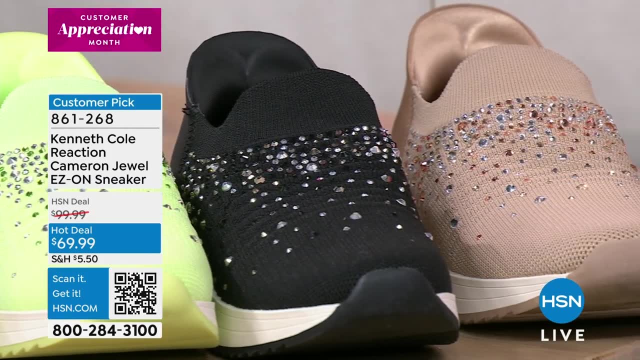 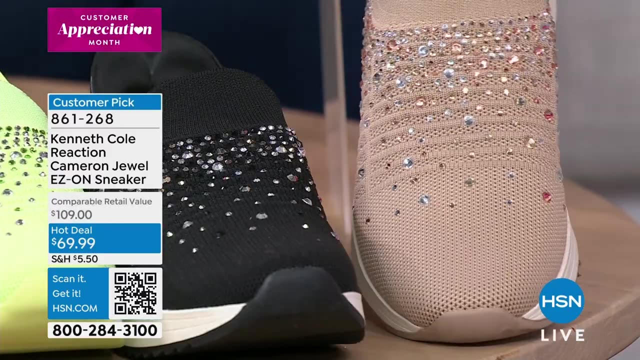 We have the black. I can't wait to show that to you up close. And then we also have the final choice, which is called Irish cream and the Irish cream. There are only 200 remaining in that choice, So the sizes are getting really, really limited. I'm going to hold them up and Casey dive in there. 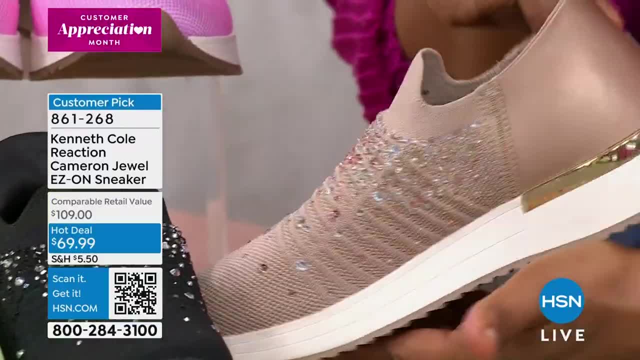 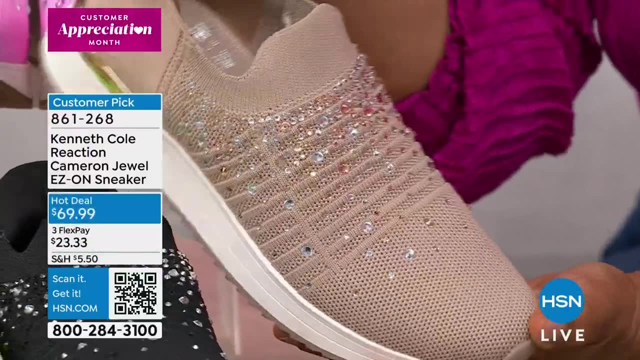 as I kind of. I kind of take everybody on just a little bit of a tour As you speak to the sneaker. I know it's been incredibly popular, but that's- I mean, that's- incorrect. That's really beautiful. 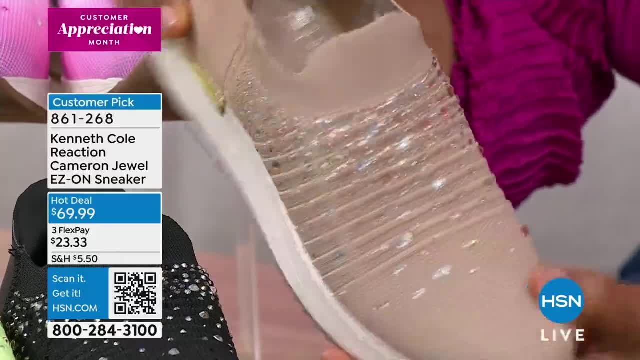 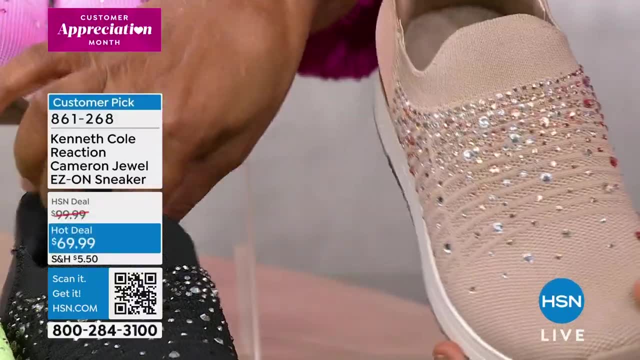 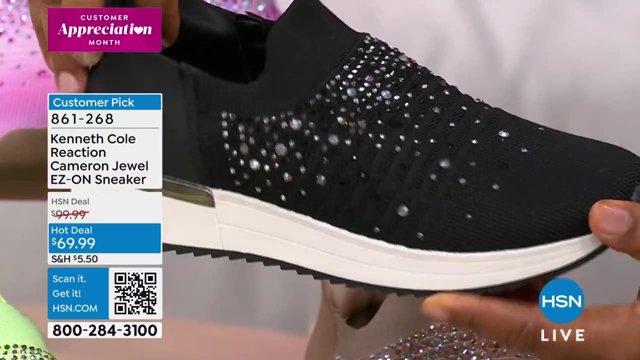 right, I'm not showing it styled with a dress, but it's going to look just as great with your, your denim jeans and your Capri shorts, your Capris, and you know all the things that you're going to be wearing during the summertime. Marlo, we launched this two weeks ago as a deal and it 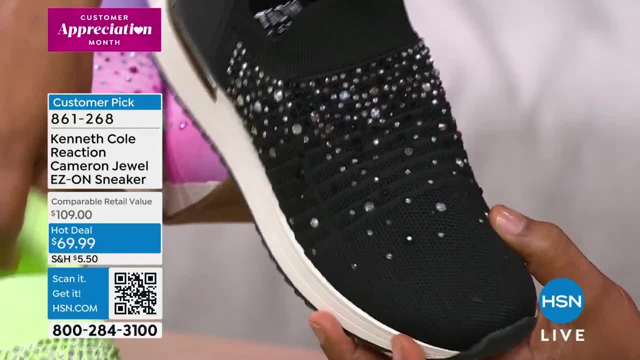 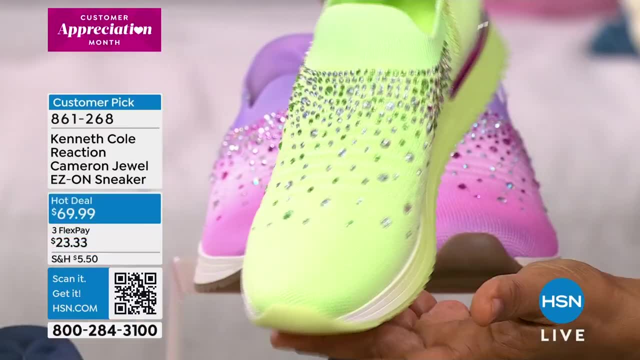 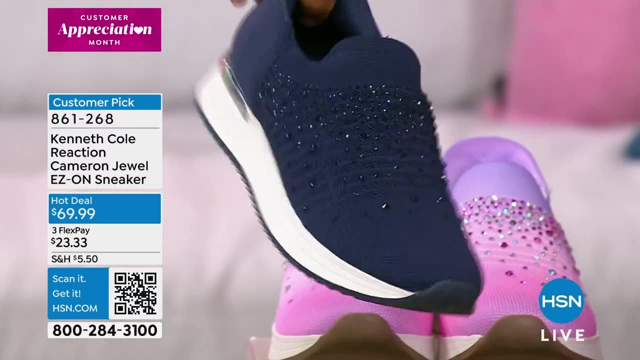 has already become a customer pick. It is a favorite. People are loving it. We cannot stop talking about it. It's such a fun shoe and it's a statement piece. That is the kind of shoe you're going to put on. You're going to walk into a room and people are going to go. where did you get that? 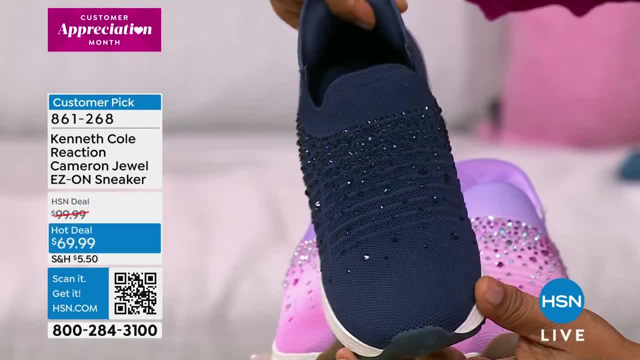 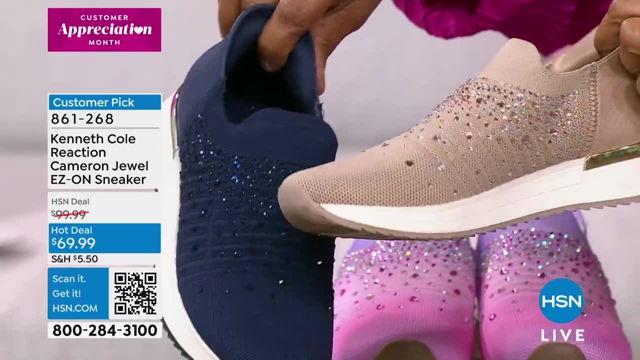 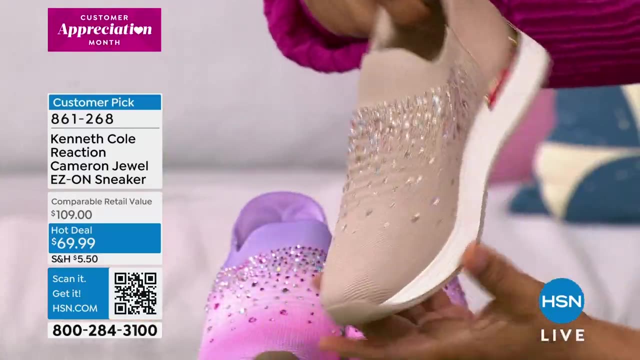 from And you know where. you tell them HSN because it's an exclusive. You're not getting these any place else. This Kenneth Cole reaction, Cameron easy on- is an HSN exclusive. It's such a fun shoe And, again, just like the harmony sandal, it's a blend of style and comfort. So Kenneth Cole was 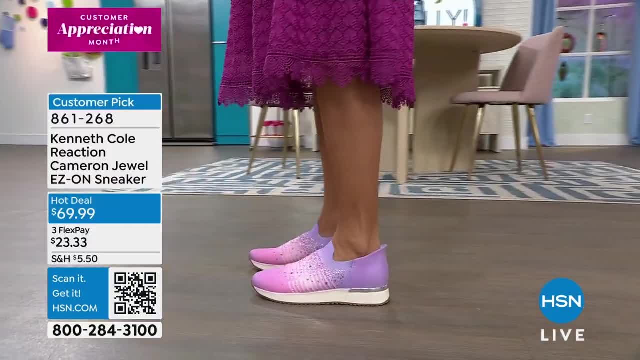 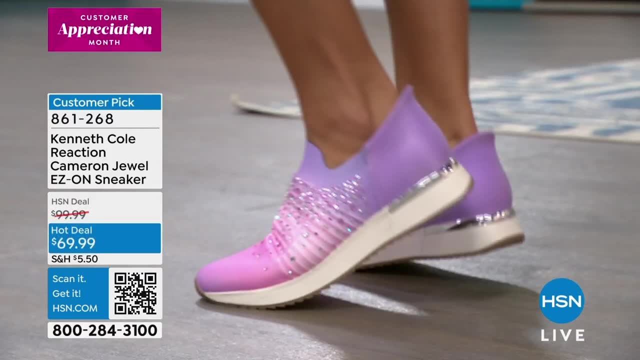 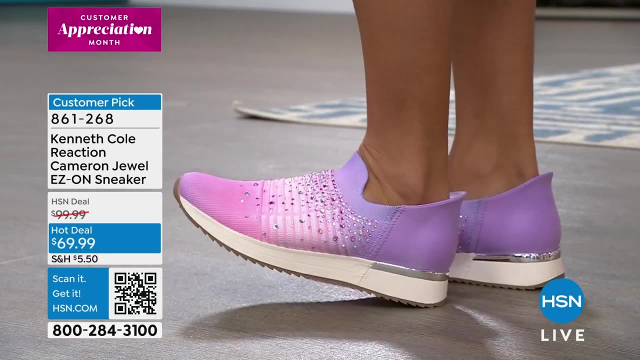 three years ago, Kenneth had three daughters who wanted style and comfort, and they couldn't find something that had a combination of both. So he said: let's start our own brand. And here we are, 40 years later: a global powerhouse and such great designs. Look at that metallic heel, Ram. 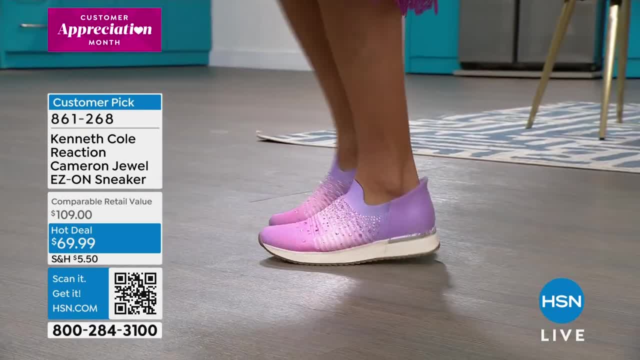 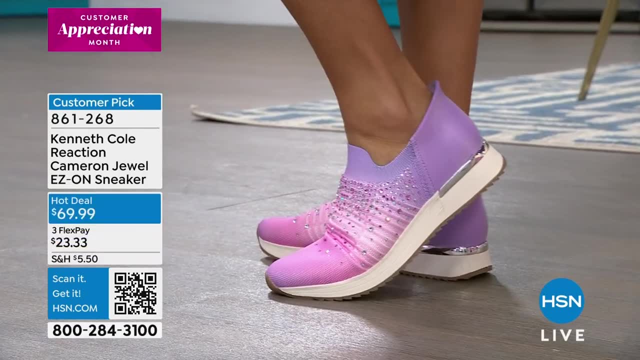 That's a Kenneth Cole signature. So we have this gorgeous little piece of detail. so subtle, but it really makes a big impact on the back of the shoe. No, I love it. I love that You don't have to have on socks or you just slip this on. Look. 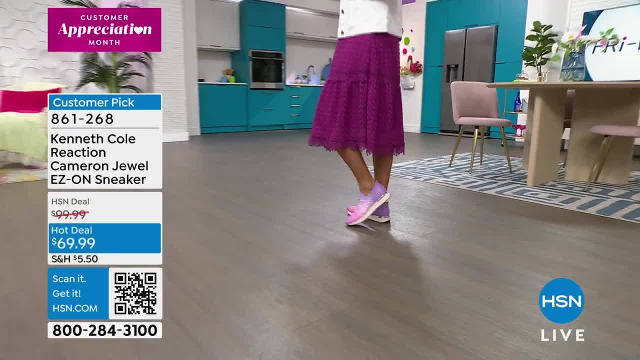 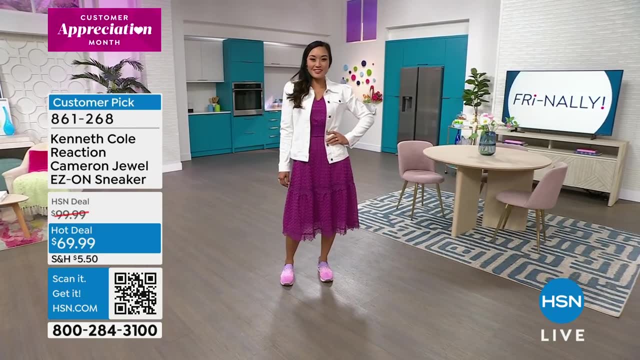 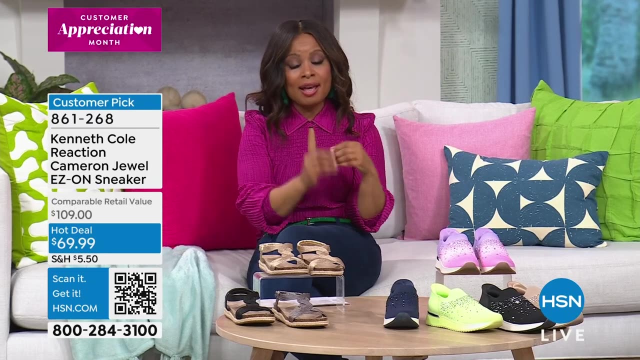 you don't even have to bend over. You can stand upright and just slip your feet right into. this style Sneaker is really, really popular. The difficulty, though, is finding one that looks as elevated as this one, So this one is definitely all about the Jews and all about the stones, And 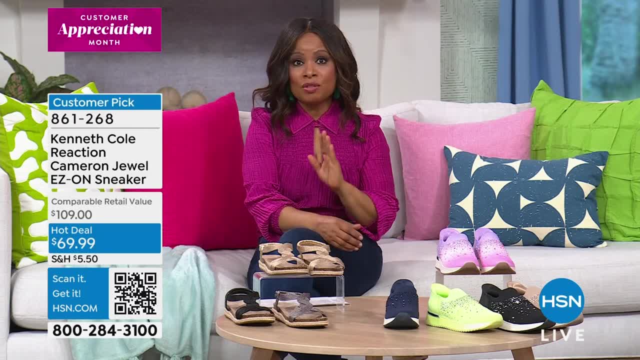 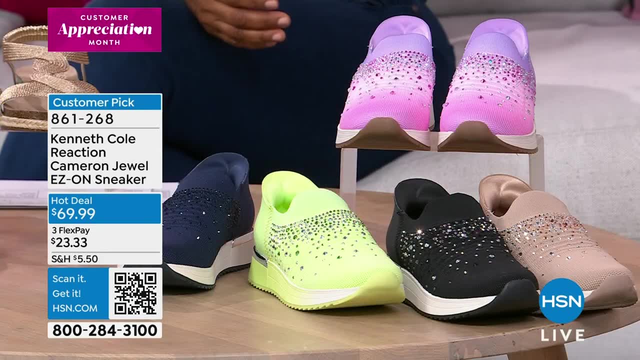 as we've mentioned, it's been very popular and you can choose the width that you need, which is rare in a sneaker, But we do offer this to you, and both medium as well as wide widths, And we don't often see that. 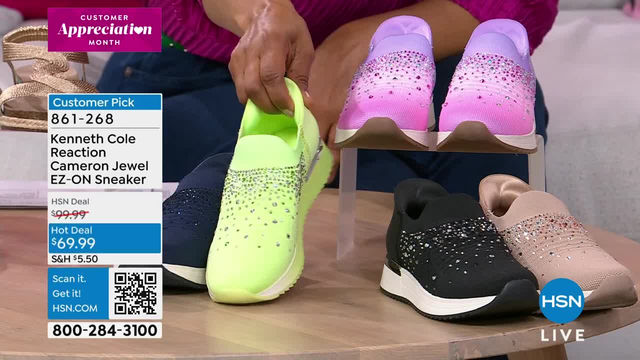 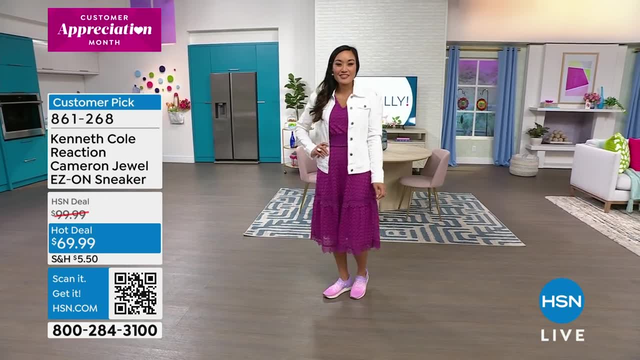 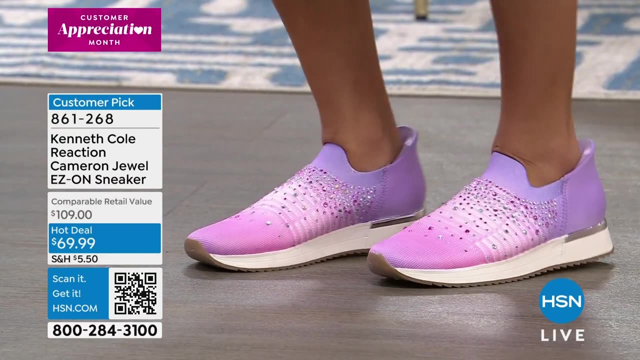 in the market. Casey, No, this is what's so exciting. True to size, We have the whole and half sizes. We have the medium and wide widths. That's such a great offering. You don't find that with a lot of sneakers and you definitely don't find that with a lot of the step in sneakers. 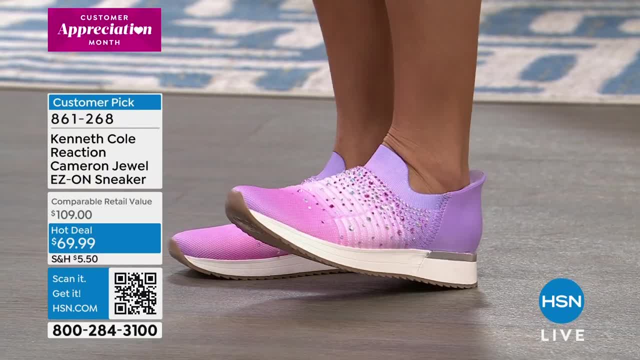 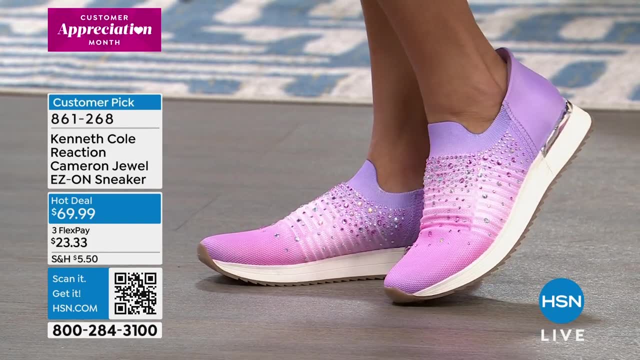 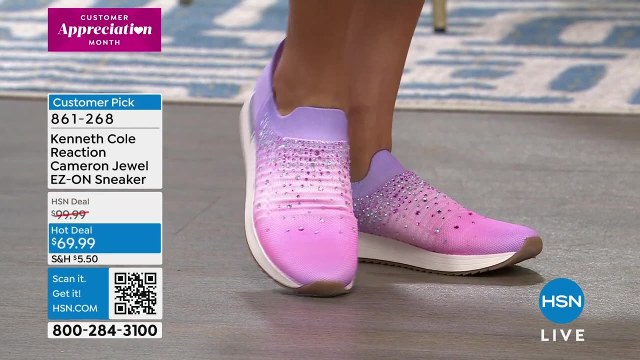 And that's why we put it in our name: Cameron, easy on it's right, You can slide into this shoe, You literally step into it. And that's because, as you'll see, on the back of her foot there's a built in shoe horn, So it's a really structured back to the shoe. 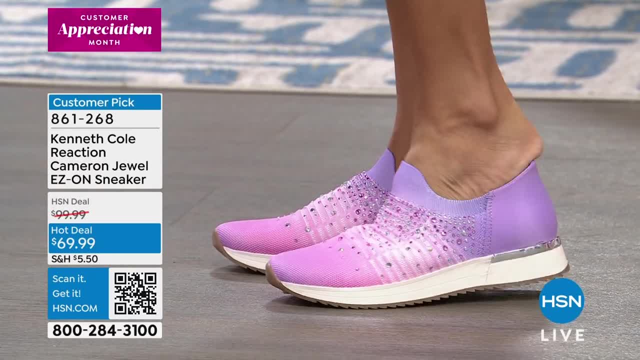 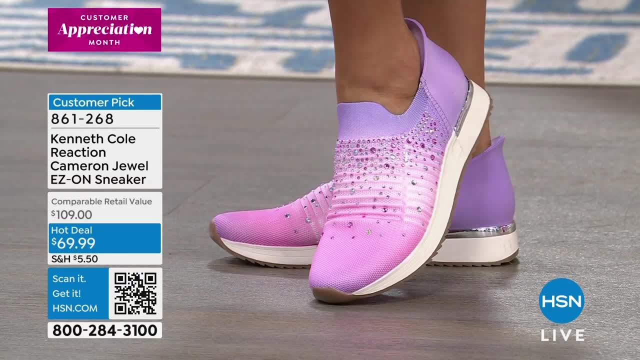 but you have this cushioning on the inside, probably an inch of of pillowy soft cushioning that makes it so comfortable And with that structured back you can step right into it. It's not going to break down over time. It's such a. 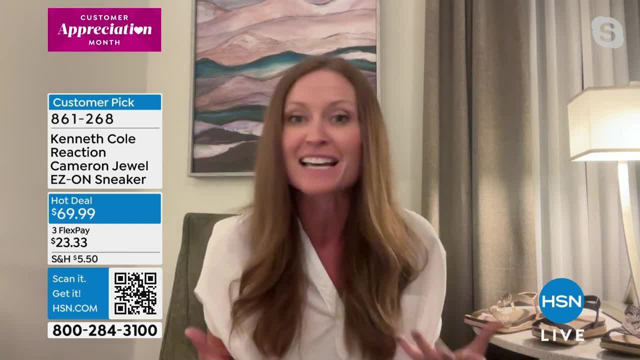 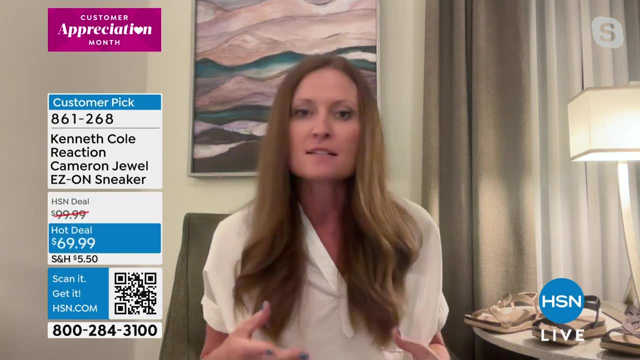 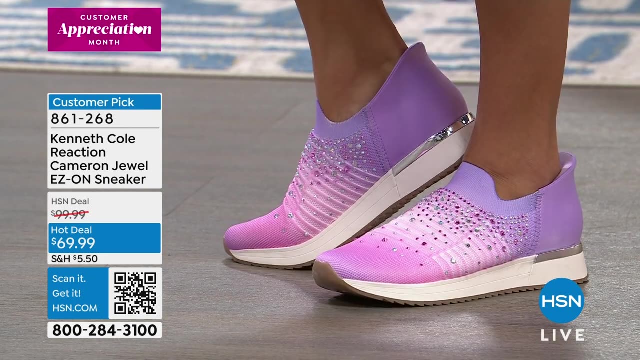 a beautiful sandal And, like you were saying, Marlo, it's elevated. That's what Kenneth Cole is known for: elevated fashion. So, yes, it's a sneaker, but it's a stylish sneaker. It's not something that's chunky or blocky or square, It's really designed to fit the contour of a foot.